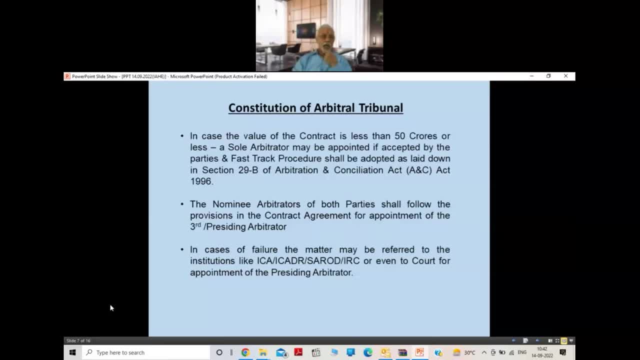 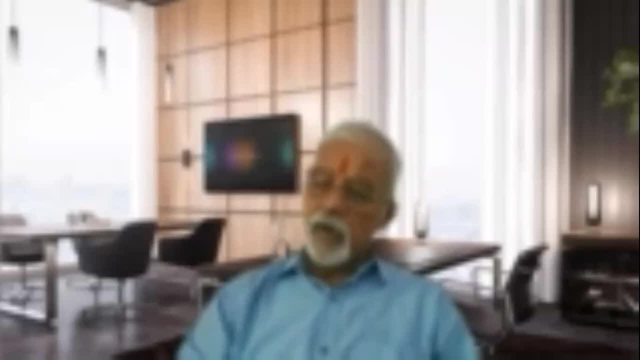 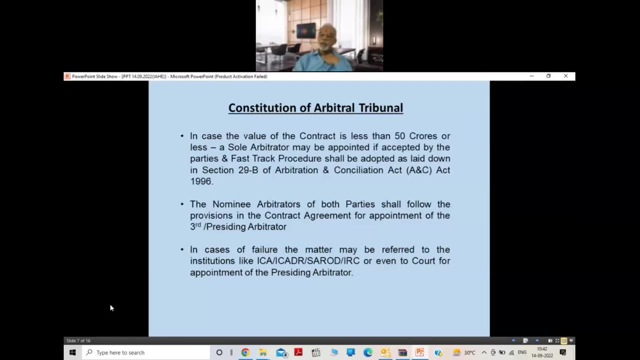 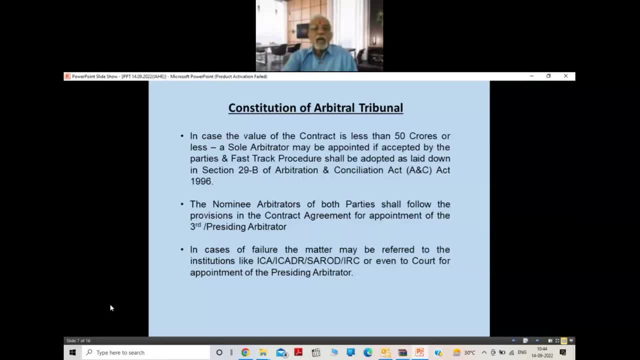 So all the participants know that we are conducting this program on 12th of September. So today is the third day of this on-going training program. We have already announced that the continuity and arm for highway project has been covered with relation to the manual of two-lane, four-lane and six-lane for the highways. 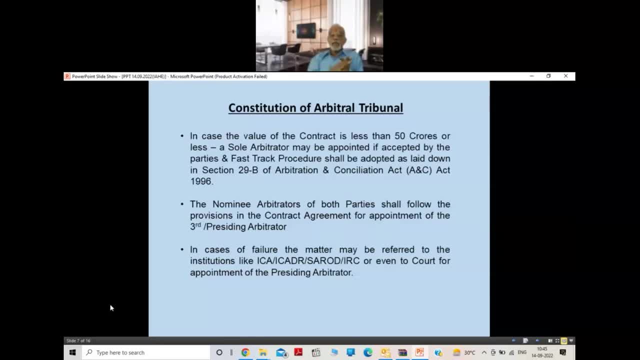 So today we will discuss on step-by-step procedure, So please make it a two-way communication. Please ask questions. I am not able to hear you, Sir. I can't hear you, Sir, I am not able to hear you. 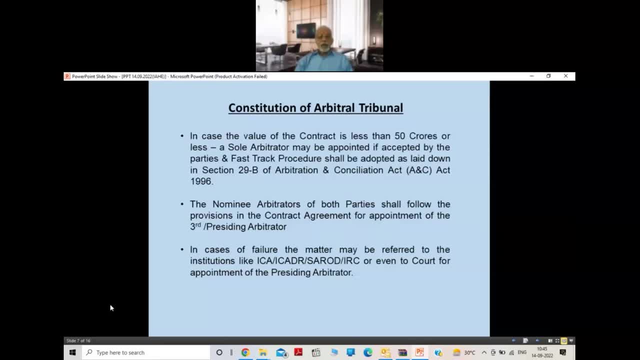 Sir, I can't hear you. Sir, I can't hear you. Okay, I could not hear you. I'm sorry I was not able to hurt Mr Gupta, but I think he might have Completed his Introductory. 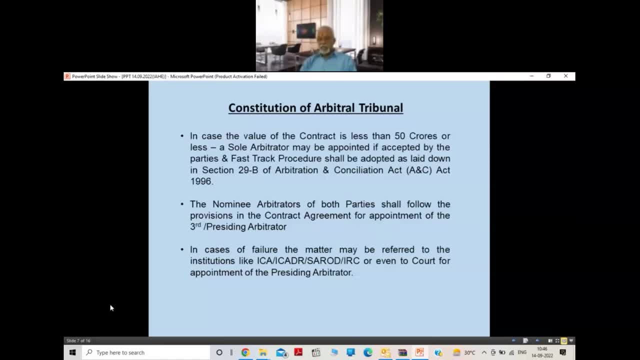 Now I'm I will introduce myself. I am Mokullu Parthak, Currently working in the Authority of India as advisor technical. Prior to this, I joined the NHI in 2001.. And in 2018, I retired. 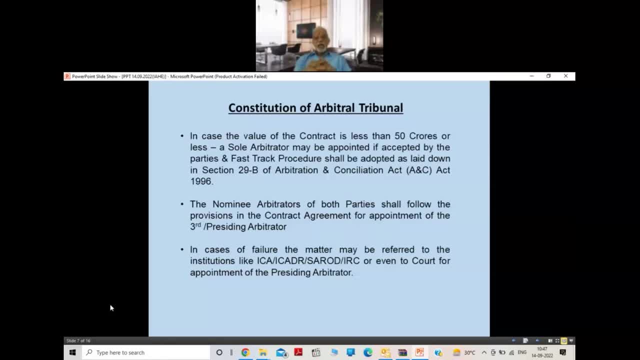 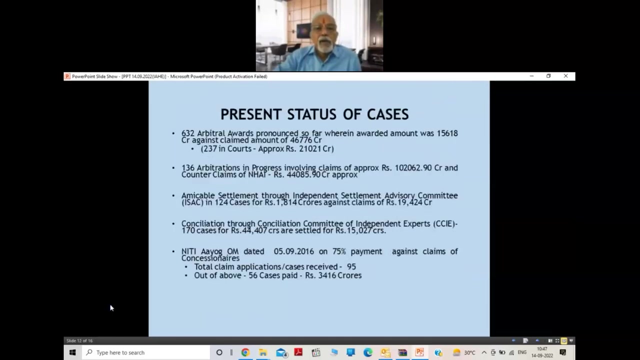 And from 2018 onwards I'm as an advisor technical in the NHI. From the beginning, I worked in legal and arbitration cell. Earlier it was known as dispute resolution and arbitration because actually my background is civil engineering, not a legal man. but 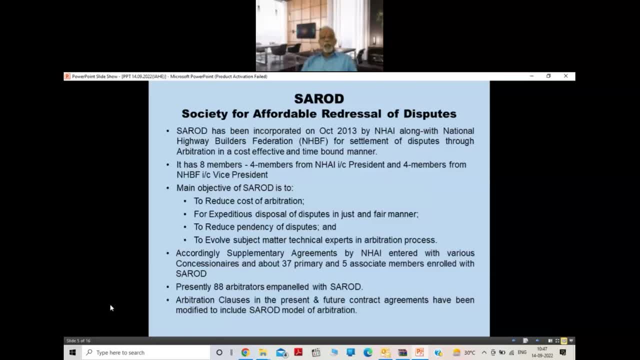 initially. at that time, the cell was looking after BRB and arbitration, So I was looking after that And I have handled almost 650 arbitration cases. This is an award that has already been published. Now, as today's lecture is on step-by-step procedure, 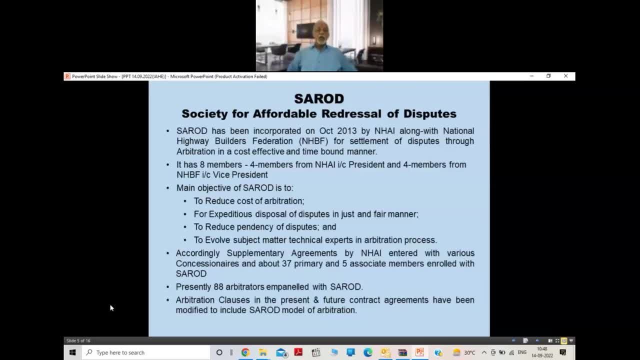 of to handle dispute from conciliation to court. Let me let you know that we're gonna get into the main topic of the webinar. If you have any questions regarding the court case, please do not hesitate to reach out to me. I'll be there. 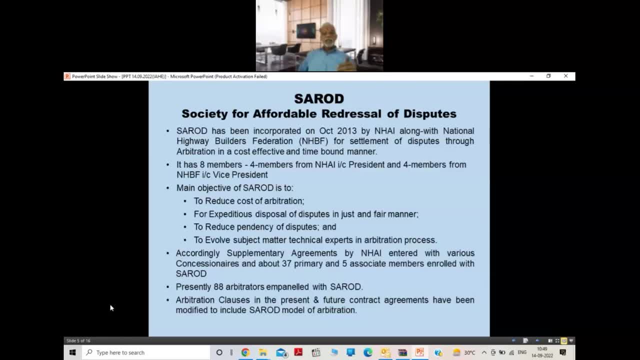 Thank you. We will be back with another webinar, So we will continue the discussion as usual. I'll be back in a few minutes. If you have any other questions, just let me know. I will have the time. I'll see you later. 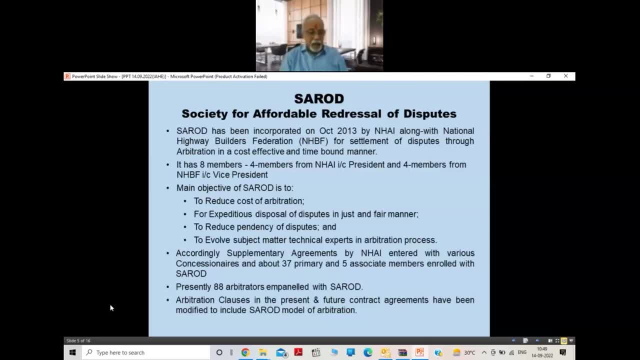 Thank you, Take care. Thank you very much. I'll see you later. Bye, Bye, bye, Bye, bye, Bye, bye, See you, Bye, bye, Bye, bye, Bye, bye. See the dispute resolution mechanism provided in the item road rate contracts. 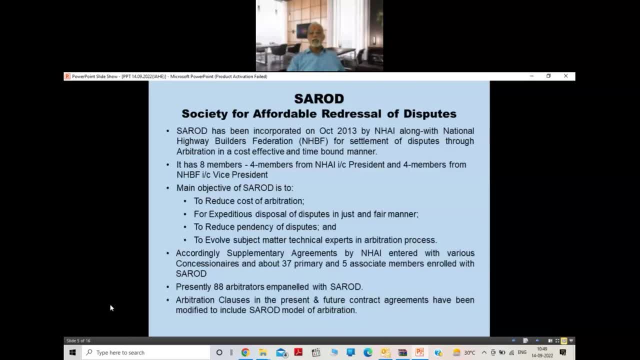 The procedure there is the, if any dispute arises during tenancy of the contract, then the supervision consultant or the engineer he supposed to mediate between the parties and to try to resolve that issues initially. but in case that dispute is not resolved by the mediation, then 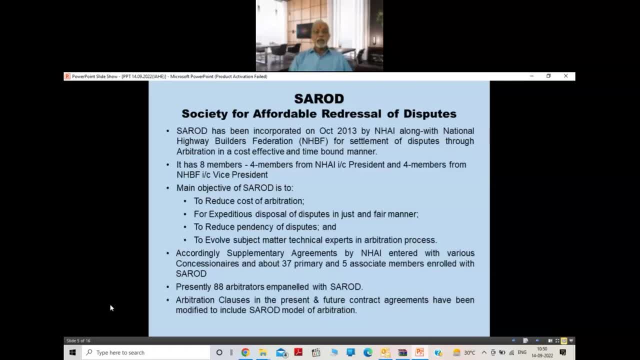 the provision is provision of the contract is that the that rejection of the from the engineer, the dispute can be referred to dispute review board or dispute resolution board within 14 days of the decision of the supervision consultant. this is what has been provided in the contract. now, once the dispute is referred to drb. 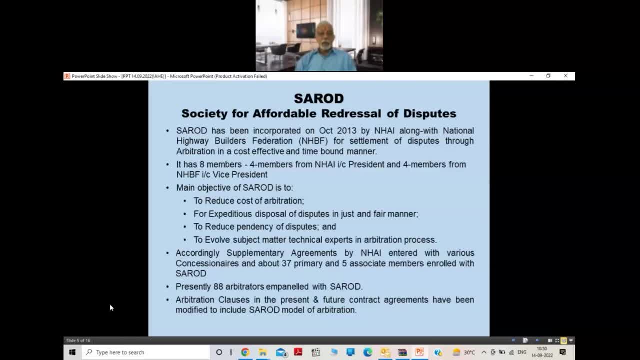 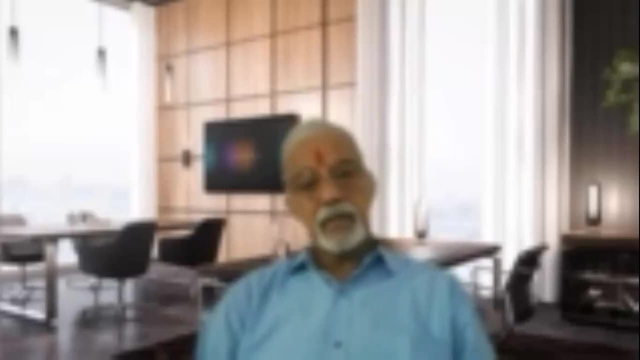 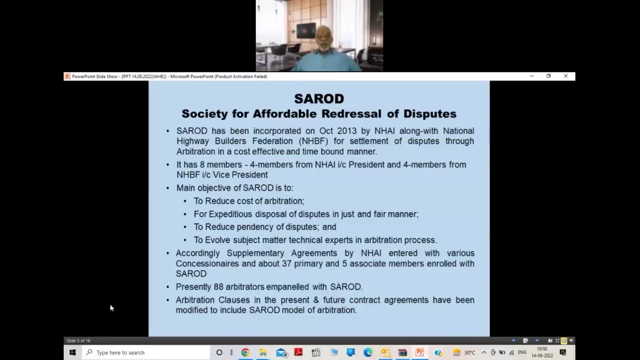 then drb, as per contract, is supposed to issue their recommendation within 56 days. now this 56 days starts from the day when the pleadings or the documents- written documents like statement of claim or this statement of defense, etc. they are submitted from from the last date. 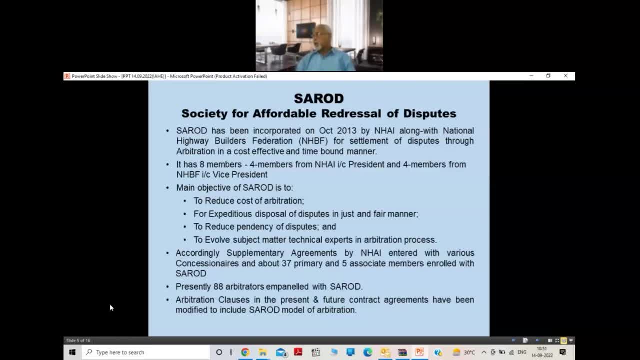 when the resender is submitted date starts, this 56 days starts from that day and in case if brb feels, or the party feels, that the 56 days are not sufficient for a particular issue to resolve or issues to resolve, then with mutual consent that 56 days can be further extended. 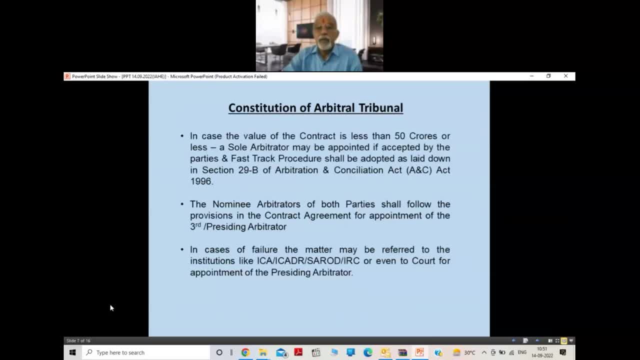 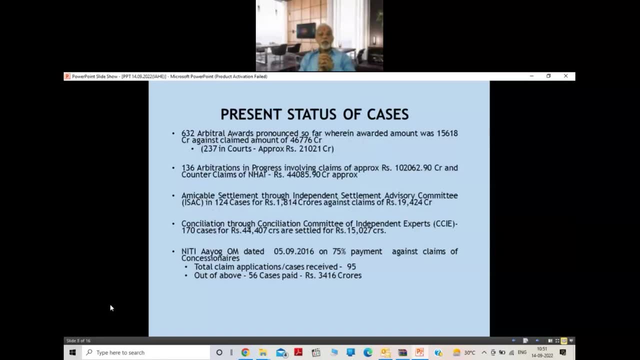 with mutual consent of all the three Parties, like the employer, the director and the DRB members. Now if any party is aggrieved by the recommendation of DRB, then that can be referred for next step in the contract as the arbitration directly. 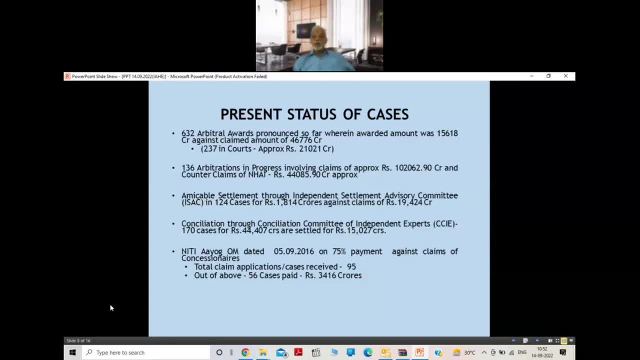 Now another step has been introduced in between DRB and the arbitration, That is, conciliation In NHI. sometime in 2010,, a procedure for conciliation was started That was called IEG Independent Expert Group. This group was created by 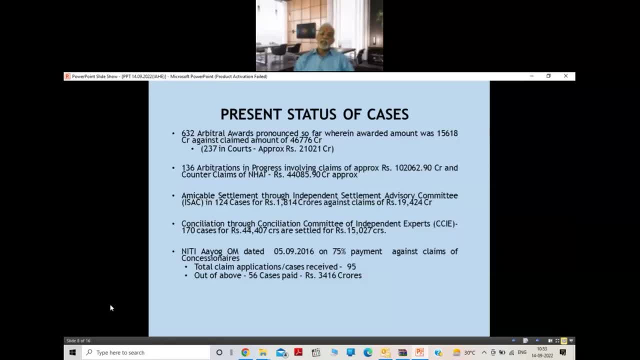 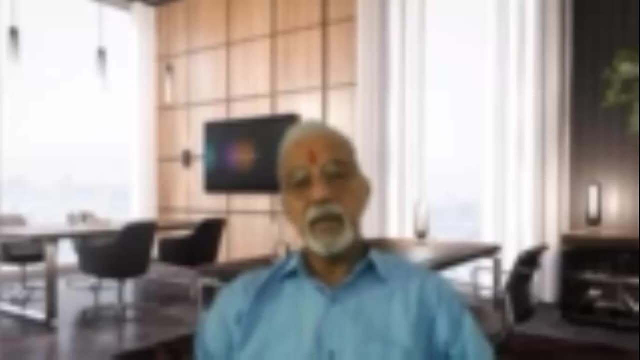 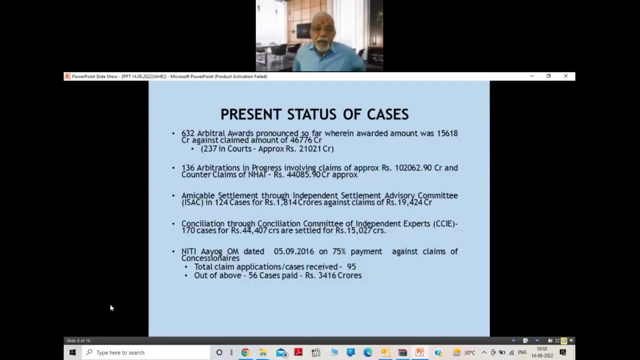 GDN Planning Commission, where four members, retired senior officials, were there, added by a retired Chief Justice of High Court, one DG MRTH, one Deputy CAG and one CBC. This group was supposed to give their suggestion, or you can say, recommendation. 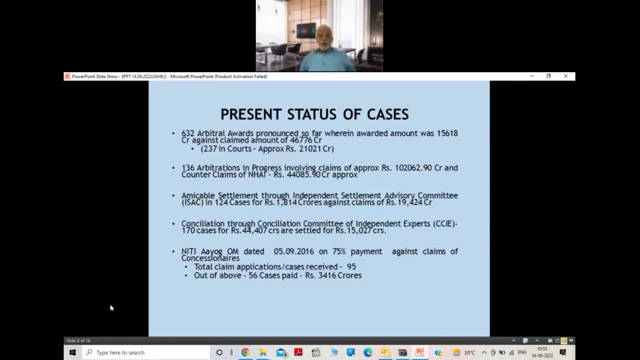 to both the parties, after hearing or looking after all the documents, whether this case is good to consider. So it was decided that either it is to be conciliated or it is to be challenged in the court or to arbitration. Since their scope of work was very limited, 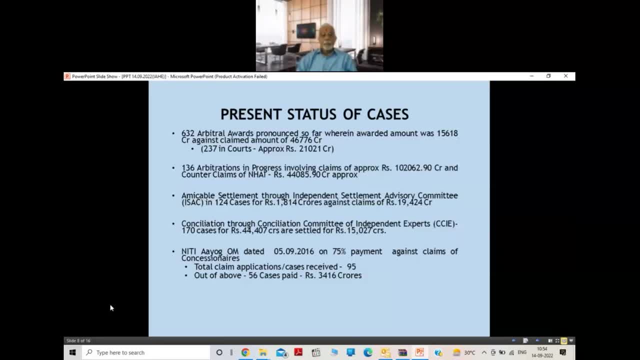 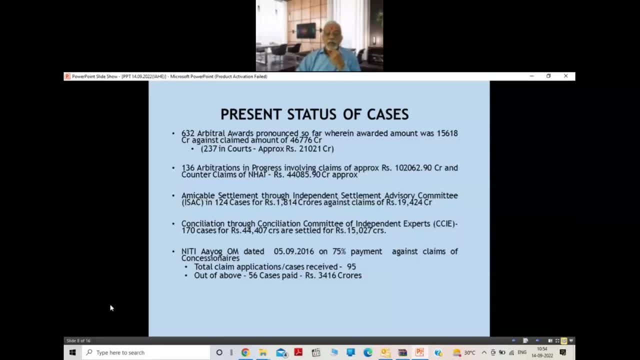 Independent Settlement Advisory Committee. That committee was comprising of three members added by a retired judge, one technical member, DG Ministry of Road Transport- and one bureaucrat, senior level bureaucrat of secretary rank. all retired are made a committee by. 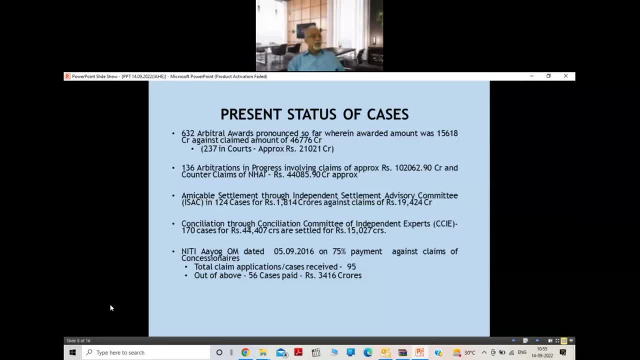 NHAI and the process of this conciliation was: once the party- any party, either NHAI or the contractor- needs to refer their issues before going to arbitration, Or before going to DRB or court, or either pending NHAI or DRB, or arbitration or court. 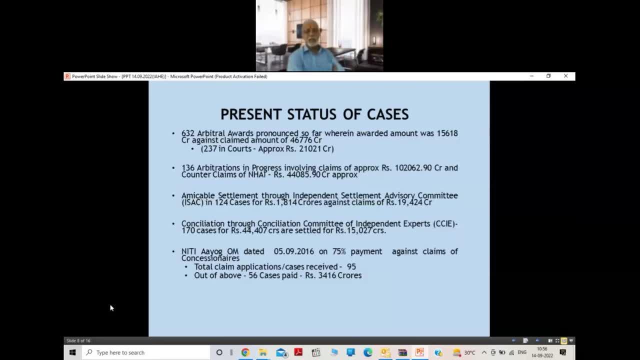 Any point in time any party can refer issues to this committee by requesting NHAI or writing a letter to NHAI. So the process of this conciliation was once the party- any party, either NHAI or DRB, or arbitration or court or any party, can refer issues to this committee before going. 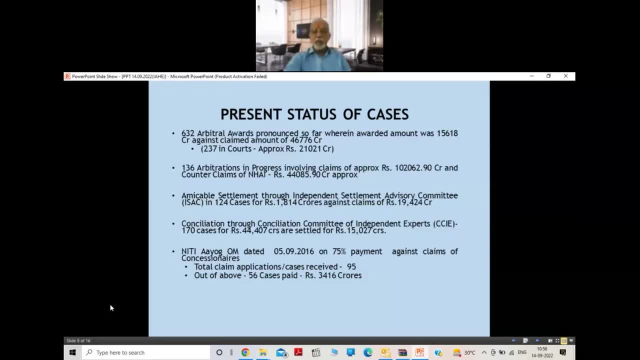 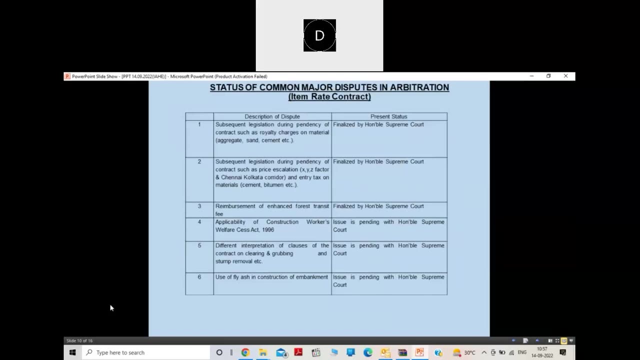 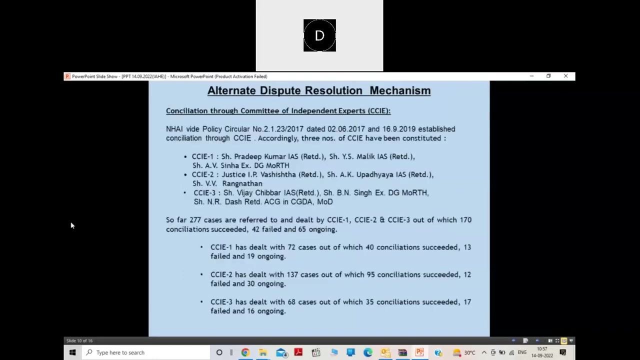 to arbitration Any point in time, any decisions, We will do it. We will be there in the morning and evening. Hello, Continue, sir. So any party can refer at any point in time and there is for settlement, advisory committee. 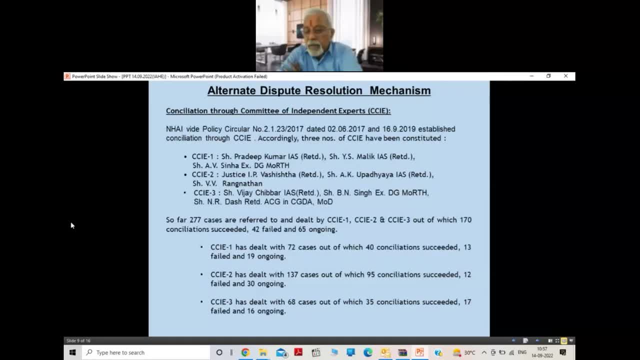 And the process of was that, as soon as And the chair receives any request from the director that they want to go for conciliation, And three different subcommittees comprising of CGM technical and CGM finance level officials, And we used to refer. 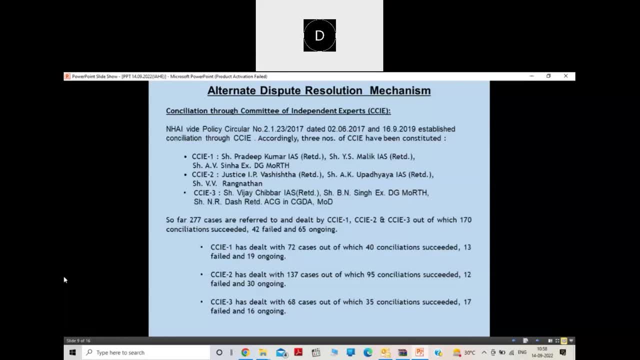 Their issues to one of the committee And that committee Discusses the issues with the contractor And the concern NHI technical division or the PIU and PD And Try to come to an Conclusion That Where both parties agrees. 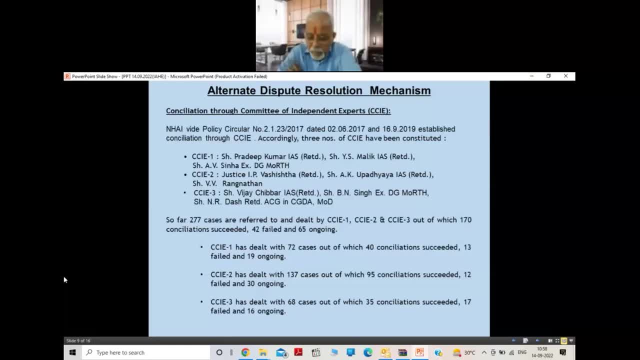 To do or to come out for an agreement at Some point in time. If any agreement has reached, Then they will make up Their report Along with complete detail of what what the contractors issues are and what they have Submitted What. 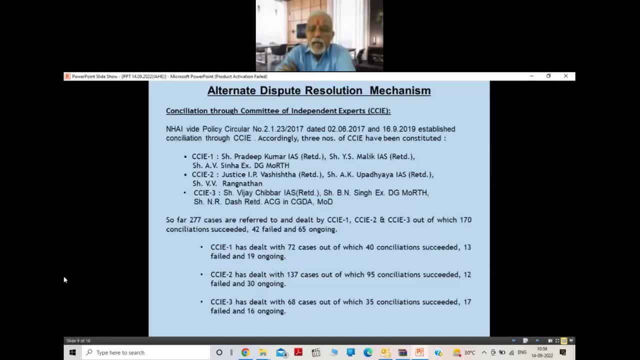 What sort of Documents In Support of Their Claim And Then Similarly NHI's Commands and their Supporting Documents And That Report They submitted to the Isaac, The Independent settlement advisory committee. 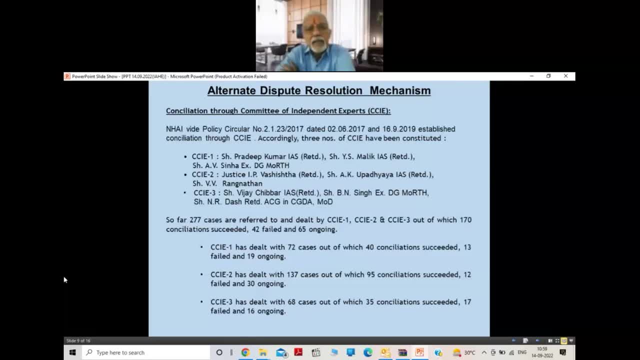 So That Committee Comprising Of Three Members- I Code Judge D, G, M, R, D, H And One Senior Secretary Level Official- They Go Through. 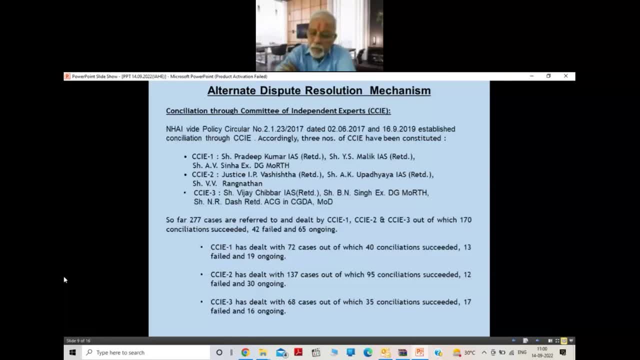 With The Report And If There Is Any Information, Either From The Rector Or From The Committee, They Call And Discusses With Them. And Finally, 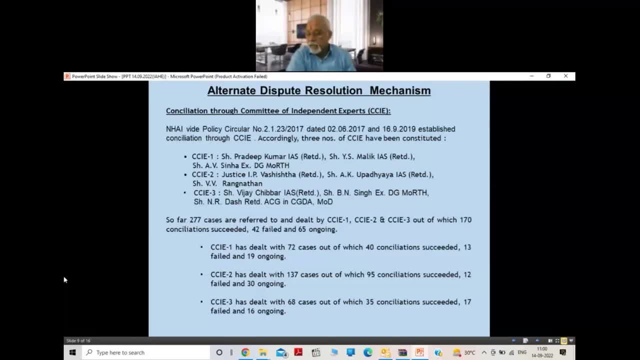 Forward Their Comments On The Reports Of The Subcommittee To Sign As Agreement: Settlement Agreement Where In Everything Used To Be There And The The Amount. 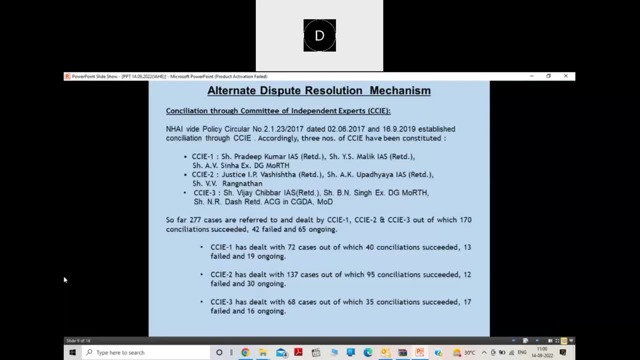 Which Has Been Decided By Both An H. I Would Like To Let You In Say Two Or Two And A Half Year From 2012.. 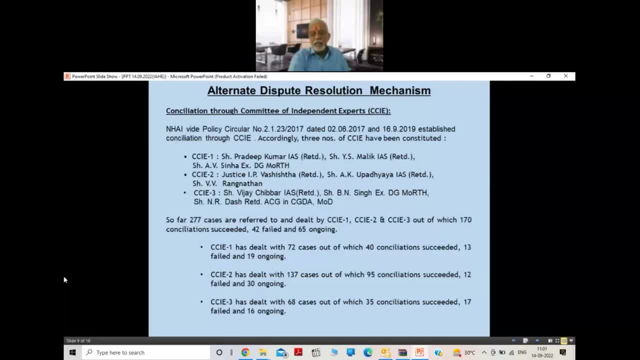 To 2013.. We Have Settled Around 125. Cases Appending At Various Levels In The World, And You Will Be Surprised To Note. That The Clean Amount On This 125. Cases Were 19. 400. Crores, The Huge 19. 100. Worth Of Has Been Settled In. 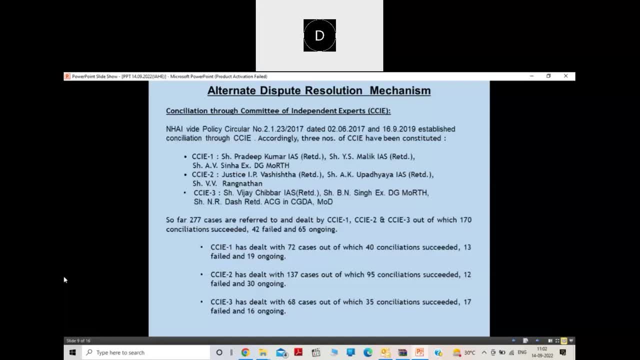 The World From 2012. To 2013.. We Have Settled Around 125. Cases In The World, In The World, And We Have Settled 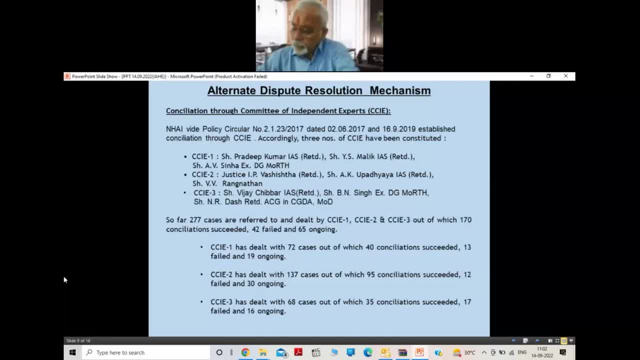 Around In The World, In The World And 2015.. We Have A Red, A New Con Correction Process, Which Will I Come Back To You. 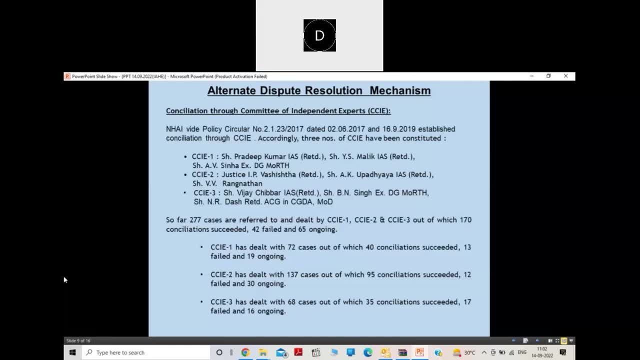 After Some Time, That So, After Recommendation Of Dr B which are not settled during the cancellation process, and it will be challenged in arbitration. That too within 28 days of submission of DRB recommendation. otherwise it used to be a. 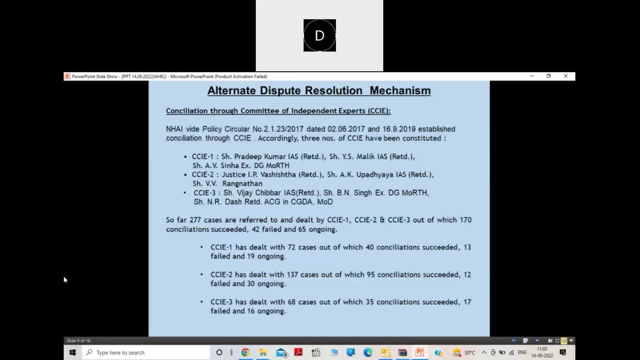 time bar, And if the award, the arbitral award, earlier this Arbitration and Cancellation Act was revised or amended in 2015,. prior to that, there was no time limit for publication of award, So it used to linger on for years and years. 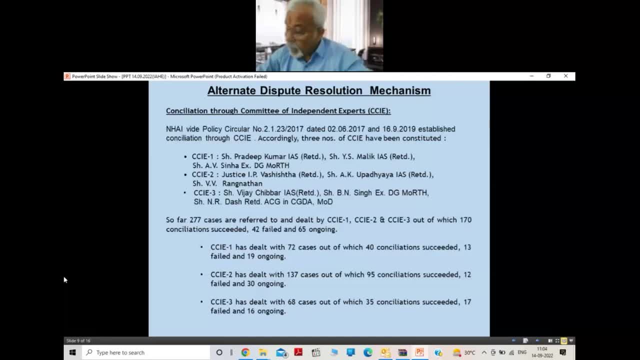 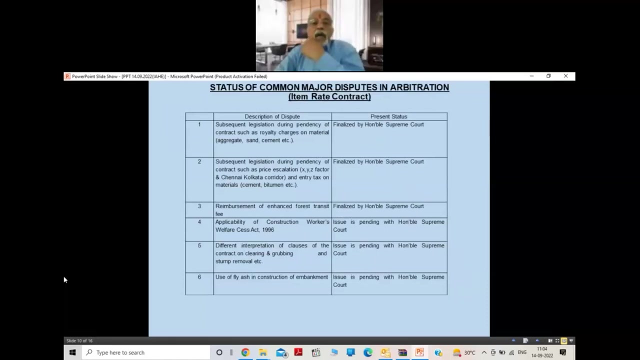 But after 2015,. that time limit has been described or provided for publication of award. Very nice step was taken. I was talking about the item rate contract provision, Now the provision in BOT, EPC hand contracts- Almost similar sort of mechanism, but the first mediation by independent engineer is. 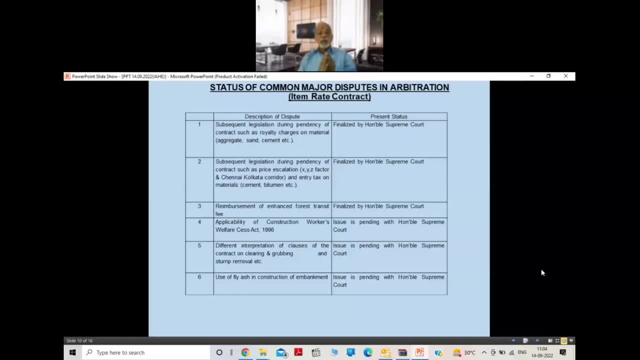 the same as it was in the item rate contract. The initial provision, or earlier provision, was after failure of mediation through the independent engineer. Correct, Sorry. The provision was that the conciliation for a makeable settlement was to be initiated by the parties. 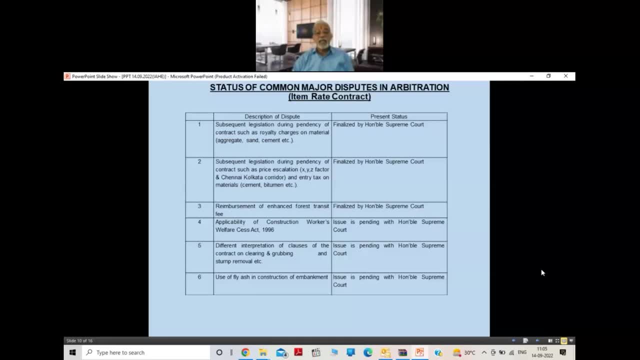 And this conciliation is carried out between chairman and the chairman of the department And the time limit was very short. They will have to call the parties for conciliation within seven days from receipt of the request by the parties and submit their report in 30 days. 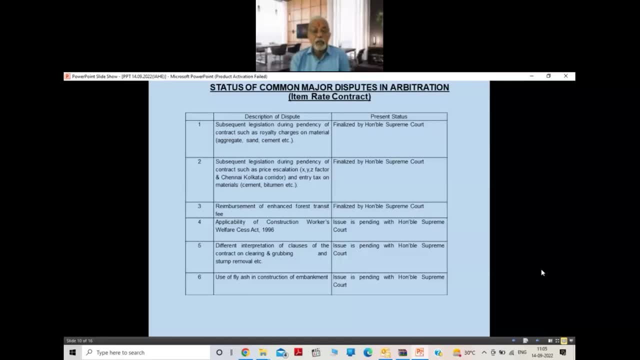 So it was found that the time limit was very short. Okay, So it was found that the time limit is very, time period is very short, as well as the availability of chairman NHI and the chairman of concession within seven days. Sometime it's very difficult. 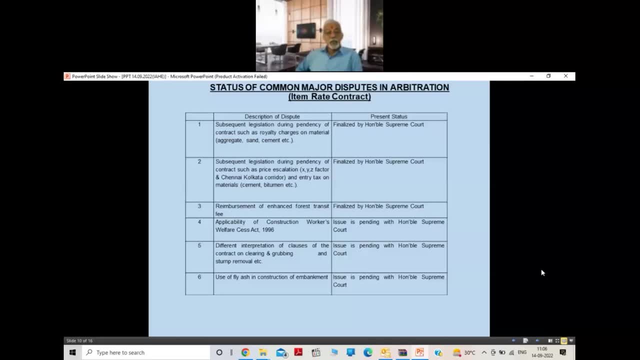 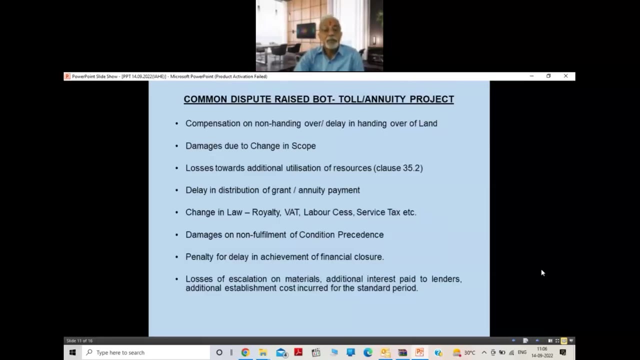 So it was decided subsequently that the conciliation process should be carried out by the department. Okay, So the process should be revised or reviewed. Then it was reviewed and a new mechanism was introduced, That is, the conciliation by a committee of independent expert. 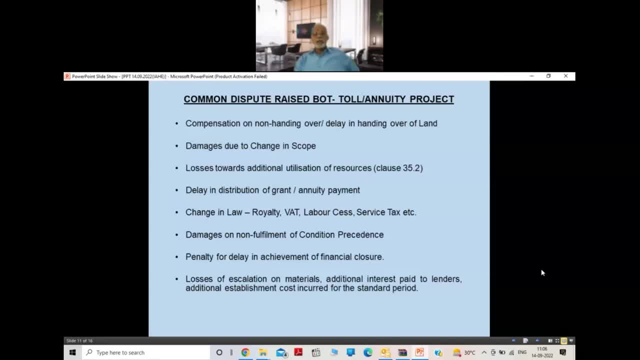 So NHI has, Okay, Constituted three such committees presently. So presently they are in function. I'll come later about the further details. Then the provision is in case. if The provision is in case, if the conciliation is failed, this provision, what I'm talking, 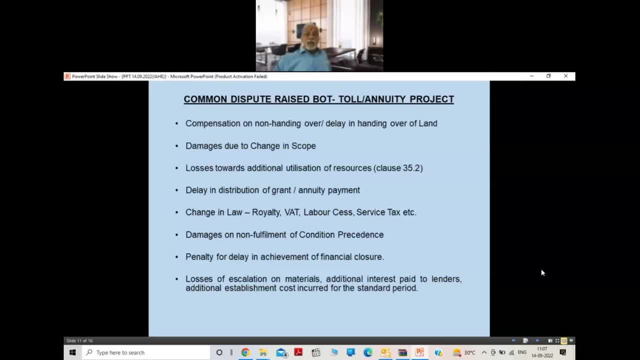 about are the earlier provision of the contract agreement which was subsequently revised. After conciliation, the matter will be referred to arbitration. Then, after arbitration, the court Now here in BOT or EPC or contract also. as soon as the mediation is failed, then next. 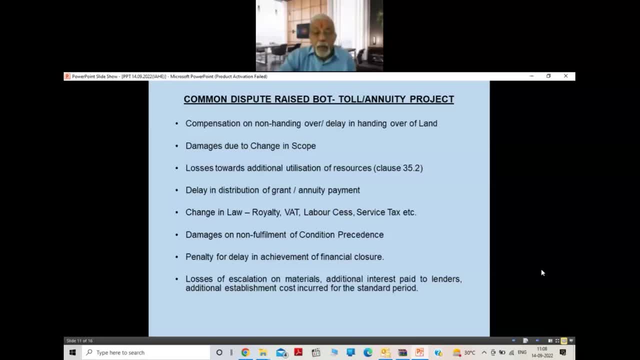 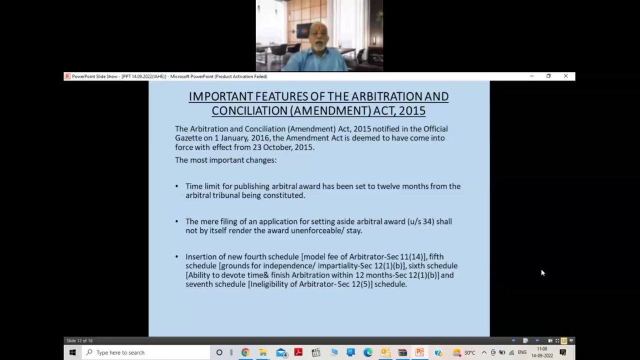 step is refer matter to DRP. Then after Any parties agreed by a recommendation of DRP, then that can be put for conciliation and then arbitration. then court is. This is what the additional provision of in contract for all BOT and EPC contract. 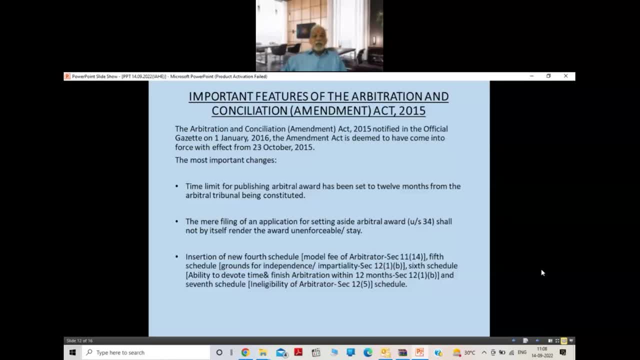 Okay, After failure of the conciliation by independent expert, the matter is referred to DRP And from DR after DRP, it is referred to conciliation by the conciliation committee of independent expert. Then, Appealing conciliation, the matter shall be referred to arbitration. 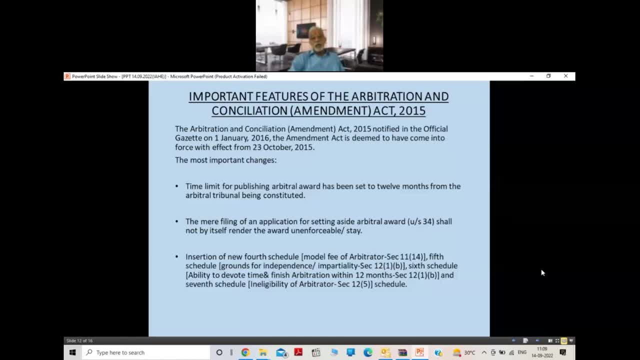 And this is what the staff chief and all other departments shall be referred to as independent expert. This is what the process of litigation we have discussed: Unresolved claims at field level, conciliation by two chairman- This was earlier provision- Arbitration, district court, High Court, Supreme Court. 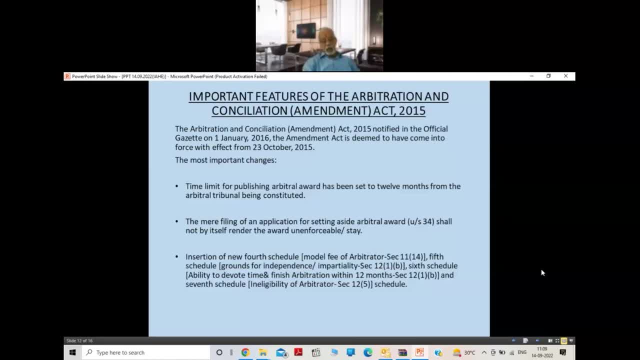 And then this conciliation by CCIE. CCIE can now be called CIE EARLIER. CCIEE can be approached at any level, by anybody. This is the provision of the Constitution of Arbitrary Tribunal. Let me come to CCIEE. 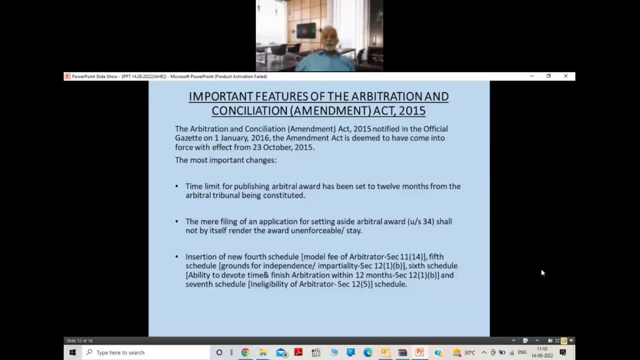 The Concentration Committee of Independent Experts. presently we are having three committees, As you can see on the screen that this CCIEE was initiated or created, or legal for the CCIEE. CCIEE was initiated or created, or legal for the CCIEE. 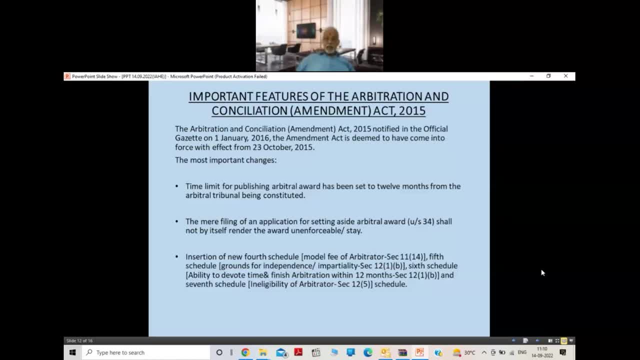 From 2017 onwards, and initially there were only one committee, then subsequently it was increased to two and finally it is presently three committees are there. The first committee is comprising of Mr Pivit Kumar, Mr Y S Malik and Mr H V Sena. 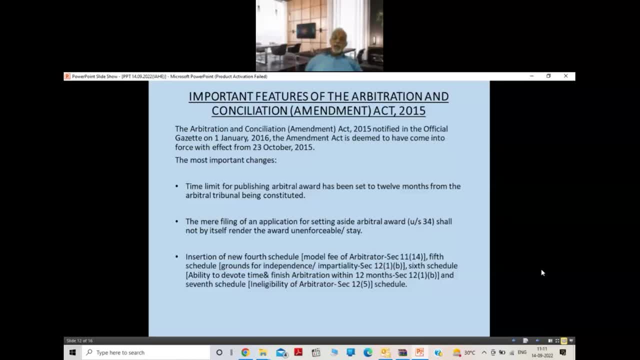 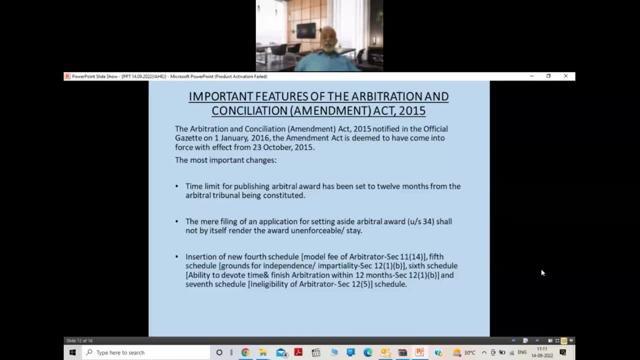 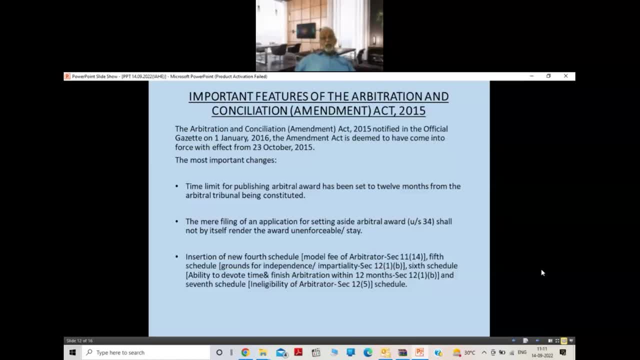 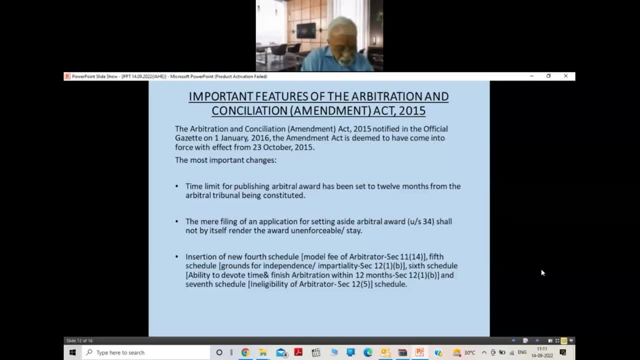 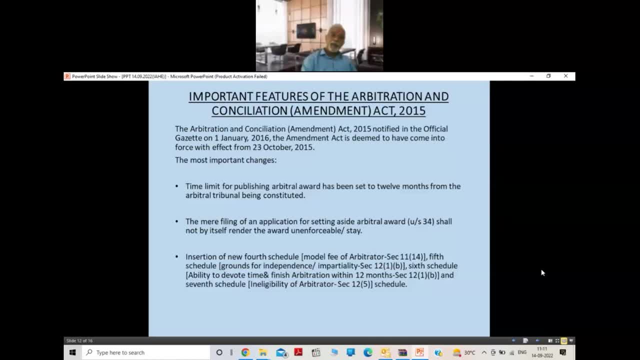 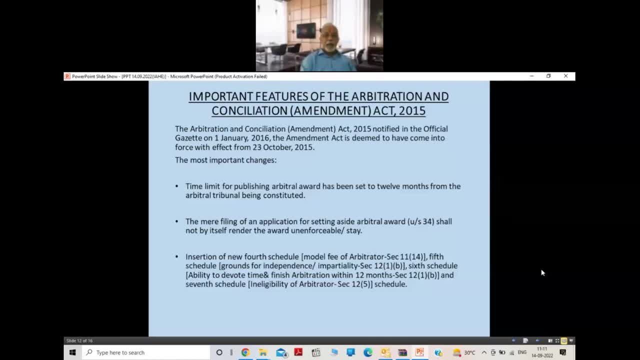 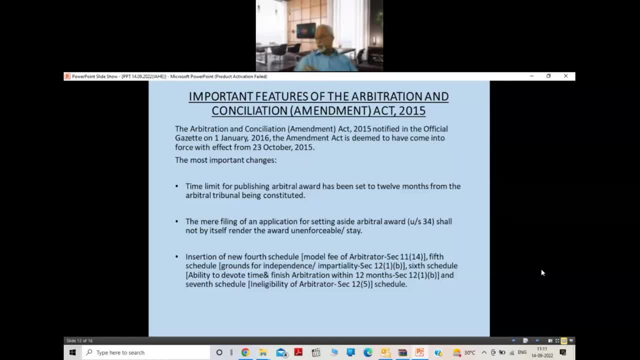 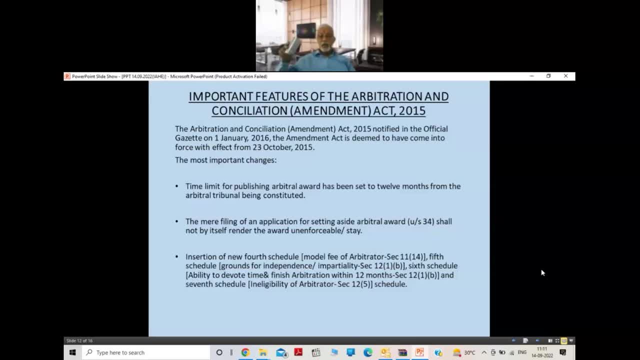 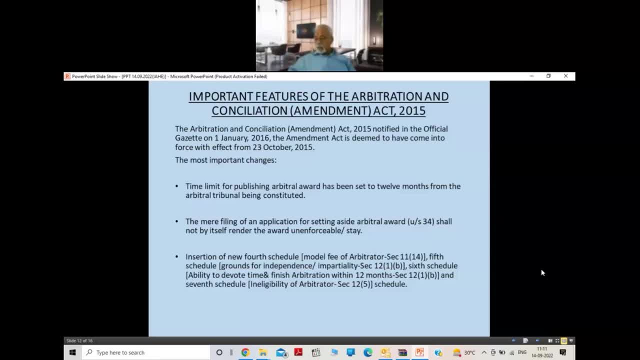 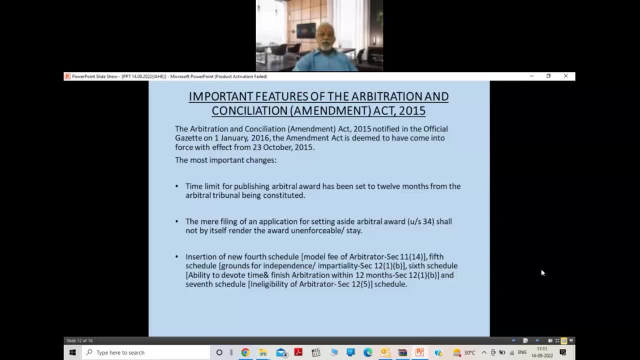 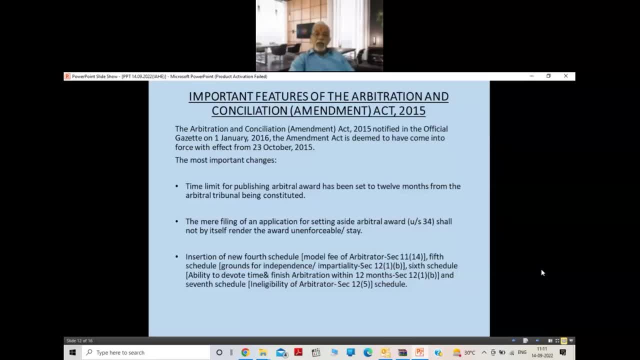 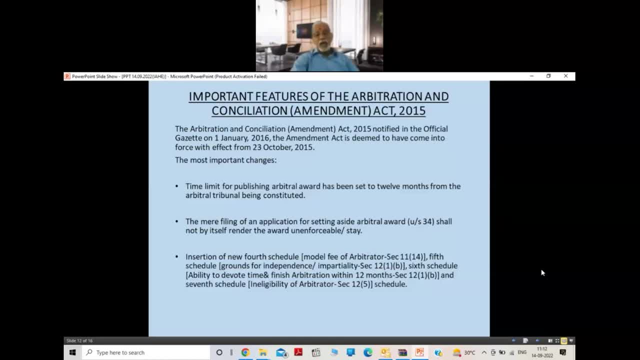 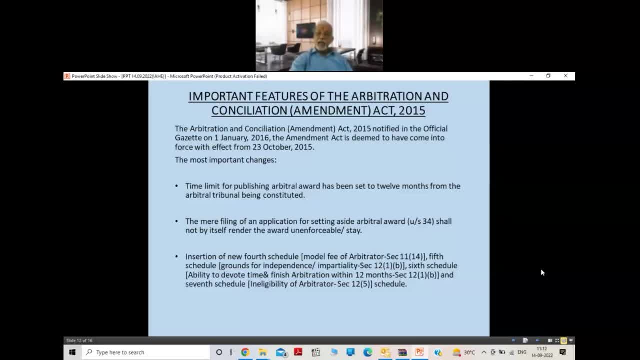 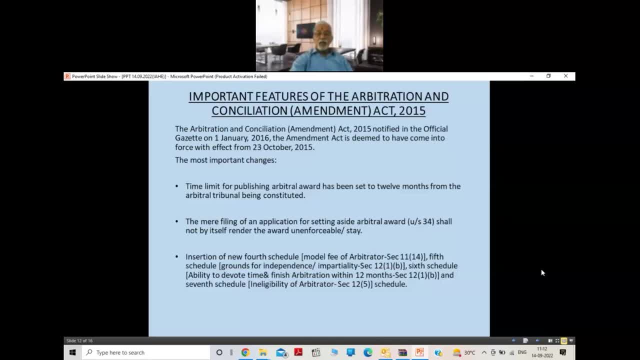 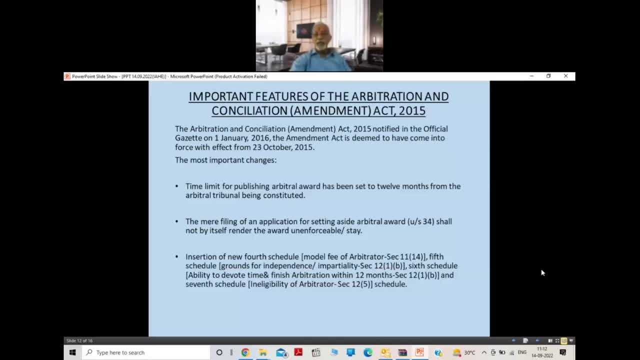 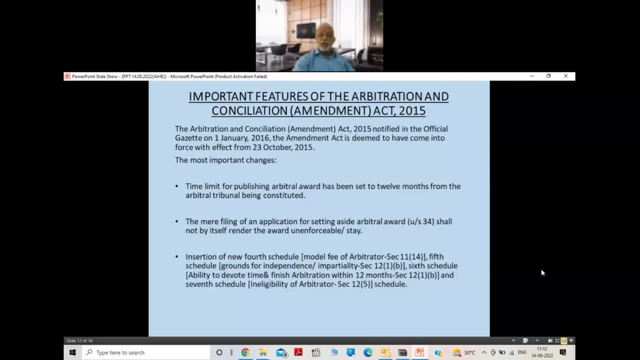 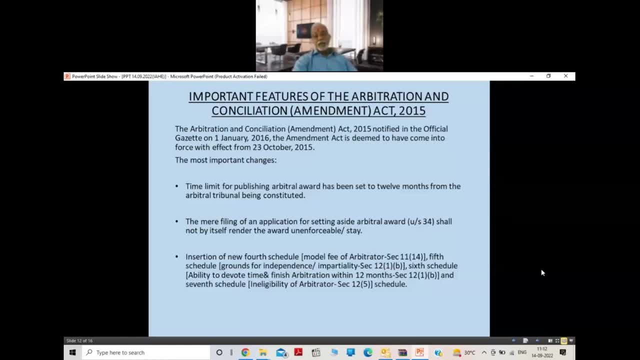 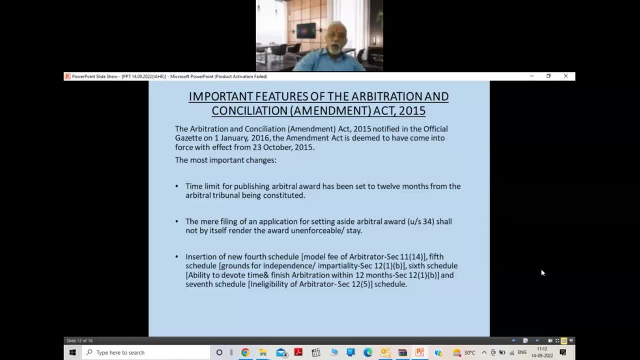 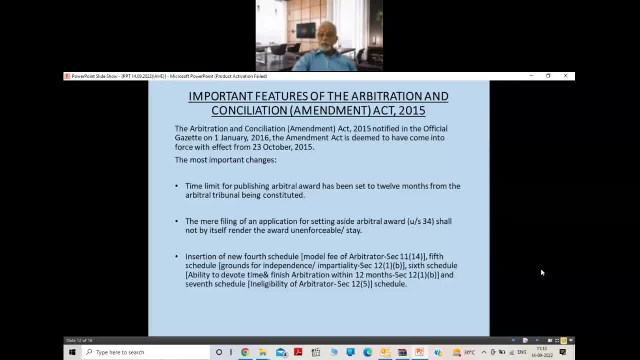 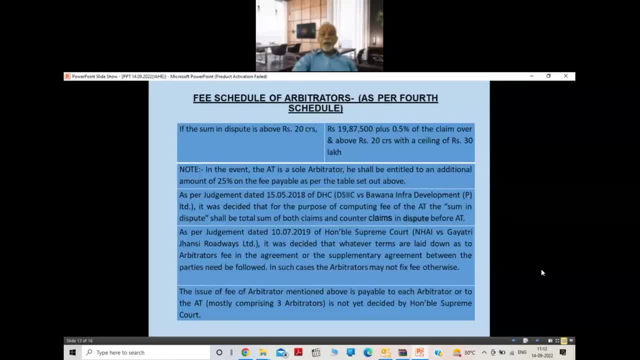 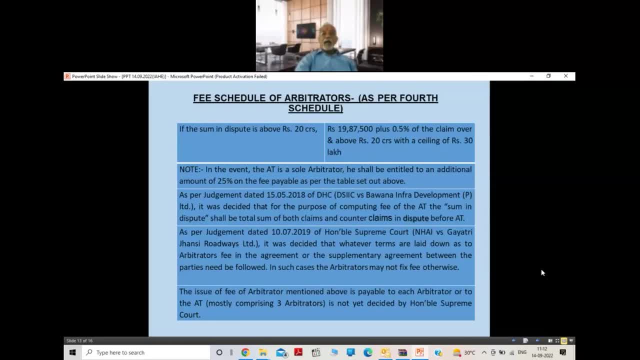 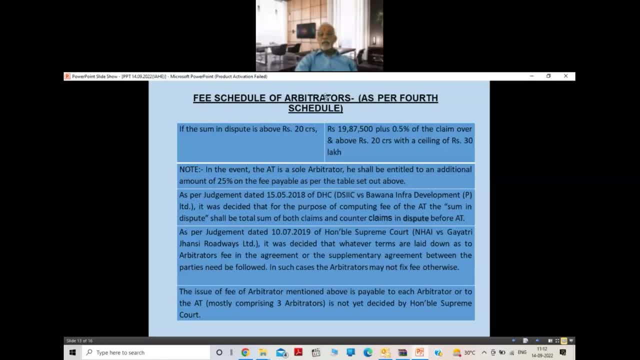 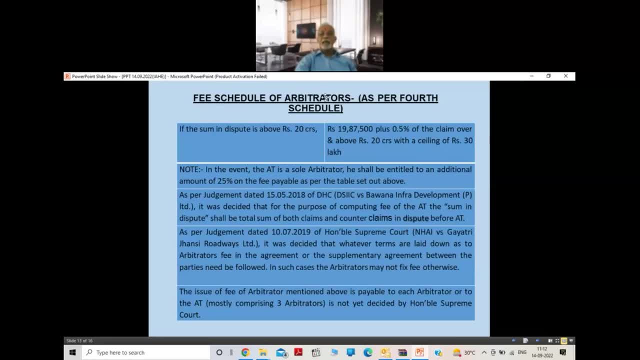 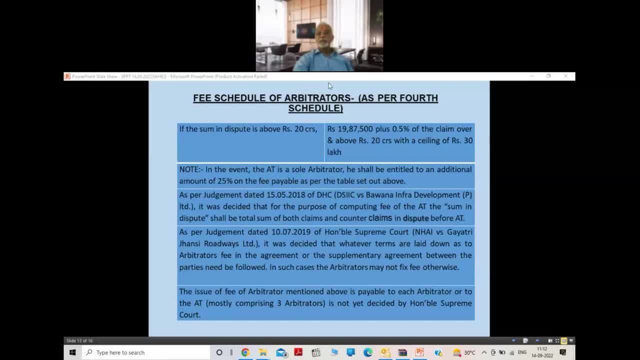 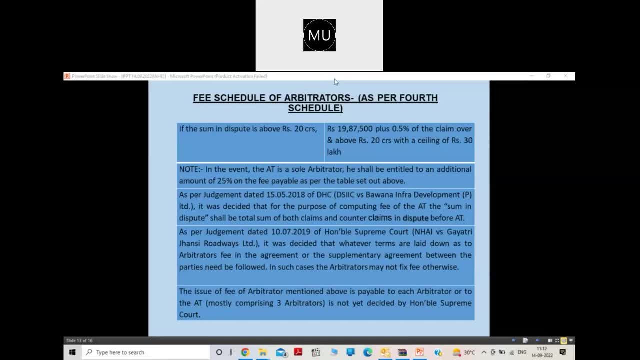 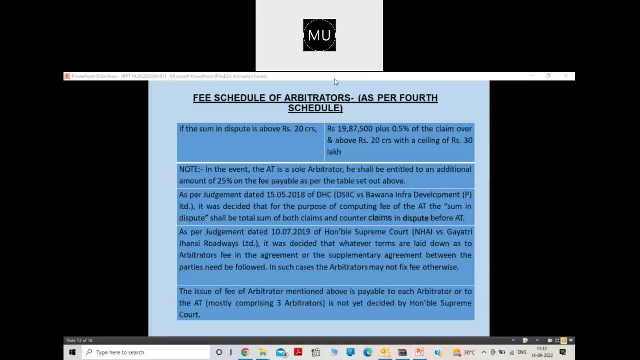 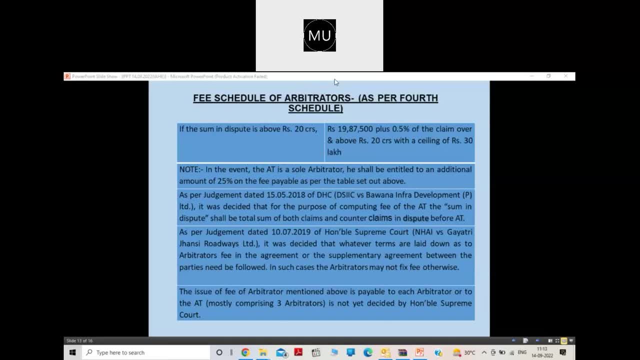 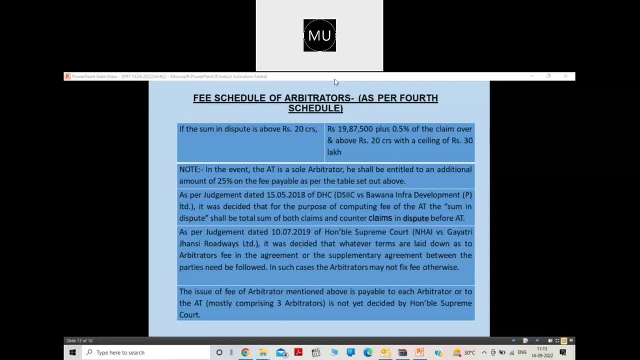 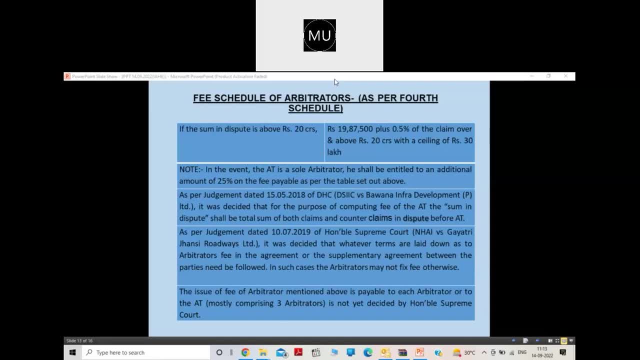 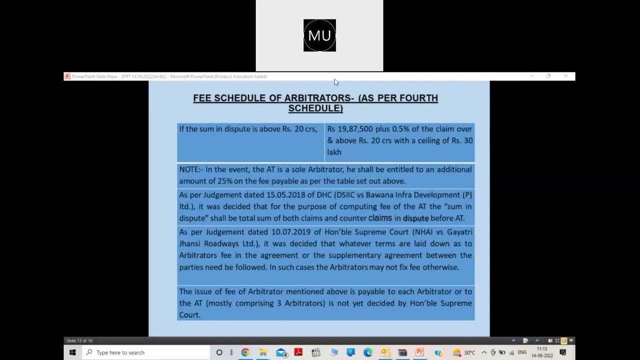 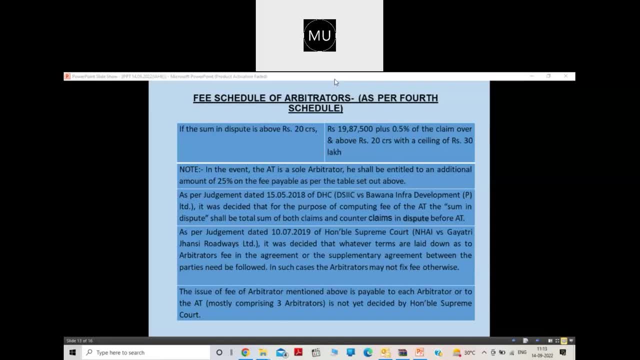 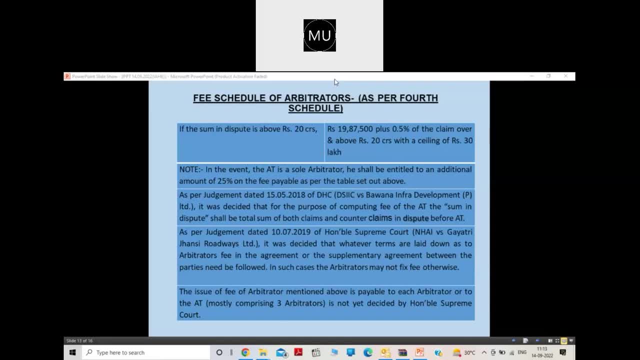 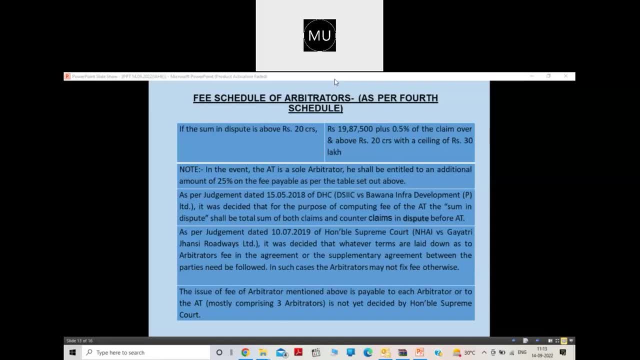 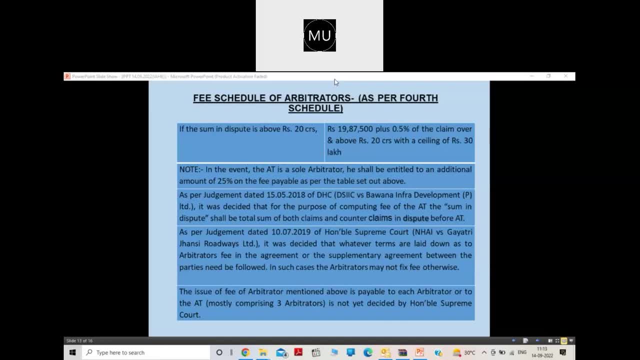 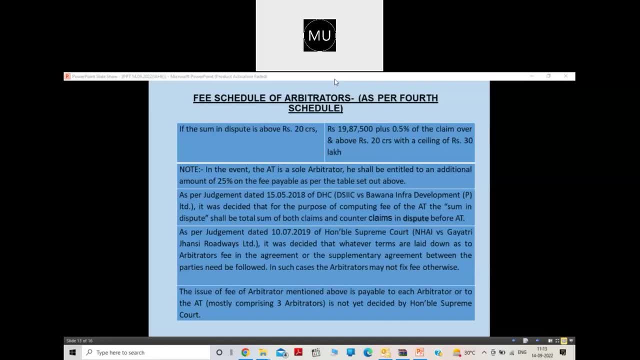 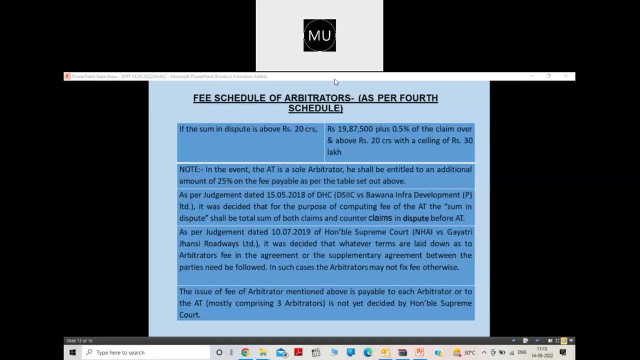 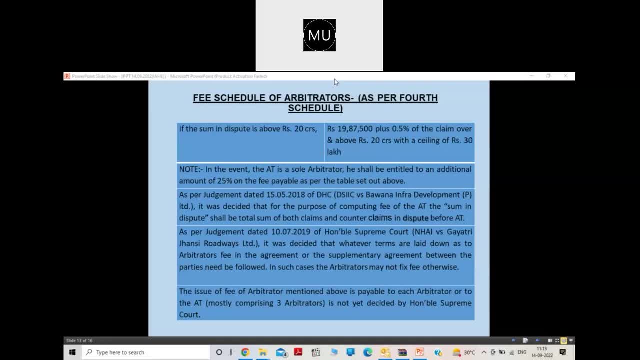 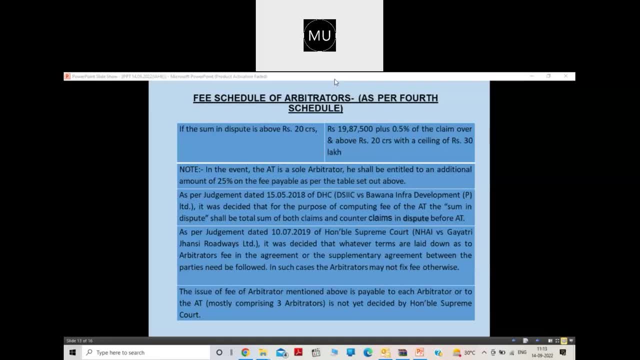 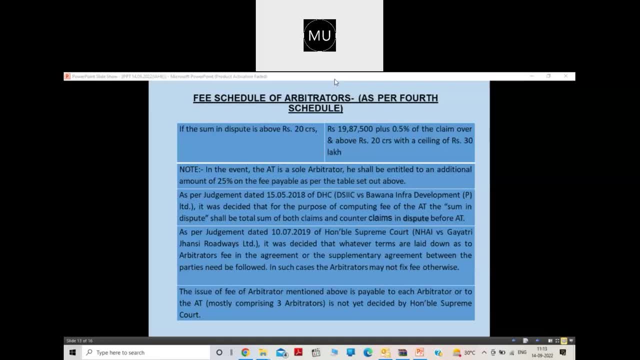 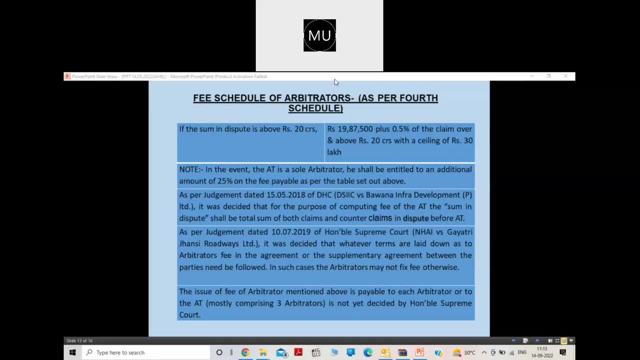 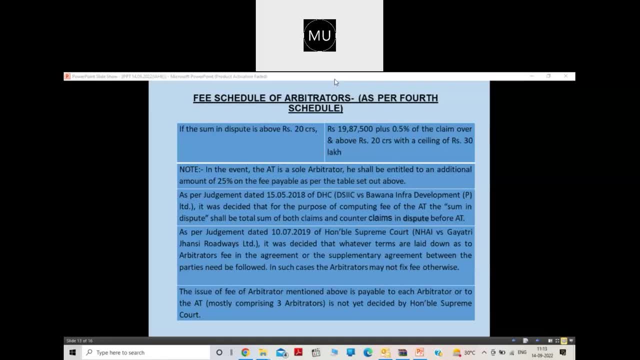 om. CCIE was introduced sometime in 2017 and ERB provision was initiated or introduced in 2020 during the COVID period, and it was successfully reduced and accepted by the contractor Initially. when the contracts- ongoing contracts- are there, we have requested all the contractors 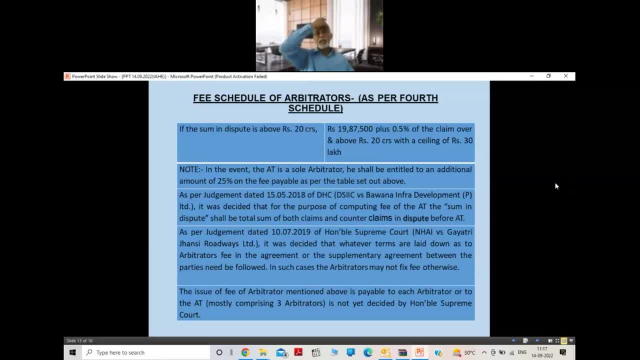 and concessionaires To enter into a supplementary agreement for introduction of the DRV mechanism after filling the cancellation process, sorry, the mediation process before the cancellation. So we have, I think, 47 or 48 contracts. In 47 or 48 cases the supplementary agreement initially was entered into and the DRV was. 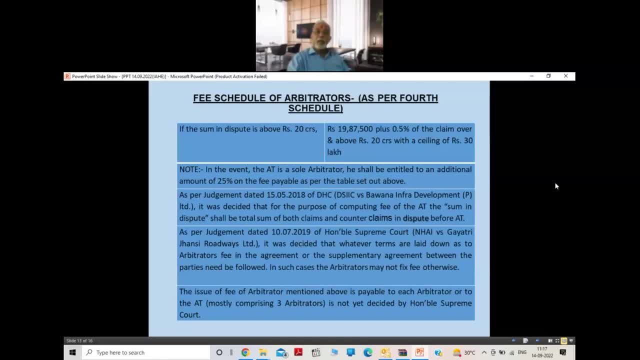 constituted. Subsequently, the contract provision has been revised and the Article 26 or Article 38, we have introduced this DRV and it is now in all the contracts. The provision of DRV has been introduced. Presently we are having 190 DRV already constituted and they are in the process of progress in progress. 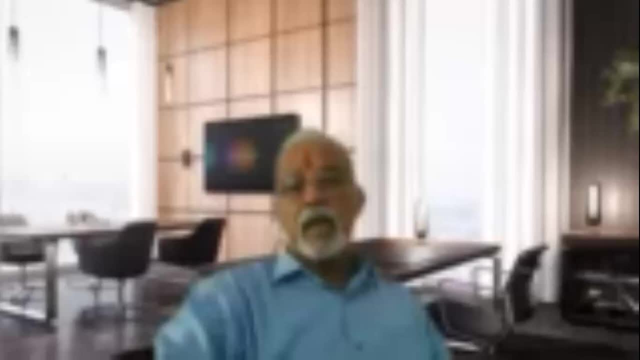 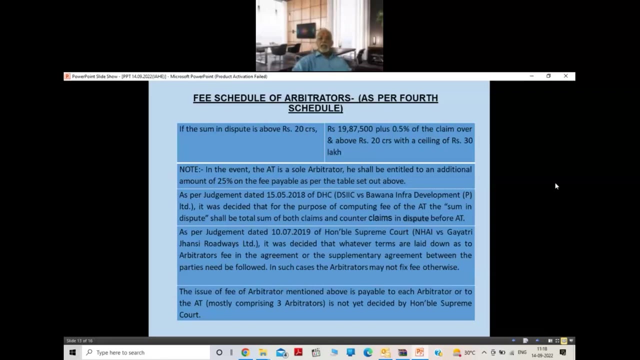 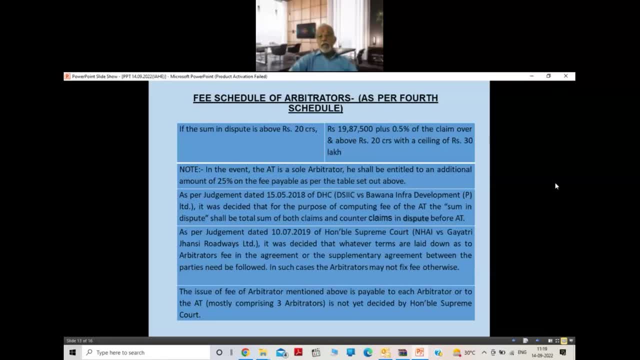 Thank you. And there is the feedback that we have received from the State PWDs, Ministry of Road Transport, Board of Road Management, MES, CPWD, etc. etc. and some of the senior retired bureaucrats are also there who have dealt with the senior retired bureaucrats here. 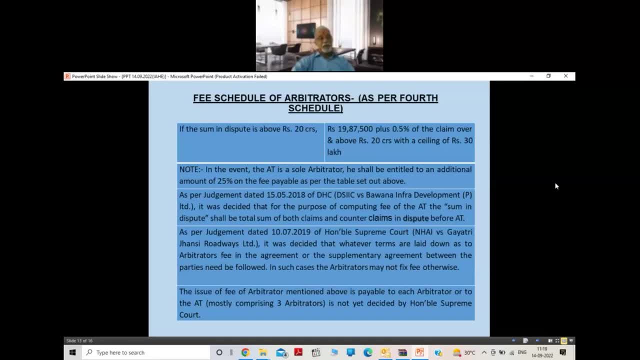 Thank you, the highway construction in their states or in centers like Secretary, MRTH, etc. And it is going to be increased because the number of contracts awarded where the DRB has not yet been constituted are almost in 100 or so. So we are planning to constitute another 100 DRBs in the near future. 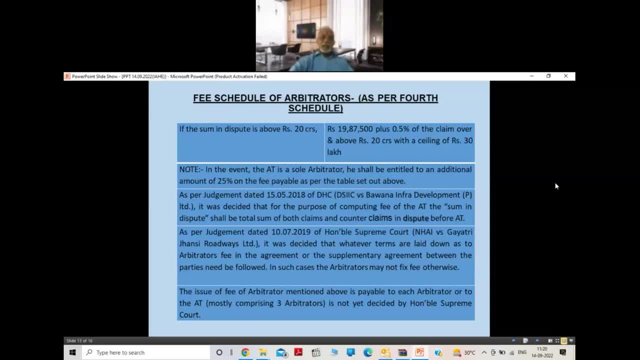 So if any issue is not settled in DRB, then the matter referred to consideration And the consideration. If the consideration fails, then we refer the matter to the arbitral tribunal. Now, as I told you earlier that in 2015,, they have amended the Arbitration Conciliation Act, 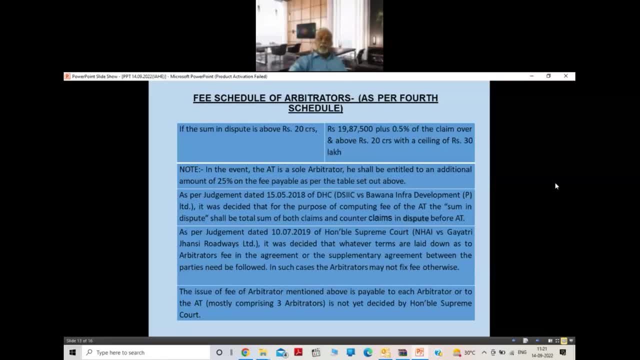 And first of all I will come to the provisions of this arbitral arbitration. It provides that in case the value of contract is less than 50 crores, a sole arbitrator may be appointed, if accepted by the parties, and fast-track procedure shall be adopted as laid down in Section 29B of Arbitration Conciliation Act 1996.. 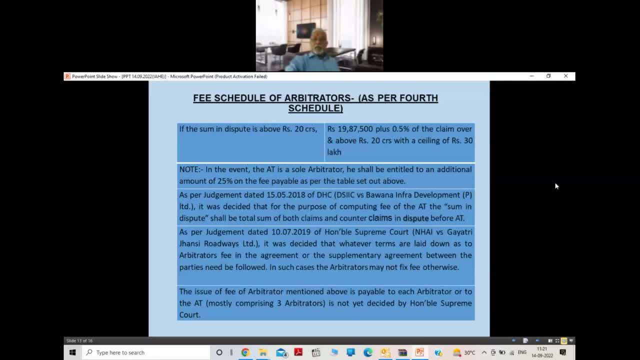 Now, if any party, if the party is accepted, then fine enough. the sole arbitrator is appointed, with mutual consent Or otherwise, the tribunal of three arbitrators can be constituted, And each party will nominate Both the arbitrators, select or appoint the third arbitrator as the presiding arbitrator. 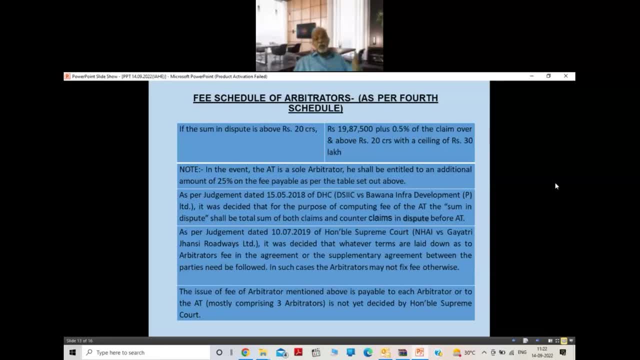 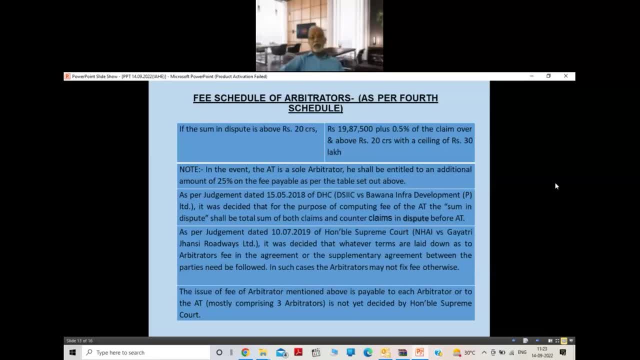 of ICA, Indian Council of Arbitration. In some cases it is written ICADR, In some cases it is mentioned IRCA, etc. etc. Somewhere it is said that it will be conducted under the Arbitration Constellation Act 1996. that is called Ad-hoc Arbitration. 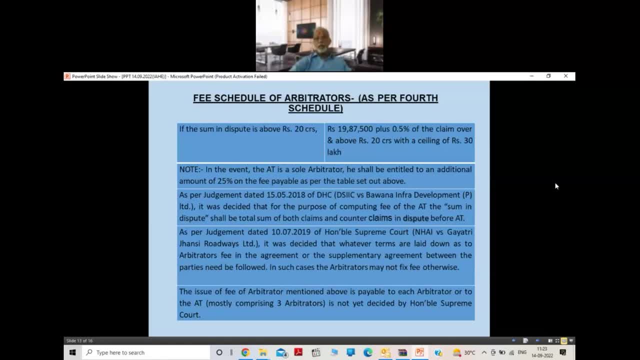 So it was subsequently thought that why not a separate institution is created where the NHI and the builders- the director of NHI or builders together perform company sort of a thing. So then a Sarod was created. Sarod is the Society for Affordable Redressal of Disputes. 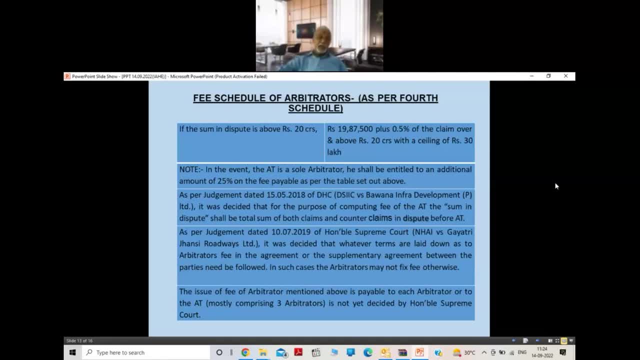 So this is incorporated in October 2013 by NHI, along with National Highway Builders Federation, for Settlement of Dispute through Arbitration in a cost-effective and time-bound manner. So in 2013 itself, when this society was created, the rules, regulations and the fee schedule, etc. etc. procedure, etc. 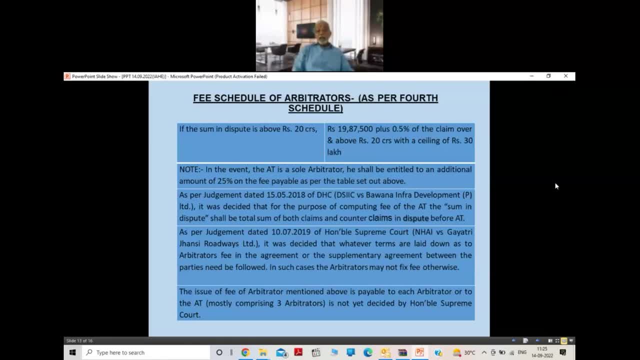 everything was framed. This was registered in the Companies' Act. this Society is registered in the Companies' Act. So at that point in time, the rules of Sarod was framed by us, by NHI, wherein we have provided that that if any arbitration is conducted under the rules of Sarod, the award is to be published. within 12 months and further extendable 6 months with the mutual consent. 18 months maximum. in 18 months. the award is to be published. This was introduced by us in 2013,, which was subsequently introduced in the amendment of. 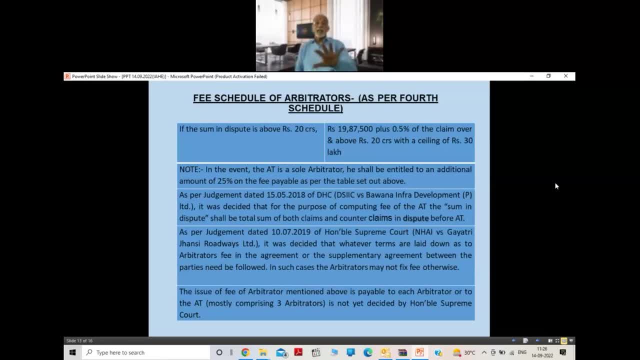 the reconciliation act of 2014.. Each lament board is having 8 governing body members, and 4 members are from NHDI and 4 members are from NHBF. The main objective of Sarod is to reduce cost of arbitration for expeditious disposal of 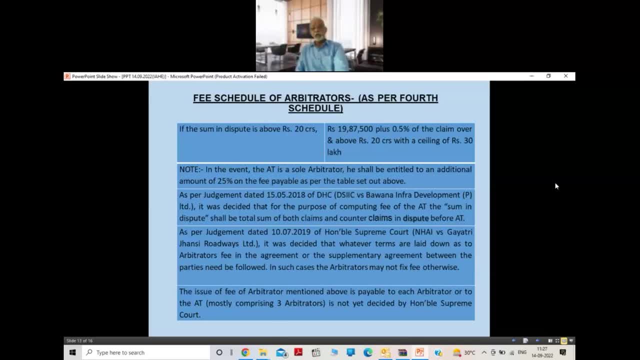 dispute in a fair and just manner, reduce the pregnancy of dispute. all subject matters: technical experts in arbitration process. So initially, when this provision was not introduced in a correct agreement, supplementary agreement has been heard between HIMB concessionaire and the Commission. It has given a very good result and it is still going on. 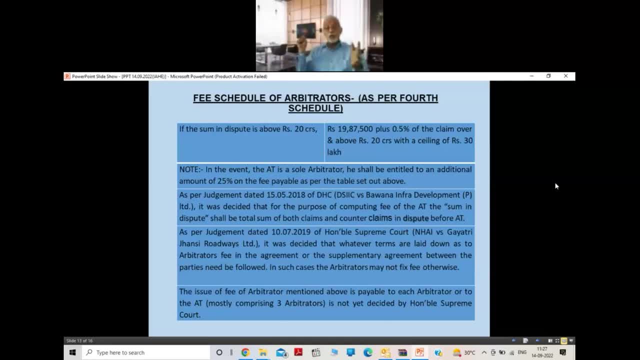 Now, in the contract itself, the provision has been made that the arbitration will be conducted under the rules of Servo. Presently, the T8 arbitrators are empanelled with Servo. This is the brief of the Servo functioning. Now I will present the status of cases in NHI Presently, in fact a month back- 632 awards have already been pronounced so far, where the claim amount was around Rs 47,000.. And the awarded amount was MasterCharge. around 15,600 crores And out of this 632, presently 232 are in court. The rest other awards have been accepted by both the parties and the matter has been resolved. Presently, 136 arbitration cases are in progress in NHI. 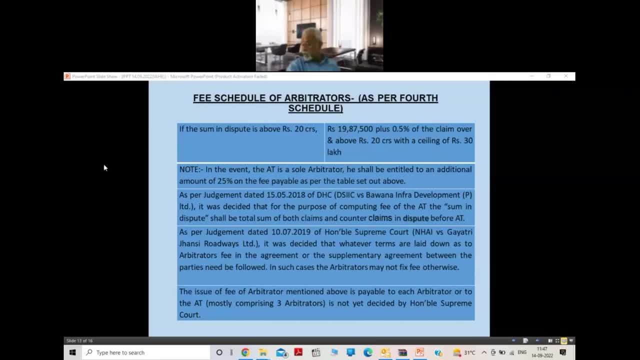 wherein the claim amount is around 1,200,000 crores and the counter claim is approximately 44,000 crores. So, if we can see, the total is around 1,200,000 crores worth of claims or counter claims are pending. 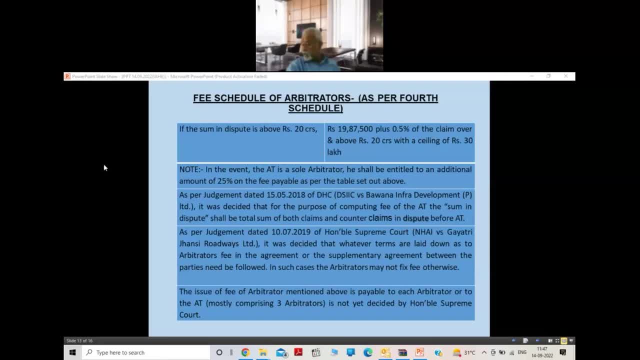 presently in arbitration, The semi-cable settlement, as we have already discussed. Conciliation: I have already told you about So in the conciliation by CCIE 100,000 cases have been resolved till date For the claimed amount was 44,000. 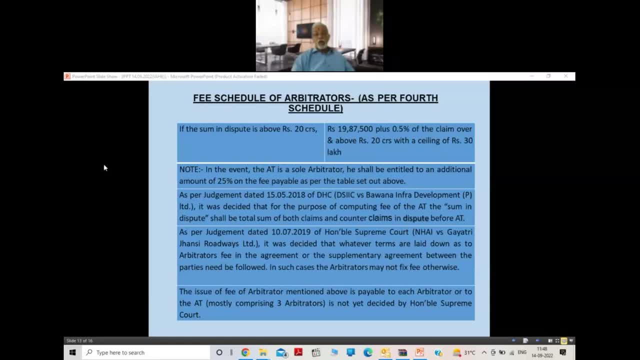 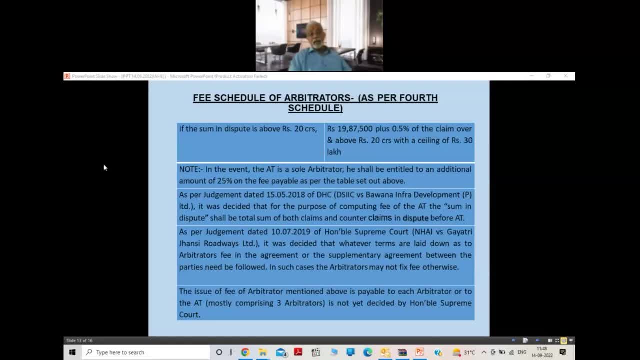 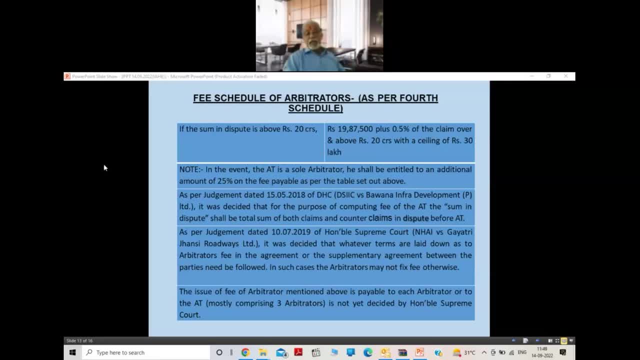 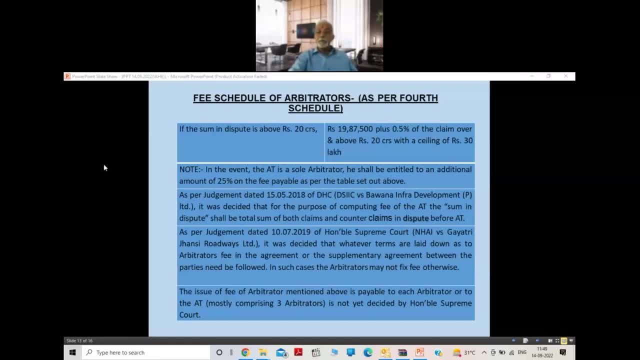 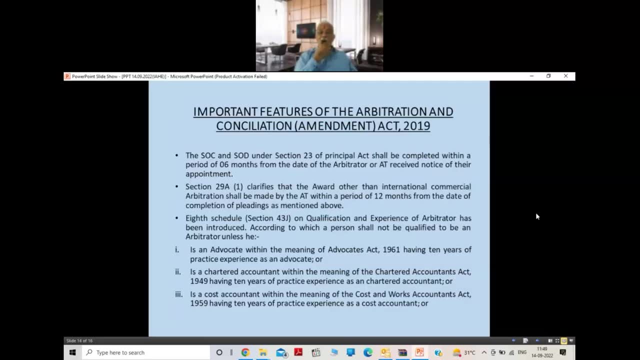 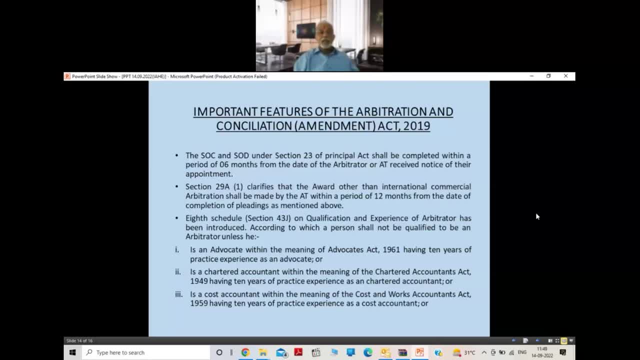 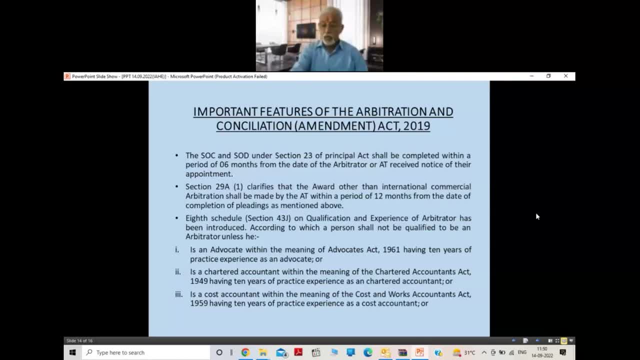 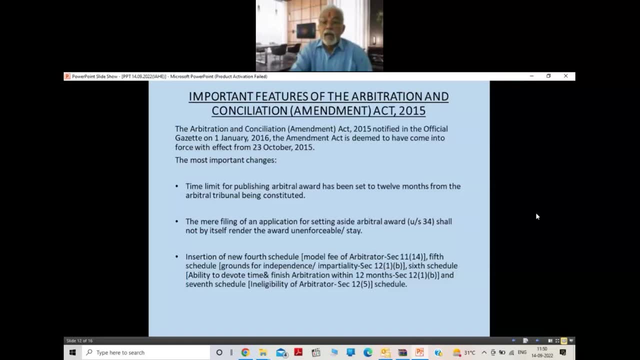 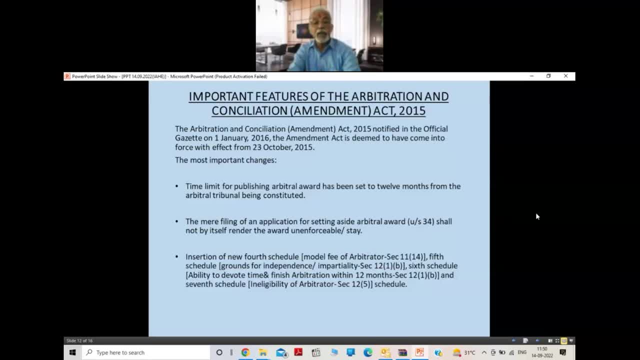 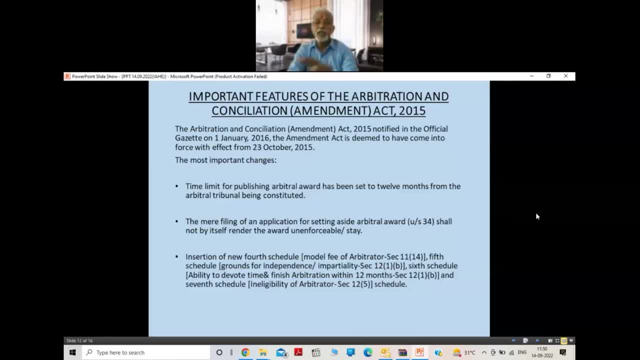 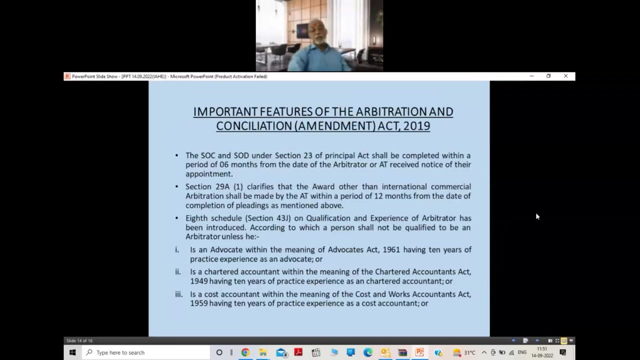 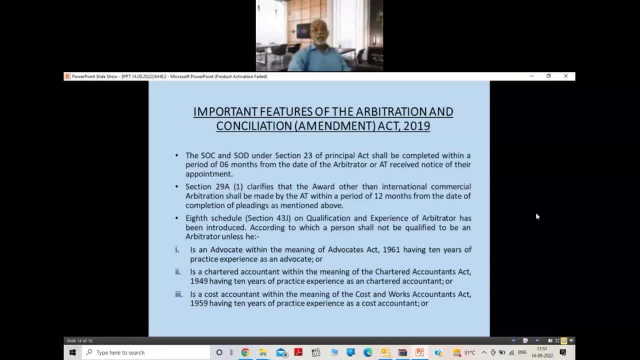 Sir, one query is there, sir. sorry, can I one query is there? yeah, yeah, sir, my name is Dilip Patil. okay, this is regarding this 75% amount of the decree. yeah, actually what? 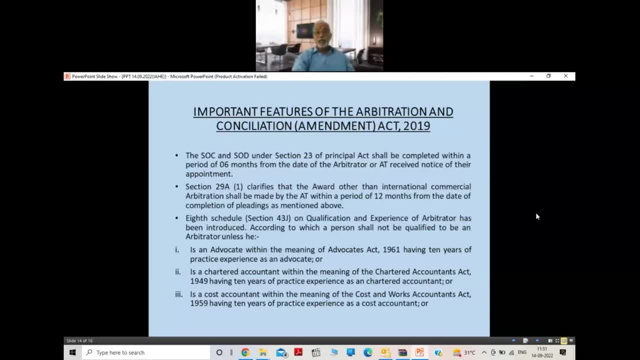 is happening right now that Honourable Delhi High Court is directing the authority to deposit the amount of rupees 3,400 crores and amount of rupees 3,400 crores and amount of rupees 3,400 crores and then only the conditional stay will be given. deposit. deposit the 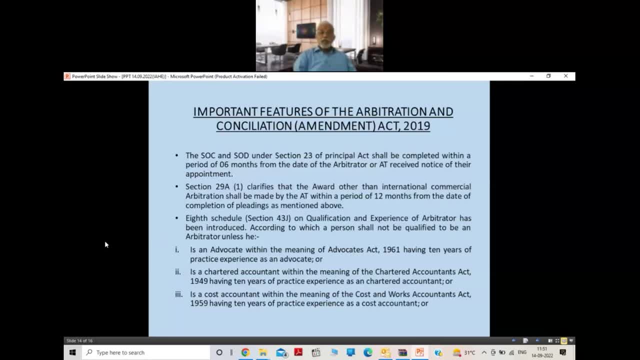 full degree amount. whatever this award, award is there, we are being directed to deposit the full amount. okay, yeah, okay, fine enough. so what is your query in that, sir? in that case, then, this actually the logic behind this: 75% was there to infuse the liquidity in the system and 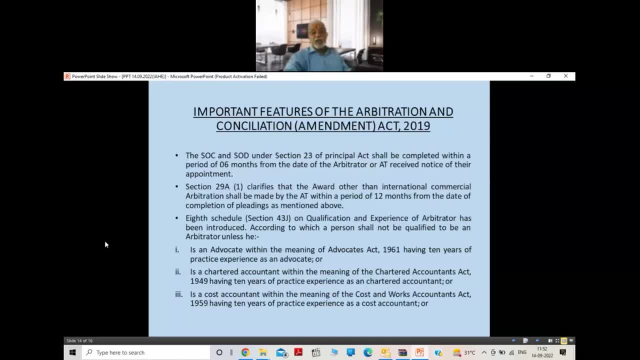 to give some kind of relief and in this High Court now directing to deposit 100%, and then these, these concessionaires are applying for this release of that amount without that to, without any this collateral securities and all these things. it is going on like. 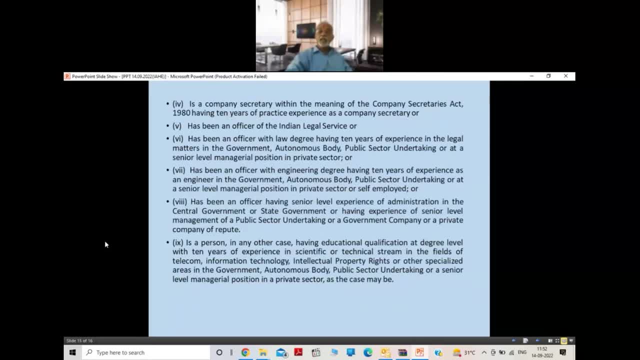 that, sir. So court is releasing that amount without having any bank guarantee or anything. We have deposited with the court registry because the Honourable Court directed us to deposit the full amount. why deposit the amount with the court register now that concessionaire? 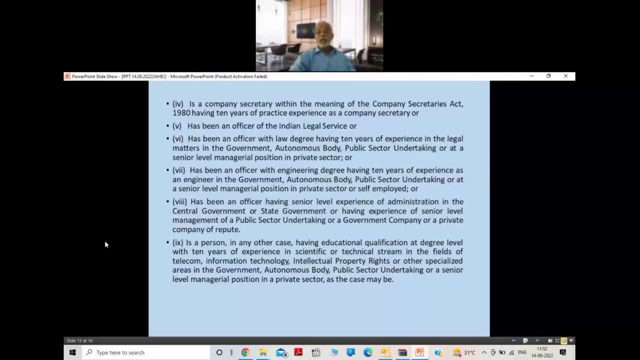 has applied to the court register that I am in financial distress and this amount will be released to me, and that, too, without collateral. so this the complete bill By now. you know this, sir. Yep, I understand, But, sir, what is the spirit behind this? 75% of this Niti Aayog circular is being jeopardized. 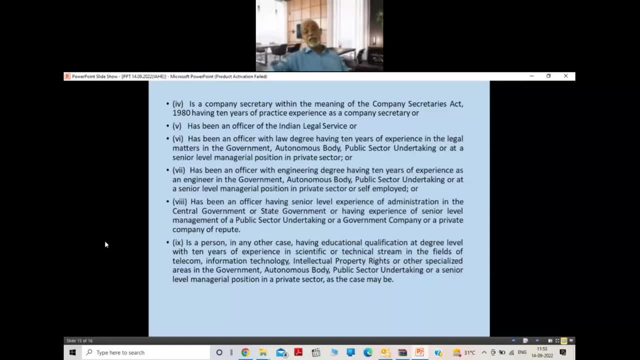 by this development. yes, sir, You are right. you are right. I have not heard about the 100% amount is to be deposited, as directed by the court. Actually, it is Justice Vibhu Bakroo's court has directed. sir, you know one of our clients. 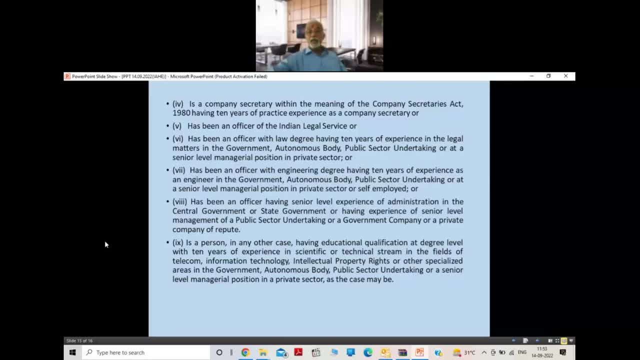 not our loan, not this one. John, do you have any comments? Sure, No, Thank you. Thank you, Sir. No cases, Fine enough What I heard here in Delhi, High Court has directed to deposit either 50%. 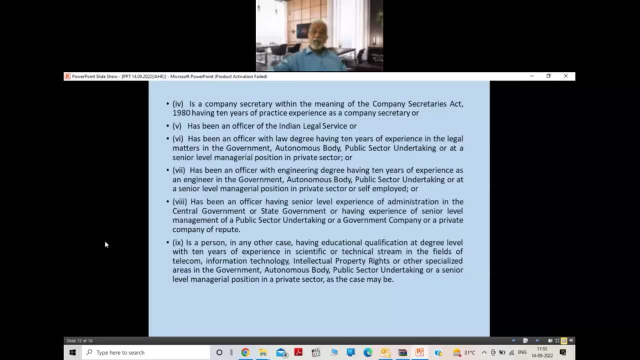 of the decretal amount, or, sorry, the arbitral amount, or maximum to the 75%. But see, once the court has directed, we have nothing to worry about. We have to deposit it. We have no say, We cannot. if you want. 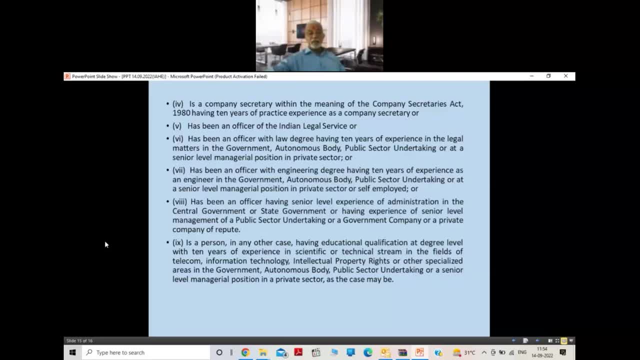 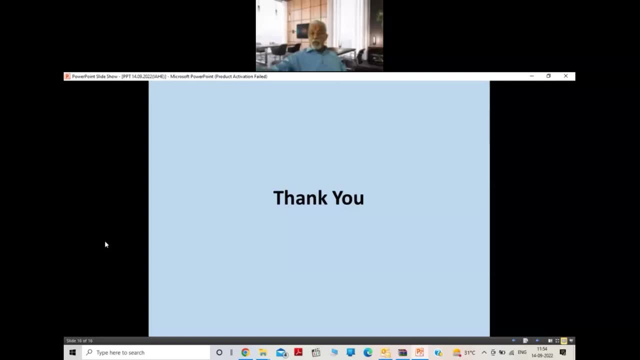 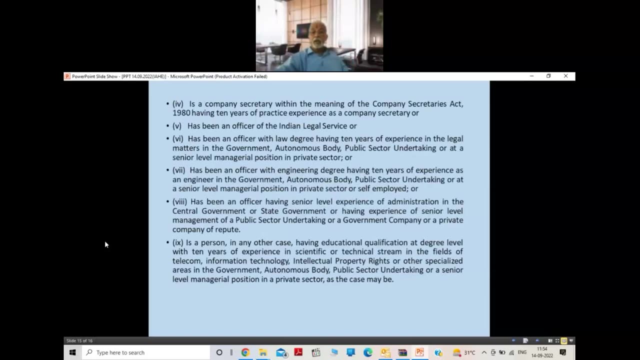 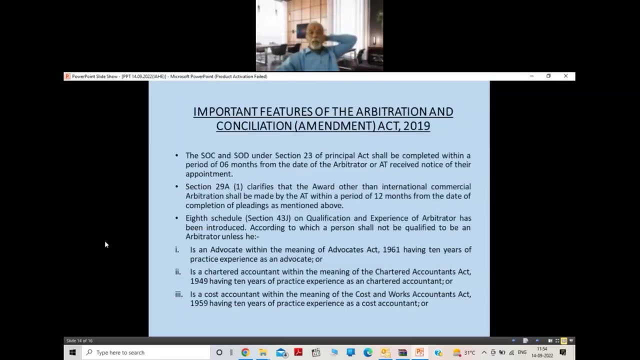 to challenge it. you can go and challenge it, But it is better to deposit it. But this is the responsibility of the court that in case if they release the payment without any collateral security, then I don't think court will release without having any bank guarantee. 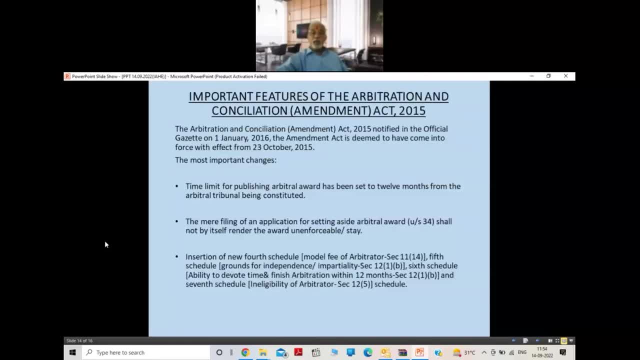 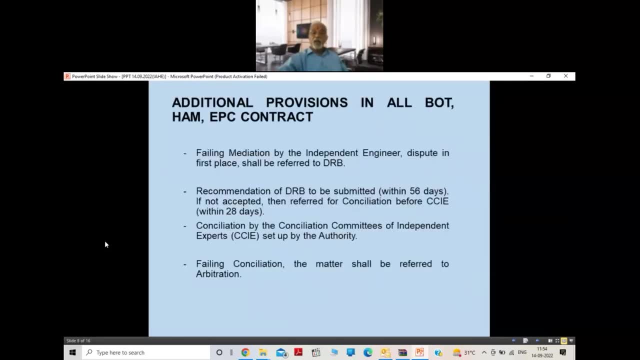 or anything from the concessionaire before release of they have. in your case, you are telling that they have asked for release of payment without submitting any collateral security. Yes, actually there is. a concessionaire has applied, with the difference that it is facing a lot of. 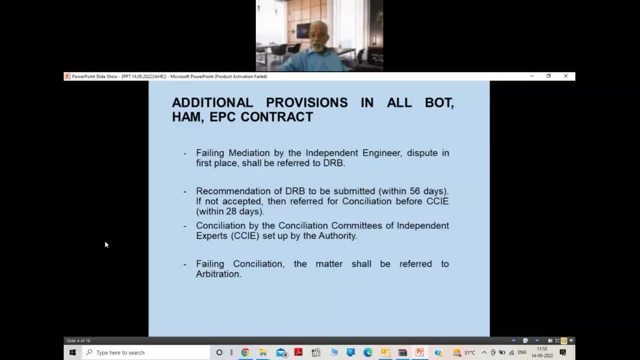 financial restraints and so they will release 100%. But I don't think the court will allow that. The court will never allow without any guarantee. They will not release a single penny. If they have asked for 100%, it is not necessary. 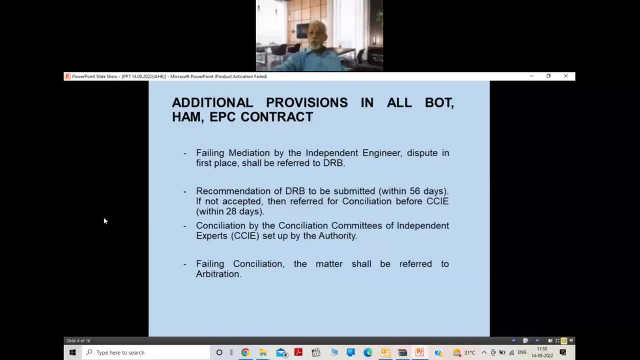 that the court will release the 100% amount. They can release only 50%. They can release 75%, But definitely, definitely, without getting any guarantee or any other security they will not release. Sir, can we take defense of civil procedure code? 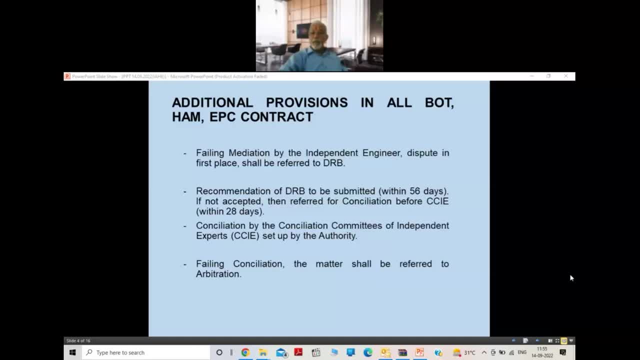 in this for being a state instrumentality. Can we take that defense that we may be exempted from the deposit of a wide amount or a little amount, like in court registry? CPC is not applicable in our arbitration, but more and less They. 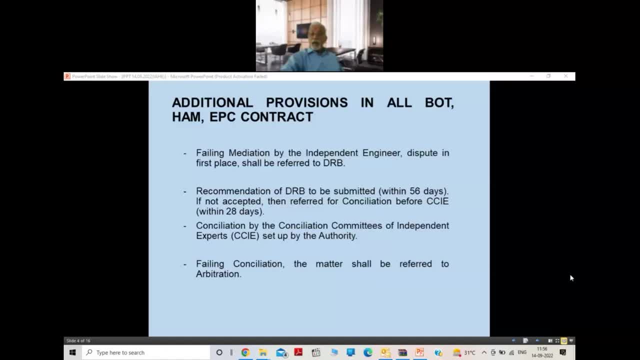 They do go for this because, in the manner of the deposit of this, I underground and and what I want to see? I'm, I'm, I'm sorry, I'm not a legal person, so I don't have any idea about this, but the legal person or I don't. I'm a person, so I don't have any idea about this. but that's very ticketed to my все trades. in this law The clams Ni freed in under 30s, Но card الص którym. 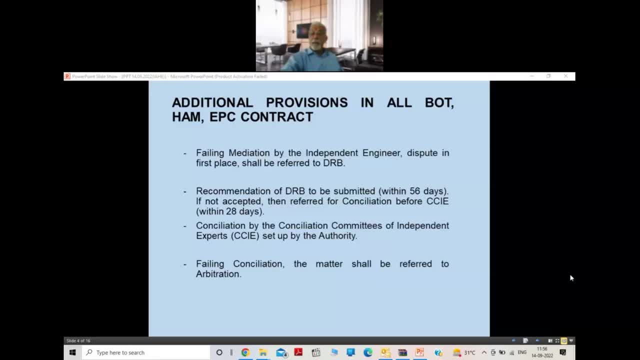 There is nothing that can Емест как i'll. i'll, yes, i'll note it down. i'll come back to you. you, you, you are mr patil. yes, sir, what is your initials? mr delhi patil, delhi patil. yes, so you are basically from. 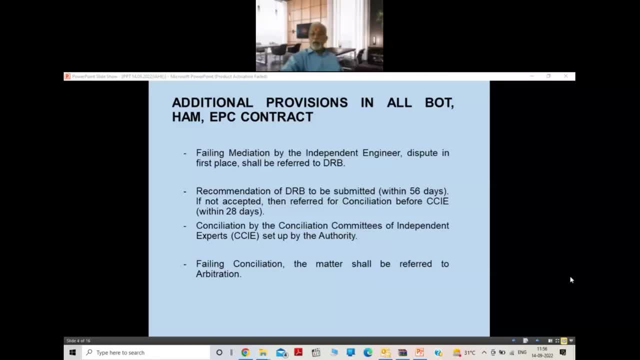 nhsi sir, i'm from the nhsi nhsi nhsi. yes, sir, nhsi was our opponent. he was a claimant opponent and that award went to his favor. and then court directed us to deposit which court delhi i got. yes, sir, okay, okay, let me see. 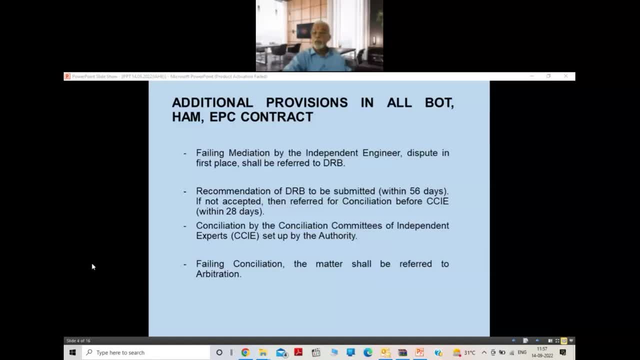 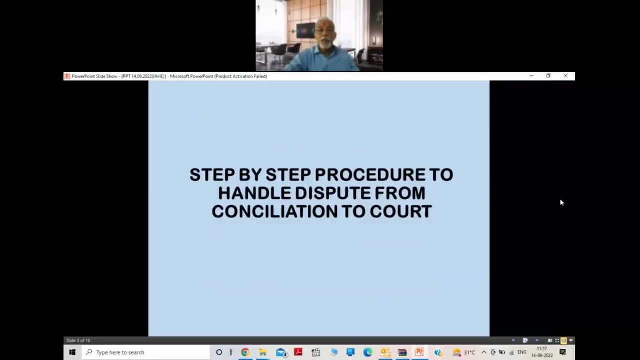 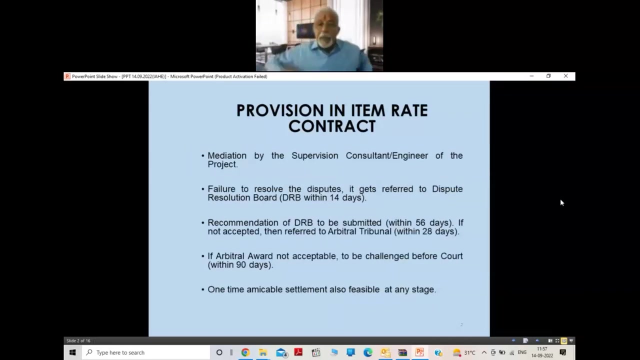 who is the concessionaire? isdpl, that is the irkon soma. okay, yeah, and singhania was our, singhania is the lawful, yeah, yeah. so we were also surprised that how can they go directly normally? yeah, yeah, yeah, 100, i heard. i i'm hearing this first time that who has directed? 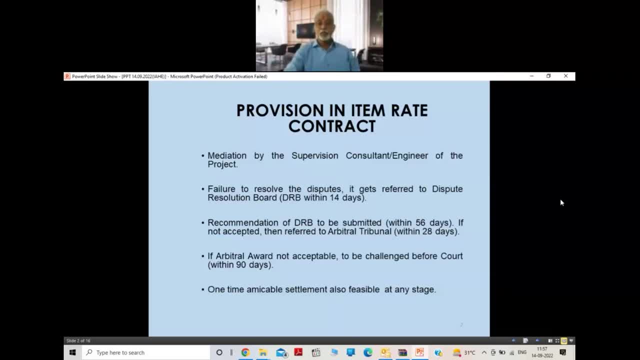 to deposit 100 percent. okay, okay, uh, you are posted where. okay, yes, your Ro has changed. is your? your under raunagpur has changed. yeah, okay, oh, oh, okay, okay, uh. I'll come back to you, mr patil, then i'll let you know what what. 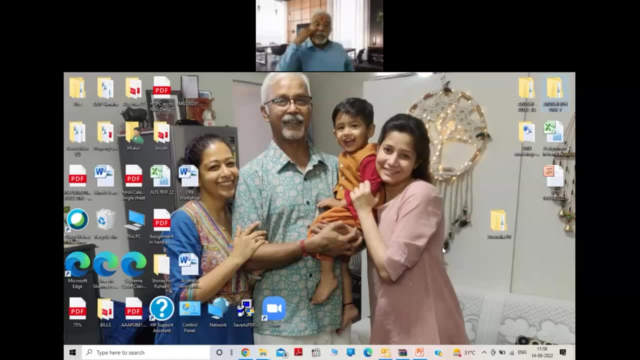 exactly is要out給您? what exactly is to be done? Yes, sir, Thank you sir. These are some of the common dispute or issues. as far as the item rate contract is concerned, We have seen, we have observed following disputes are: 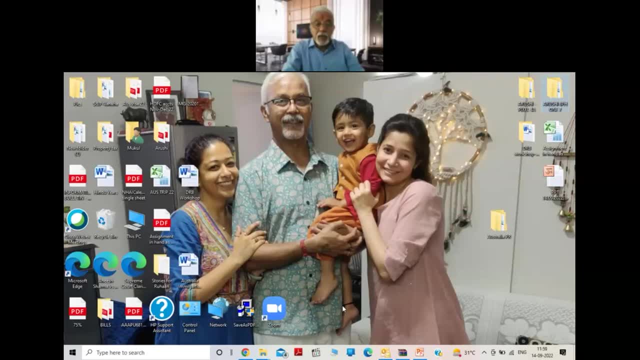 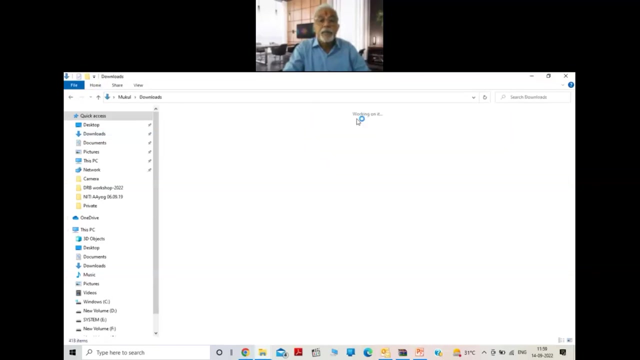 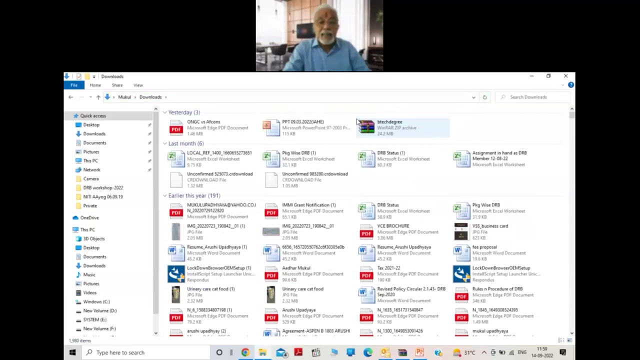 very common in all arbitration cases in item rate contracts earlier, like the royalty charges, revised royalty charges on materials. So this issue has already been finalized by the Supreme Court, So now issue is resolved. Similarly, price escalation issue was there, which was also. 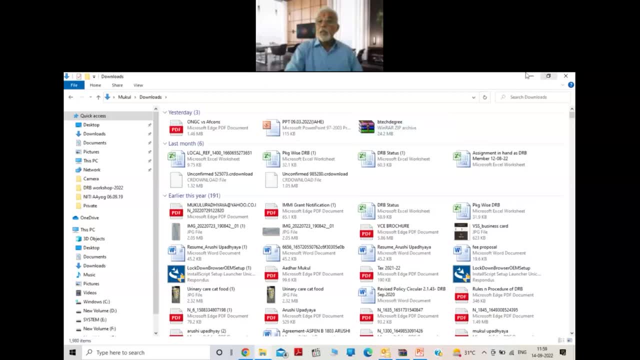 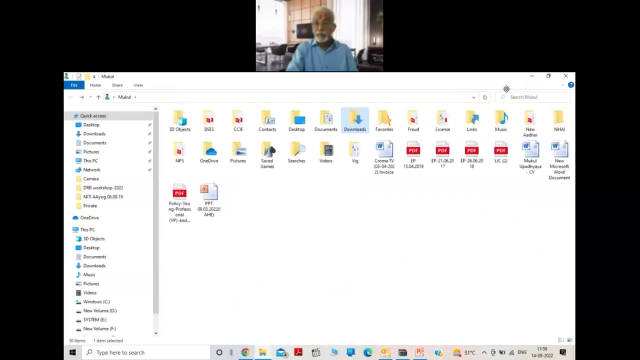 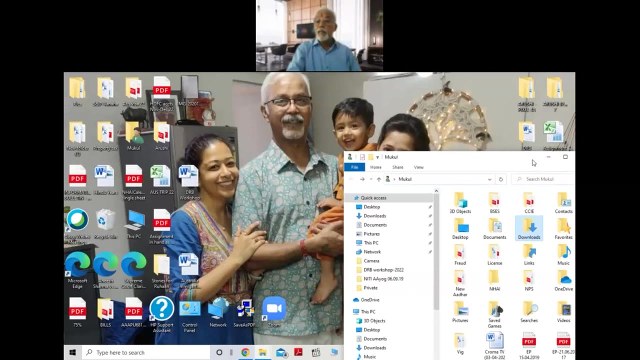 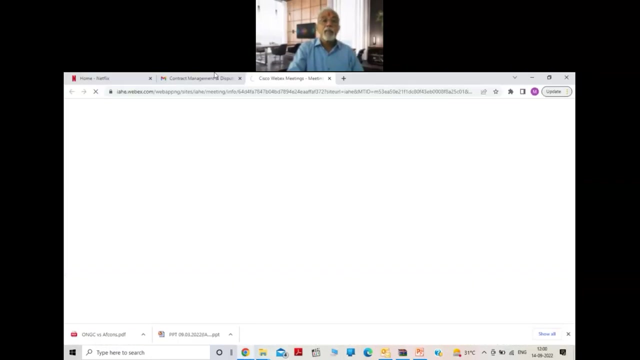 resolved by the Supreme Court. Forest transit fee was also there. This has already been resolved by the Supreme Court игры. One major issue: this applicability of construction worker's welfare, ses. This issue is pending since long and yet to be decided. 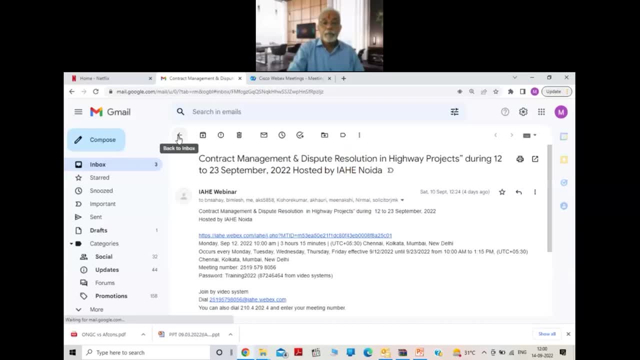 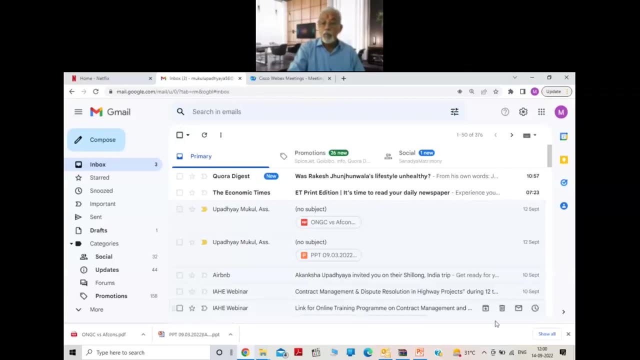 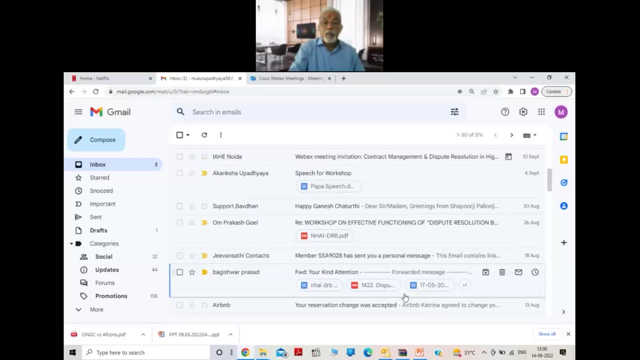 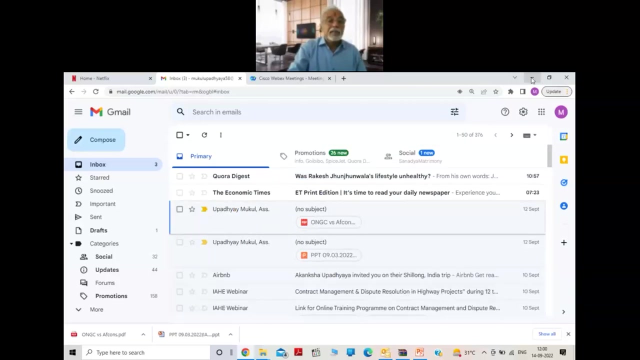 So this issue is pending is very small issue like clearing and grabbing the stump, removal etc. This issue was also referred to Supreme Court is still pending. Flyers issue is also pending in the Supreme Court for the construction of an amendment And some of the issues- common issues in BOT and MOT projects. Compensation on 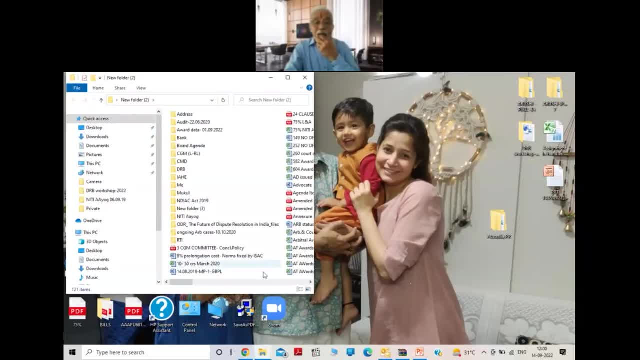 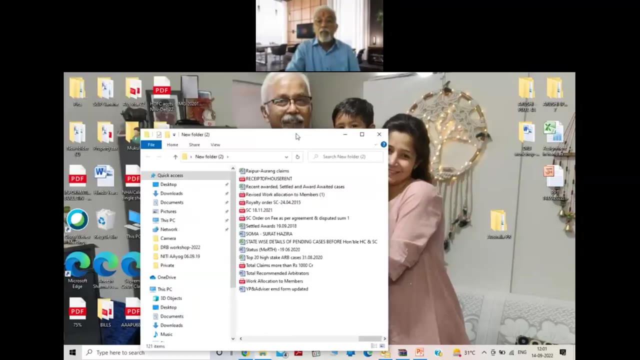 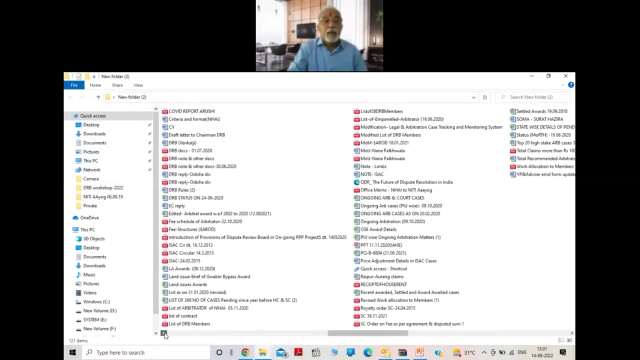 non-handling handing over or delaying handing over of the land. Land acquisition problem was there earlier, but now it has been decided that until and unless 90 percent land is available, the contract, the agreement will not be signed or the date will not be released or issued. 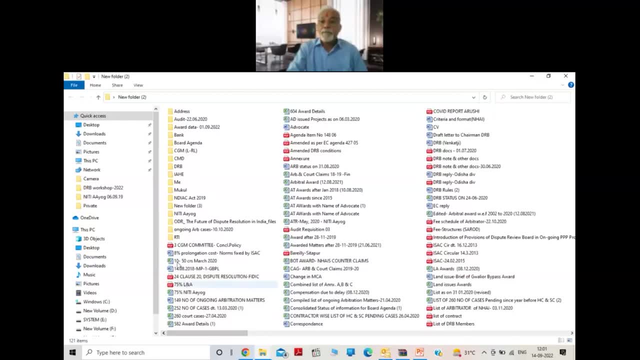 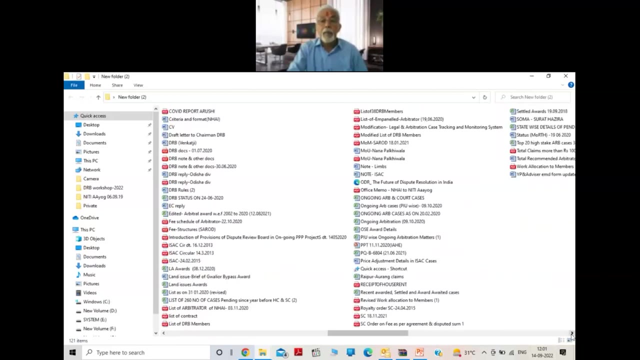 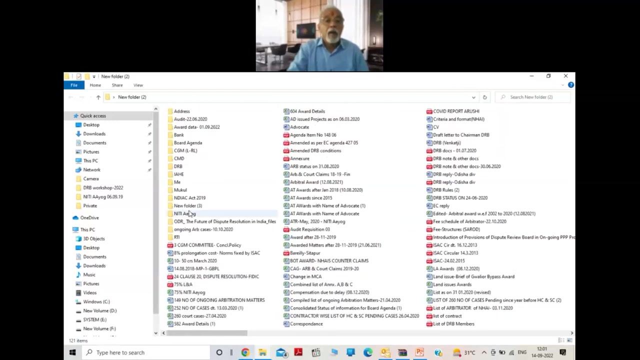 So this issue of land acquisition or compensation due to delay in handing over of land, I think will be resolved. COS is definitely one of the major issues: Change of scope and some losses towards additional utility of resources, Delay in distribution, disbursement of grant or annuity payment. 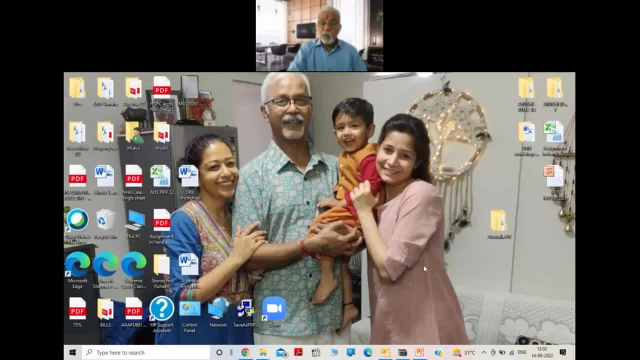 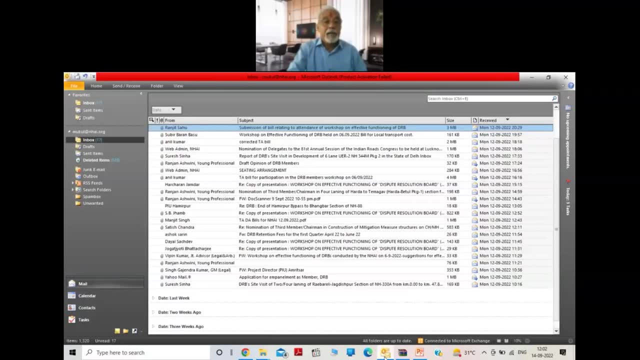 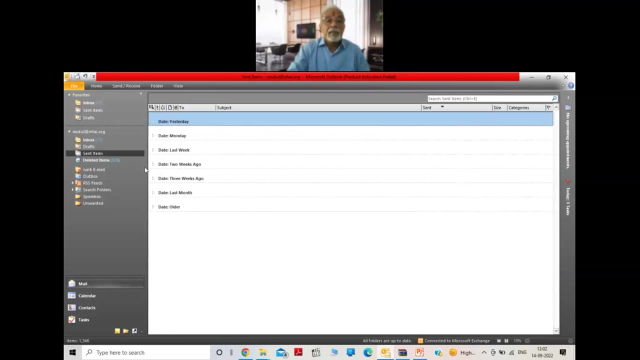 Change in law also is the issue in this DCM case: Damages on non-fulfillment of condition, precedence, Penalty for delaying the achievement, Losses of financial closure and losses of escalation on materials, additional interest paid to lender, etc. 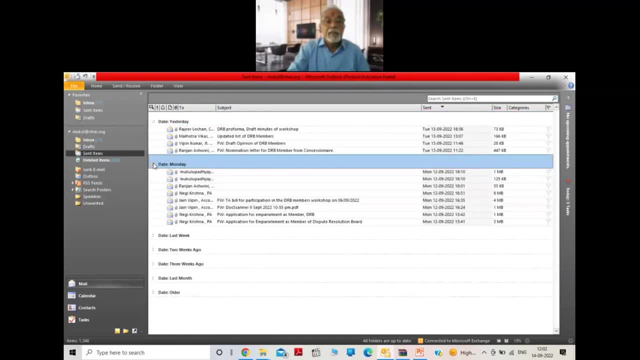 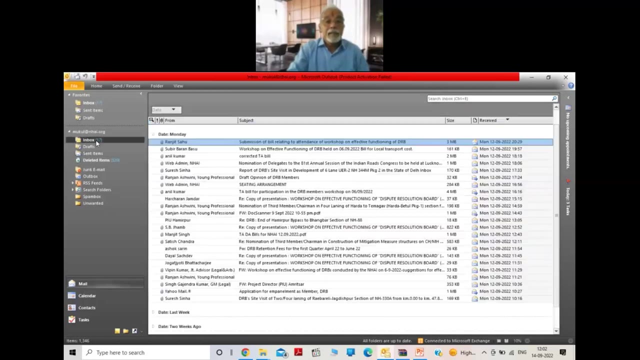 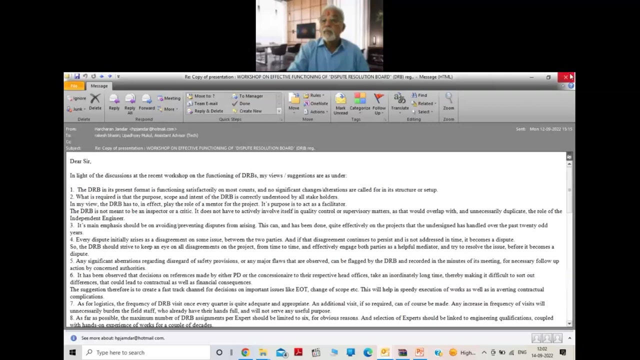 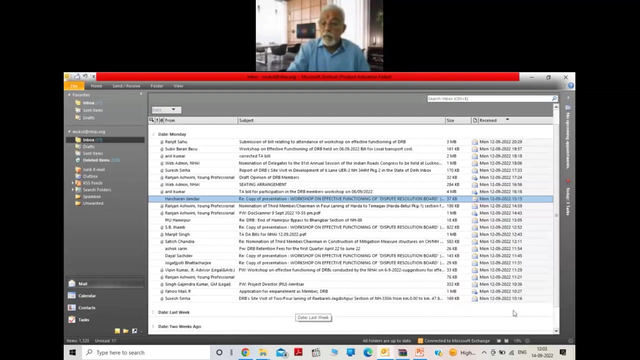 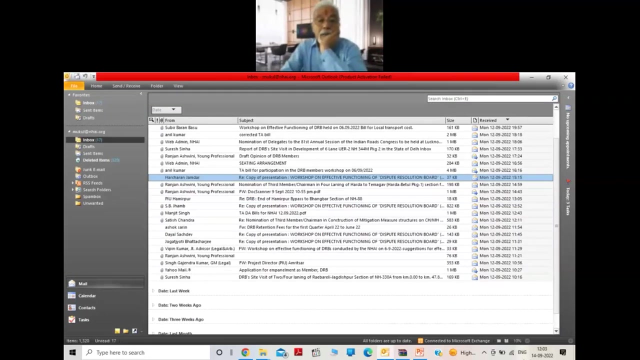 These are the common issues we observed when the arbitration is invoked in the BOT or PPP model cases. Now these are the important features of the Arbitration and Conciliation Amendment Act 2015.. The very important amendment was the time limit for publication. 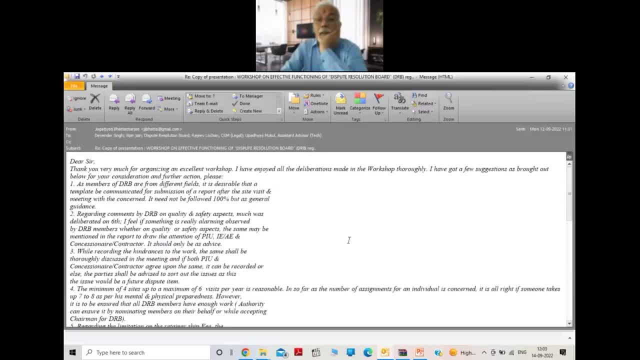 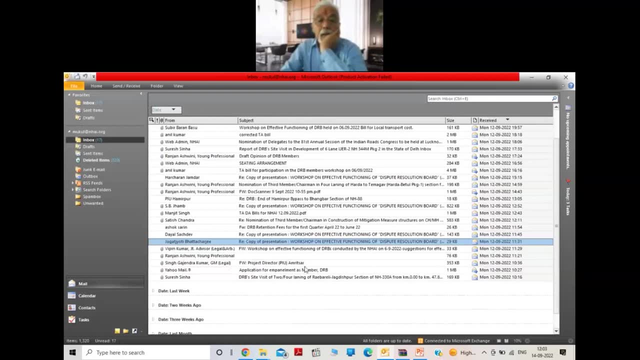 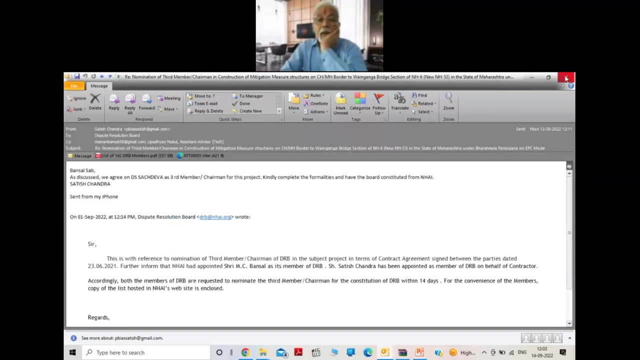 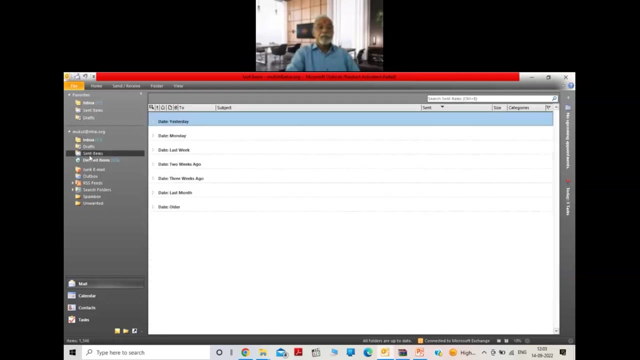 Publishing. the award has been set to 12 months. set to 12 months from the arbitral tribunal being constituted. Then, second here, 12 months time further can be extended for 6 months with mutual consent And in case that 6 months, the total 18 months time are exhausted and still the tribunal and the parties feel like that they want some more time. 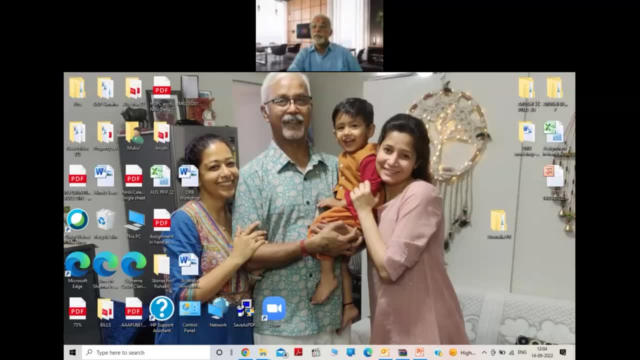 So the parties have to approach to the court and get it done from the court itself. Then after that completion of the 18 months time, the parties are not authorized or not increase the time limit for after 18 months. The second amendment was the 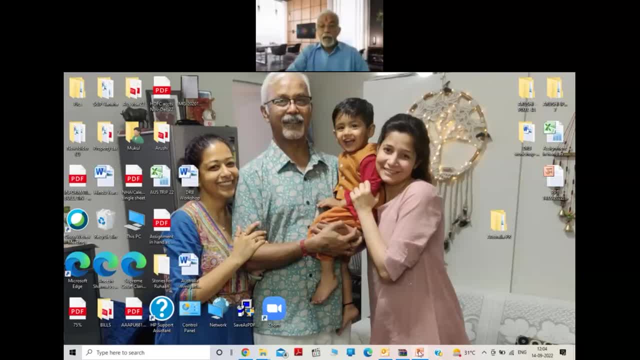 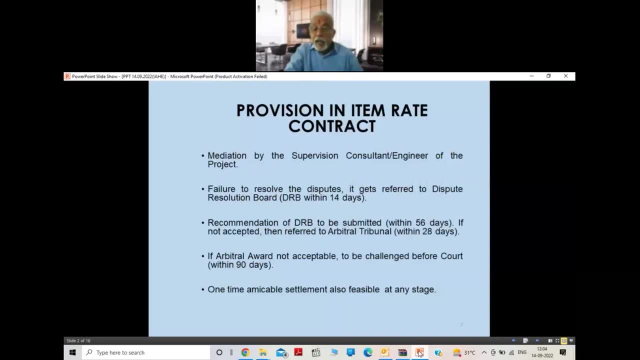 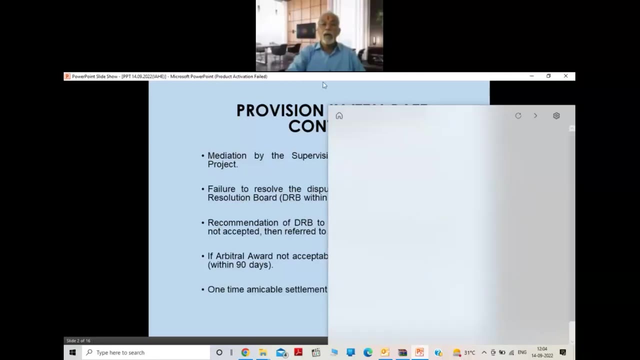 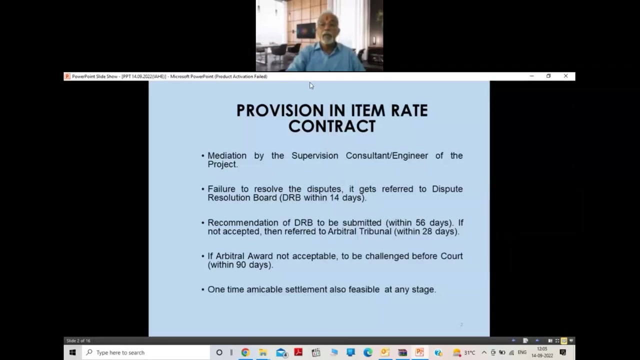 mere filing of an application for sale That is setting aside the arbitral award shall not by itself render the award strict. Section 34 application is filed for setting aside or challenging the arbitral award If that award needs to be stayed by the parties. 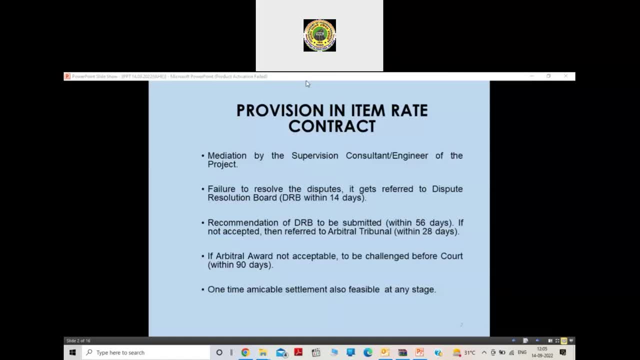 then they will have to file another application for staying the award. Earlier it was: as soon as the application under section 34 is filed, the award was automatically stayed. Now in the amendment, two different application needs to be filed for. 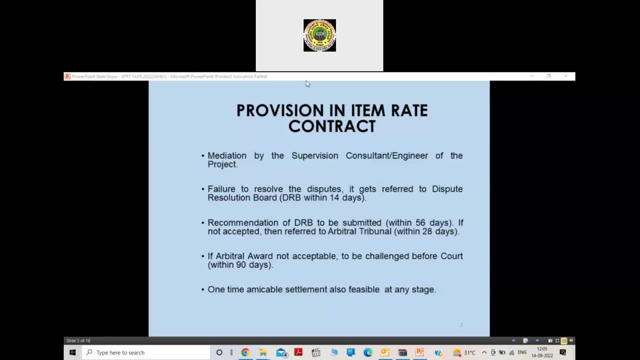 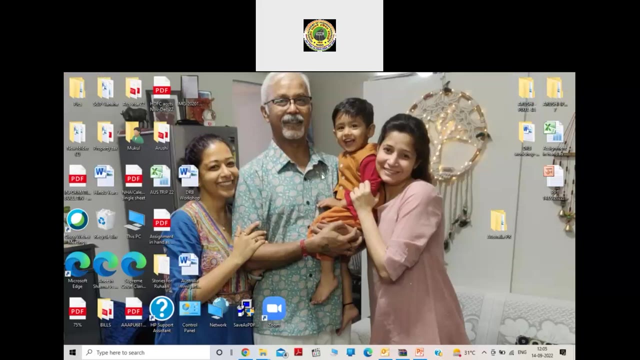 one for setting aside the arbitral award and another for staying the the implementation of the arbitral award. The fourth schedule has been introduced regarding the model fee of the arbitration. Fifth schedule was introduced on the grounds for impartiality and independence. 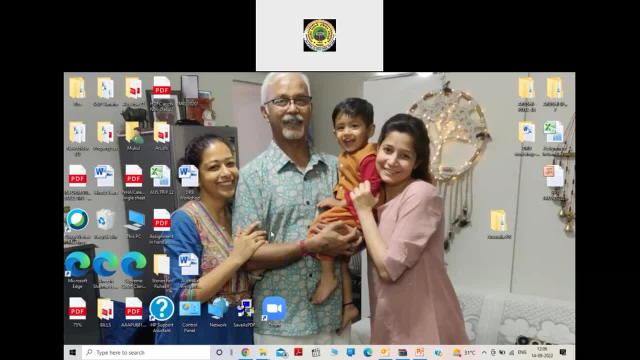 Sixth schedule was introduced to ability to devote time and finish arbitration within 12 months. And seventh schedule was introduced for eligibility and ineligibility of arbitrators, The qualification of arbitrator. Let me take just five minutes break. I will come back. 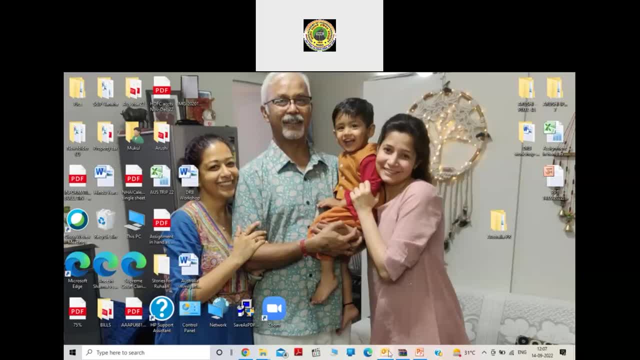 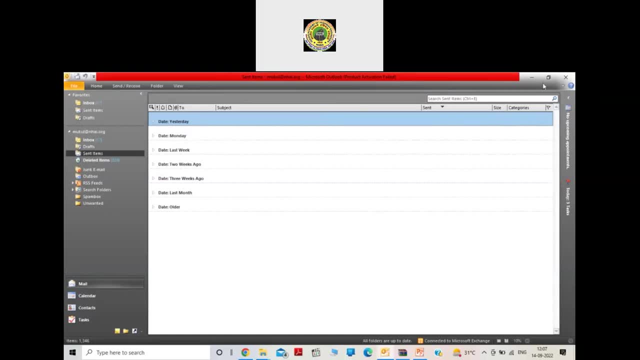 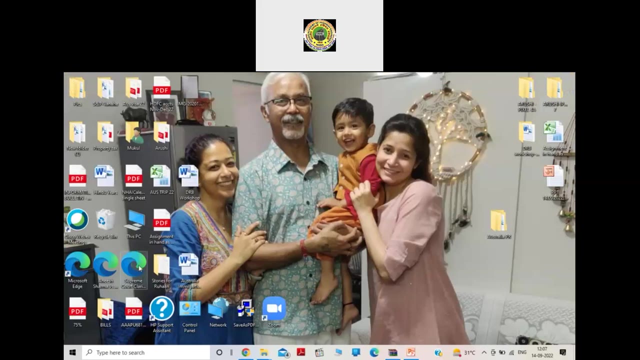 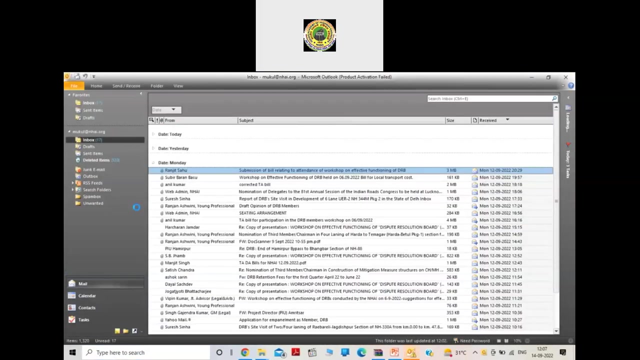 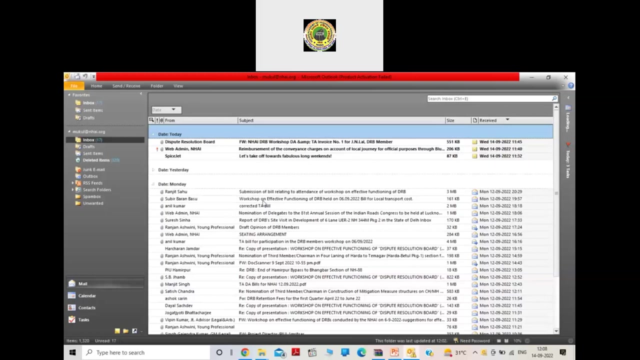 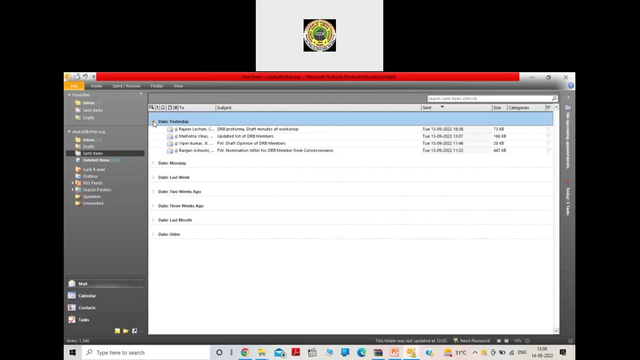 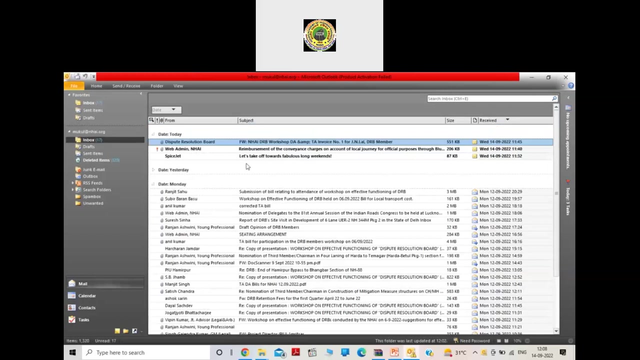 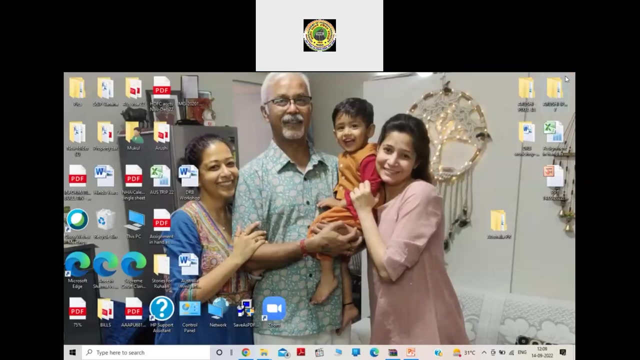 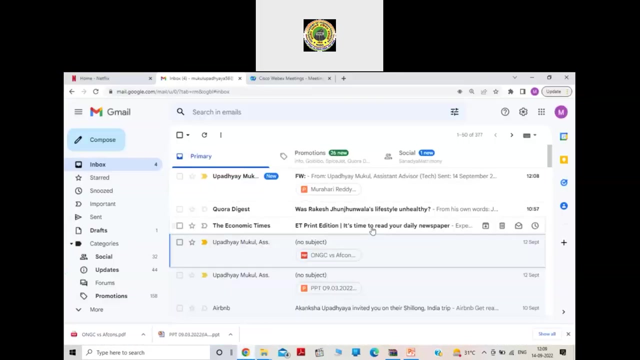 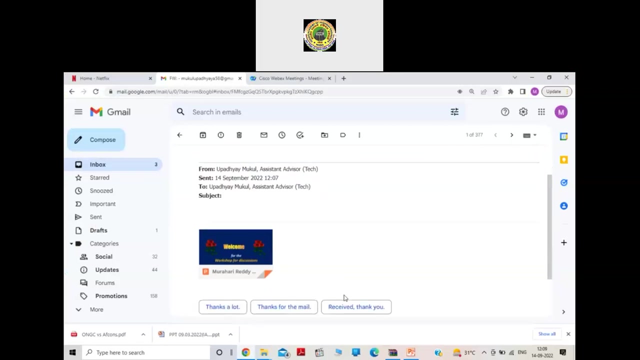 Thank you, Thank you, Thank you. I'll have to take this phone. please Excuse me one minute. Thank you, Sorry. Yes, this free schedule of arbitrators as far as the fourth schedule introduced in the amended Act of Arbitration 2015,. 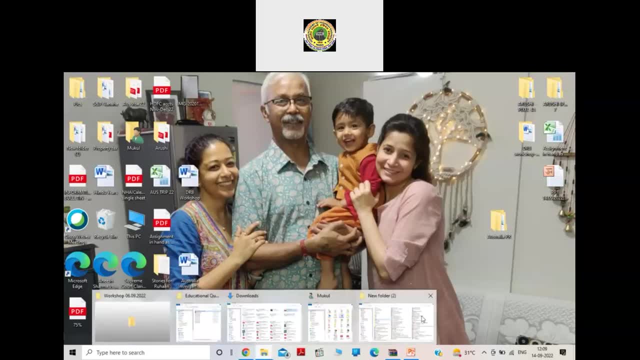 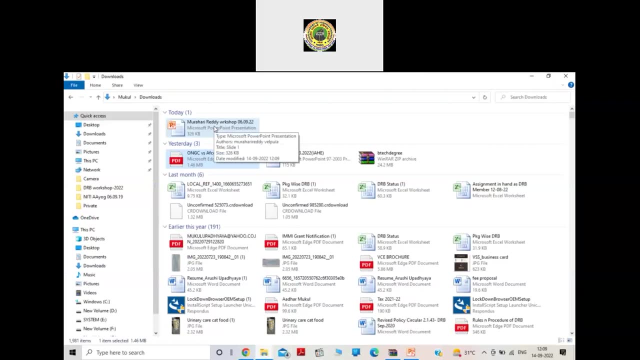 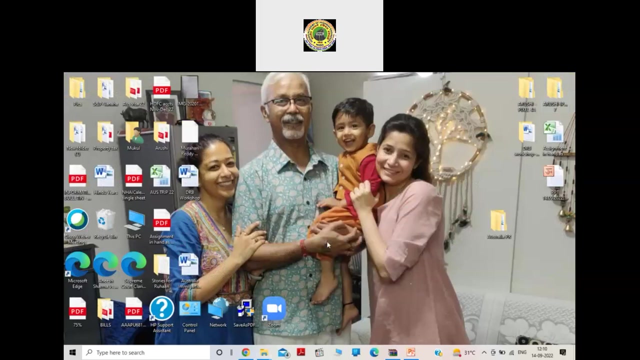 wherein I have taken only the last provision of the sum in dispute, because we are not having any case less than 20 crores worth of. So this says that if the sum in dispute is about 20 crores, in that case the 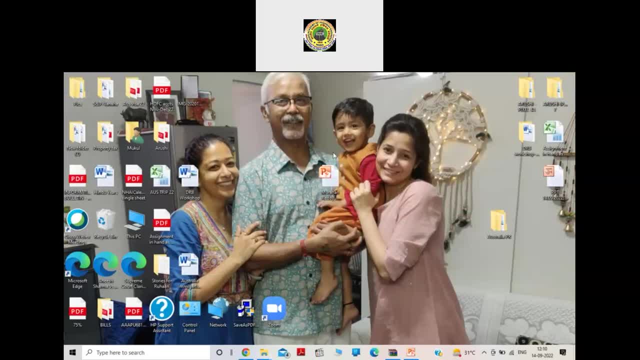 fee of the arbitrator will be 19,87,500 plus 0.5% of the claim over and above rupees 20 crores It means, and with a ceiling of 30 lakhs. So there were a lot of confusion. 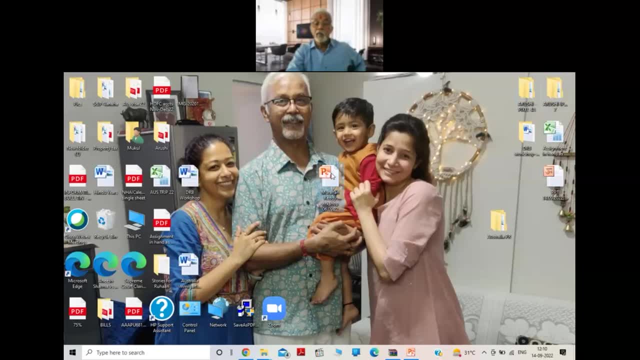 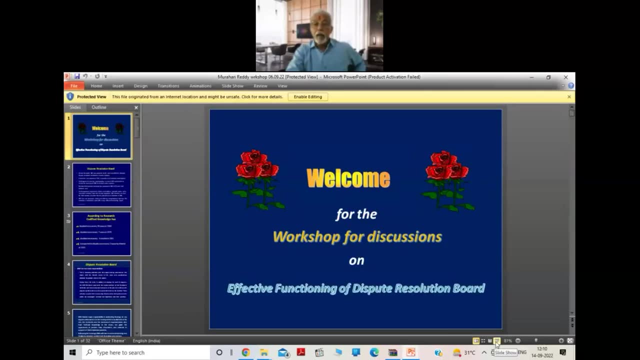 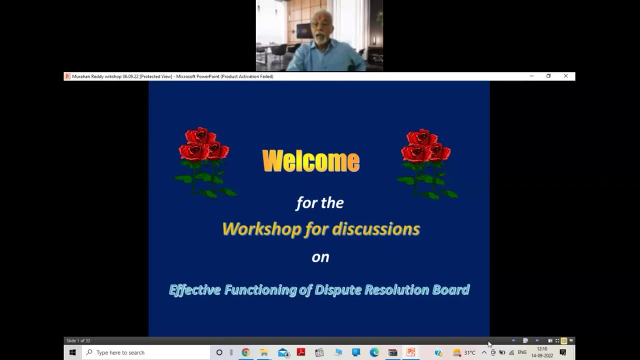 in fixing or upselling of the money among the three arbitrators actually, And there was no clear discussion of the fee grant to all. theako- Earlier he said that we need 10 и0, 2000,000 rupees per arbitrator for tenía. 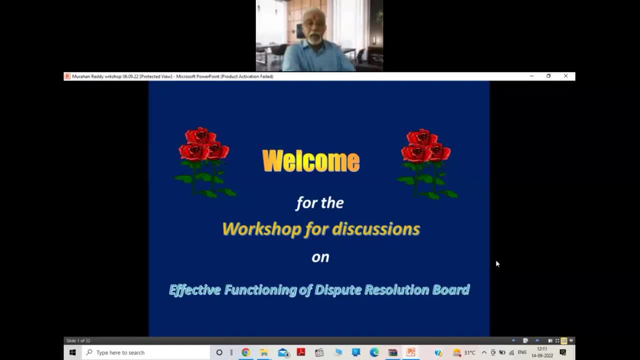 lol Here. there was a next process, namely the fee payment. So further says that in the event the arbitral tribunal is a sole arbitrator, he shall be entitled to an additional amount of 25 percent of the fee payable, as per table set above. 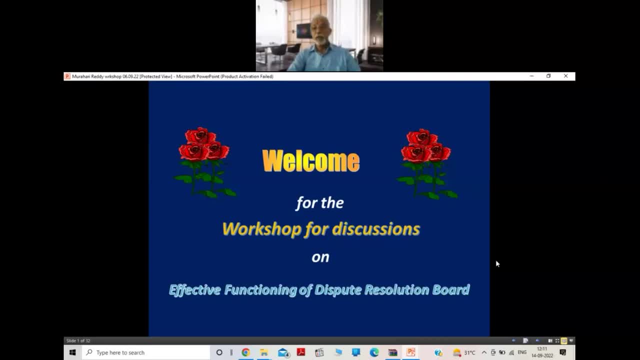 Now what some of the tribunals have done earlier and that if an arbitral arbitration case, the claimant has submitted their claim, the respondent has also submitted their counterclaim. So they have concede they are considering the two different arbitration in one arbitration by saying that the claim amount is one set of arbitration. 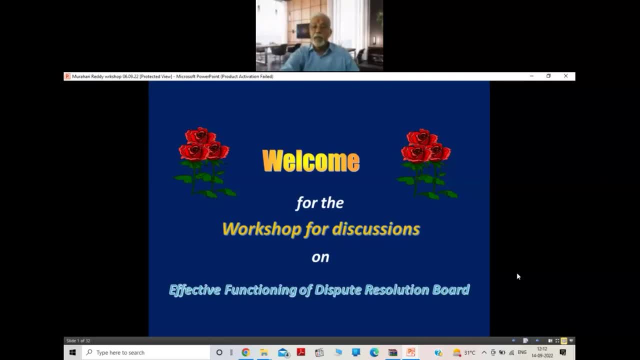 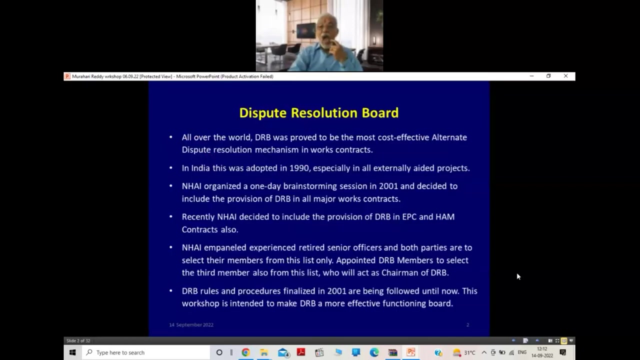 and counterclaim is another set of arbitration and they are charging double the fee in one single arbitral arbitration process For one arbitration case. So this was the judgment of the Delhi High Court of 15-05-2018.. It was decided that, for the purpose of computing fee of the arbitral tribunal, the sum in dispute 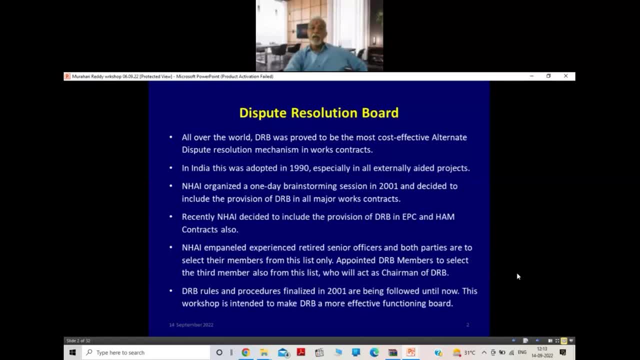 shall be the total sum of both claim and counterclaim Before arbitral tribunal. So this was decided that the claim amount includes the claim as well as the counterclaim for this computing or deciding the fee of the arbitral tribunal in particular case. So this judgment has: 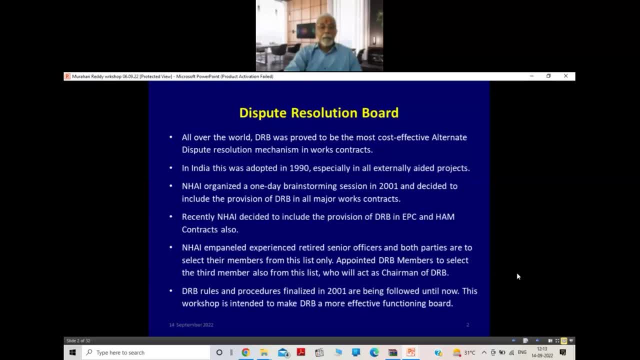 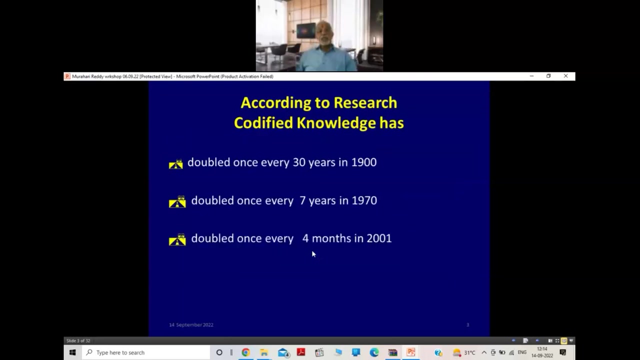 Further Clarified The Fee: How to calculate the fee of arbitrators. Now, judgment of 10-07-2019 of Supreme Court in case of NHAI versus Gayatri Jhansi Roadways Limited. It was decided that whether: 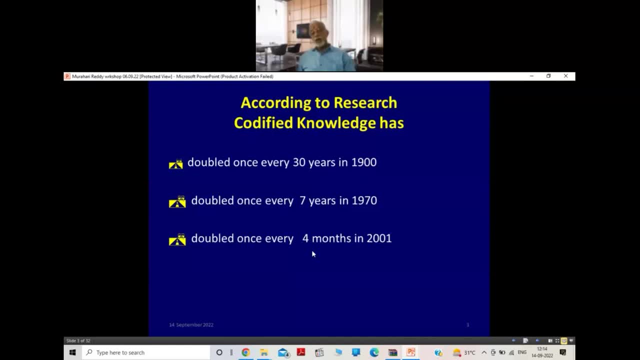 Terms are laid down as To arbitrators fee in the agreement or the supplementary agreement between the parties need to be followed. In some of the cases It was found that the A supplementary agreement was entered between NHAI and the concessionaire or the contractor. 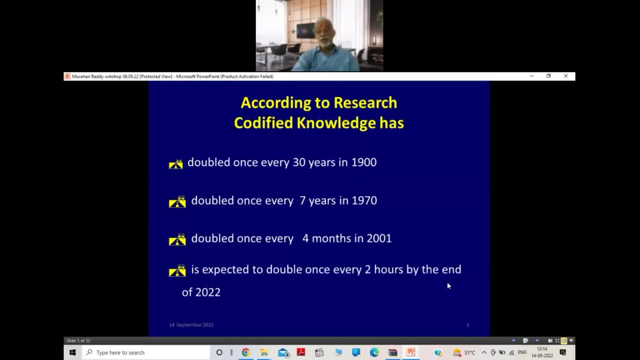 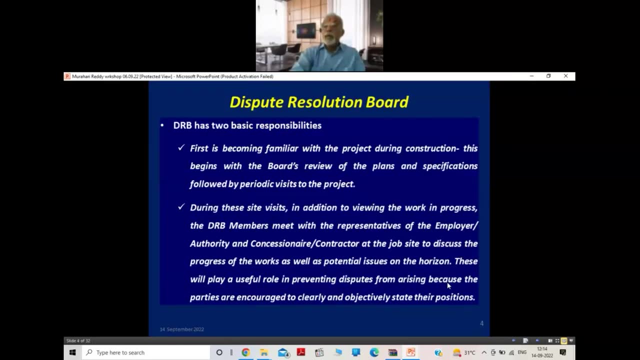 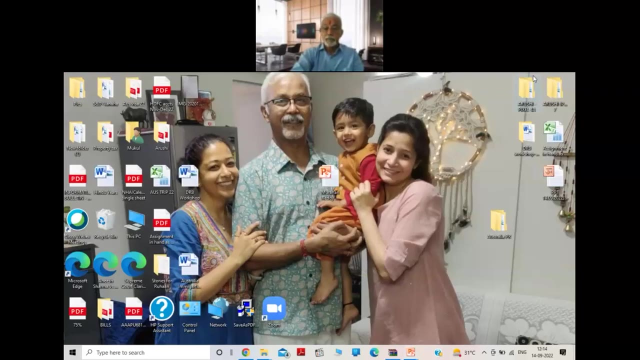 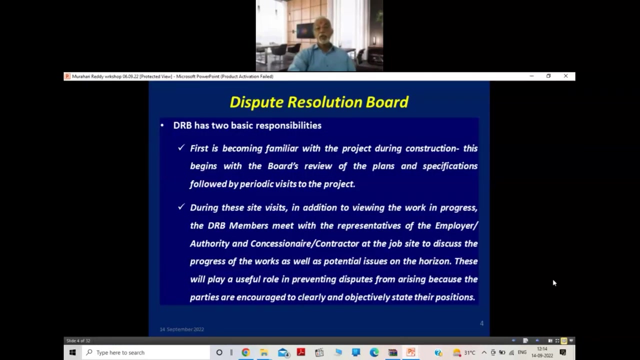 Prior, Prior to initiate The arbitral arbitration And And the once the arbitrators are appointed, They Have Or they have been informed At the time of appointment that This is the supplementary agreement and, according to supplementary agreement, These 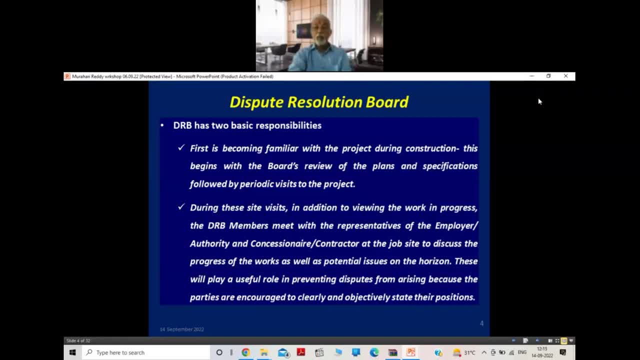 Fee will be applicable. Nobody Used to object Initially. Well, After Constitution of The Arbitral Tribunal, They, Some of The Tribunal, Used to say that We will not accept, We will not Bound by your supplementary. 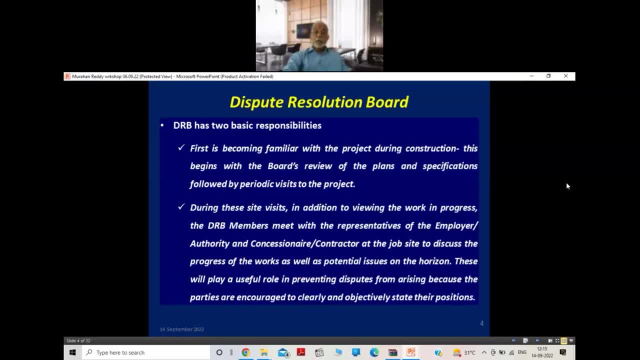 Agreement or Agreement, We will fix our Fee Of Our Own. And then- So this was challenged by us. Finally, The Supreme Court has Decided that If, If The Fee Schedule 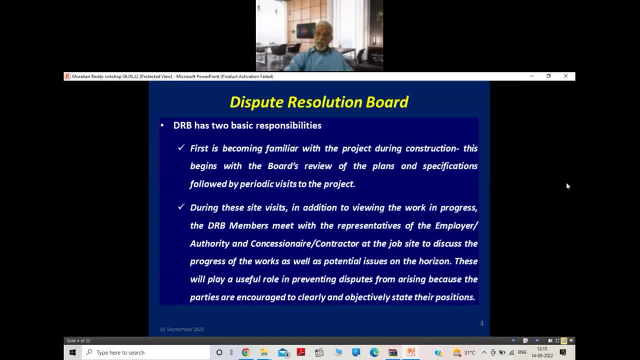 Has Already Been Provided In The Agreement- Main Agreement- Or In The Supplementary Agreement That Needs To Be Followed By The Supreme Court. The Issue: 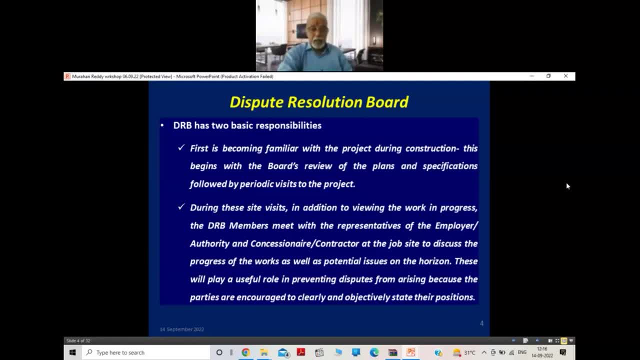 Of Fee Of Arbitrators Mentioned Above Is Payable To Each Arbitrator Or To The Pay? T Is Not Decided, But Recently Supreme. 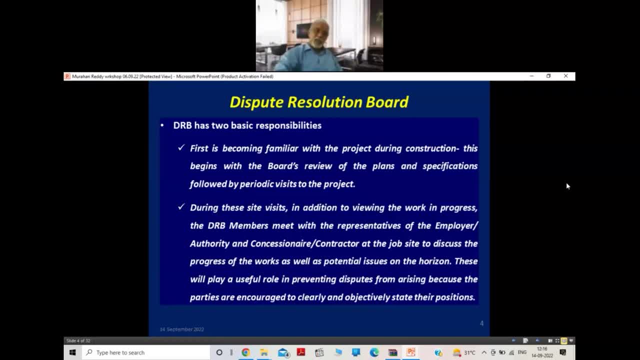 Court By Their Decision In Case Of O N G C V S F Com, The, They Have Decided Certain Issues, Number One That This 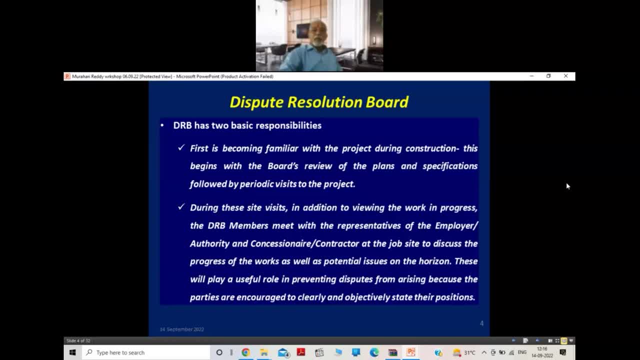 30. Lakh Fee Is Payable To The Arbitrator Is Payable To Each Arbitrator. About One Interesting Point In Between I Forgot To. 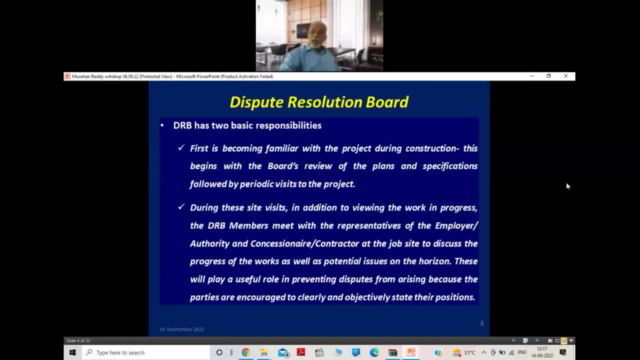 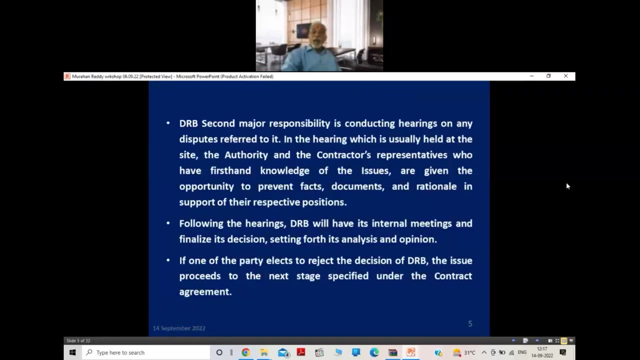 Tell Everyone If You Are There. Some Of The Tribunal Have Interpret It: The, The Is A Amount To That X, To Some Extent That. 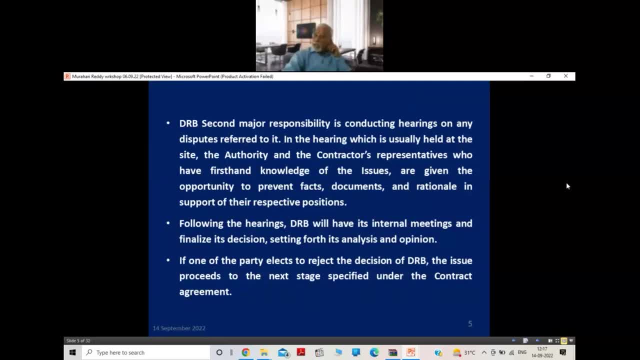 The Total Amount Comes To Forty Nine Less Eighty Seven Thous. What They Say Is. What They Say Is The Provision Is If The Sum 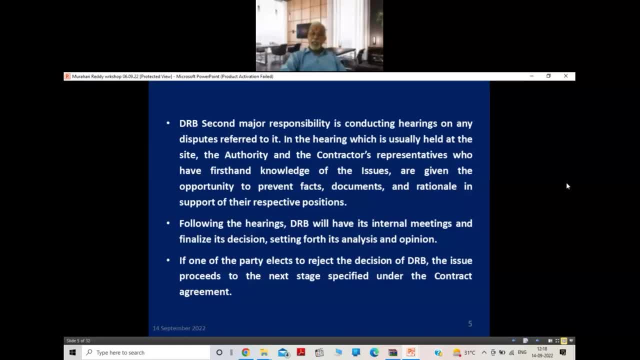 Of Dispute Is Above: Rupees Twenty Lakhs Twenty Crores, Then Rupees Nineteen Lakhs Eighty Seven Thous Plus. Point Five Is To: 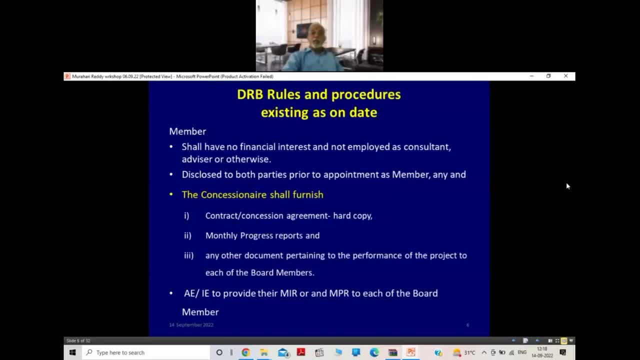 Pay That The Nineteen Lakhs. Eighty Seven Thous Is The Amount Payable Till Twenty Crores Of Amount Of Dispute, Subsequently Or: 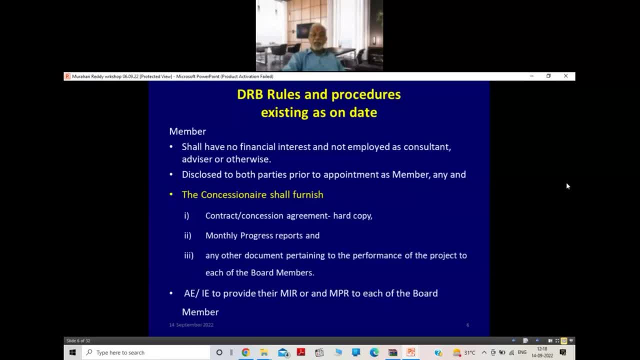 The Subsequent Claims Say The Claim Amount. They Say That Up To Twenty Crores The Amount Of Fees, Nineteen Lakhs Eighty Seven Thous. 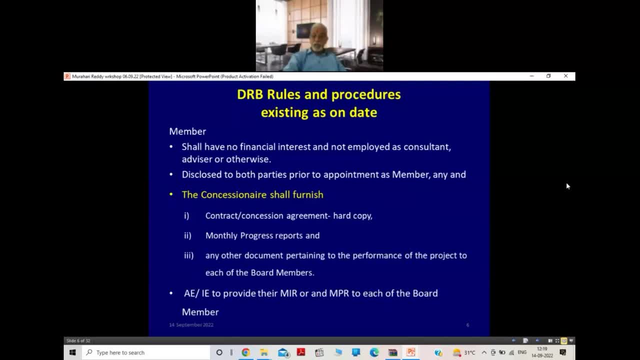 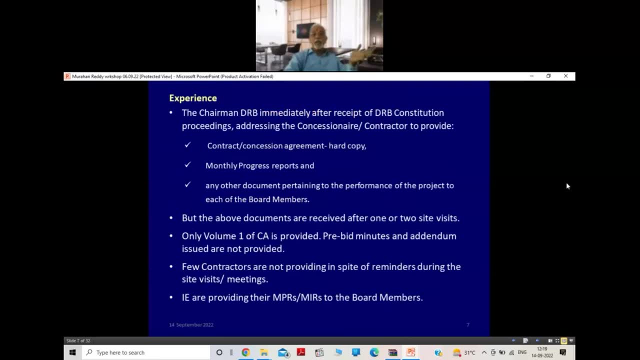 And Over And Above That, The Ceiling Is Thirty, Thirty Lakhs, So Thirty Lakhs, And They Have Forced Parties To Pay According To This Principle. 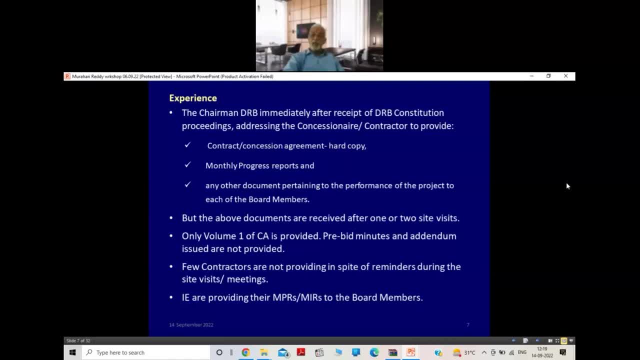 Forty Nineteen Now, As Per The New Judgment Of Thirtieth August, Twenty Twenty Two Between This Case Is Sealing Is Thirty Lakhs. 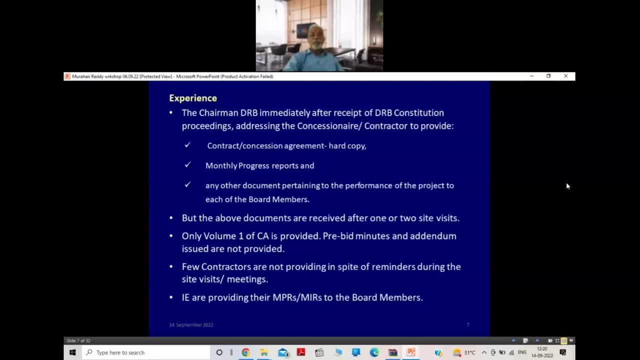 Irrespective Of The Amount About Twenty Crores, Not Forty Nine Lakhs Or Eighty Seven, Eighty Seven Thous, And Amount Of Money Paid. 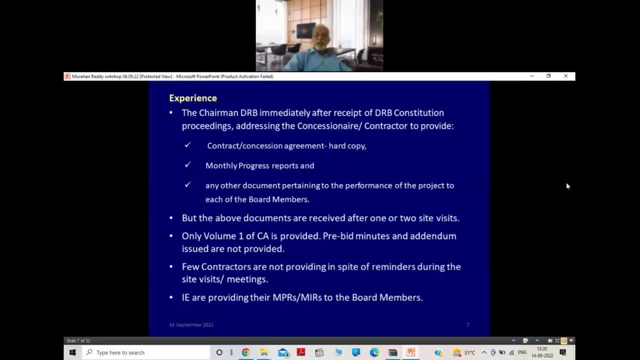 To The Arbitrator Will Be Thirty Lakhs Only, And That To Sorry, Sir Fine, Fine, Sir Fine, Sir. No, No Issue, No Issue, Thank. 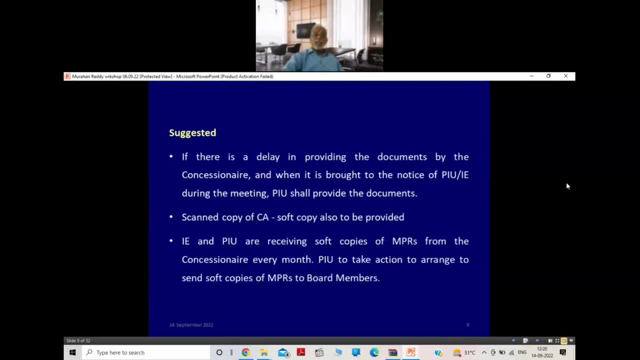 You, Thank You Now, Welcome Back. So We Were Talking About The Pre Schedule As Far As The Fourth Schedule Of Education Consideration At This. 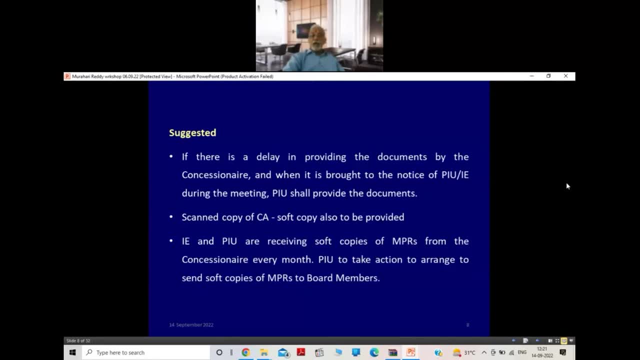 Consent, And I Was Talking About A Recent Judgment Of The Pre Schedule For 2022.. In The Matter Of When GC Was F Cons, 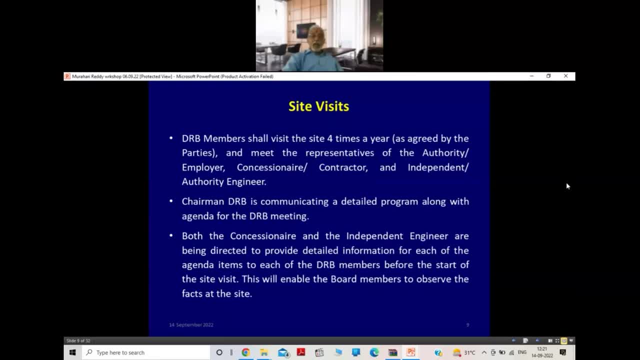 Wherein It Was Decided That The Maximum Limit Of Arbitral Arbitration Fees 30. Lacs. Was Also Decided That The Sum In Dispute 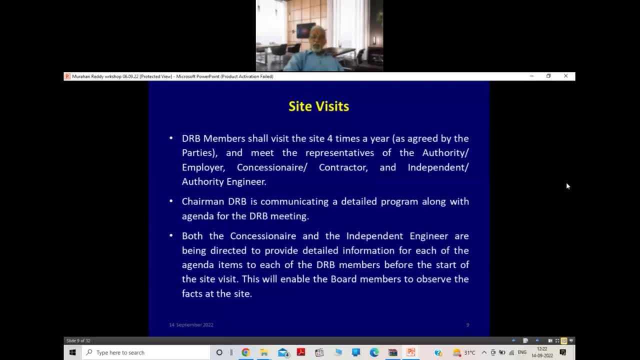 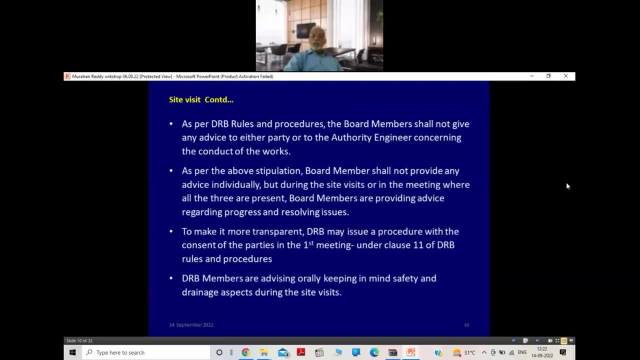 Shall Be The Total Sum Of Both Claims And Counter Claims, And The Decision Was Decided That The Sum In Dispute Shall Be The Total. 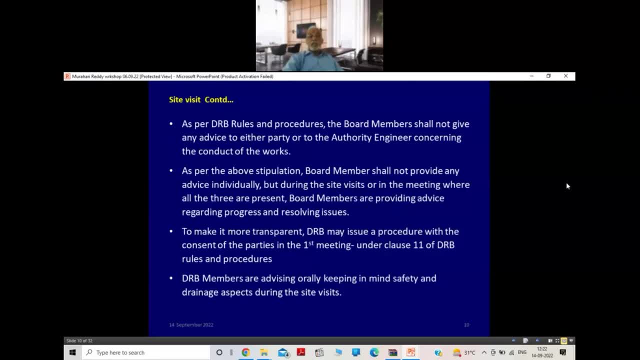 Limit Of Arbitration And, In Dispute, The Sum Of The Sum Of The Cons, That Decision Was Decided. That Was Decided That The Cons 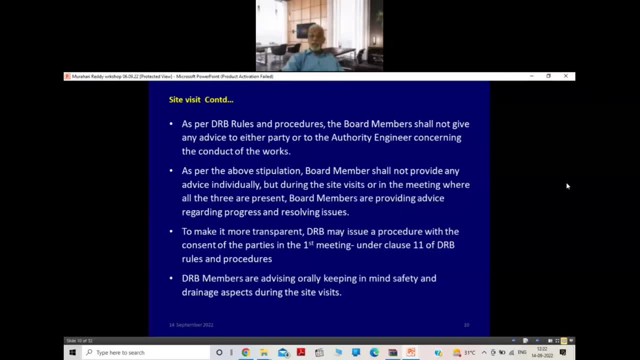 Was Decided That The Sum They have reverted back into what exactly the earlier arbitrators were asking for, which was clubbed together by Delhi High Court in their judgment of May 2018, that some of both claim and contract claim will be considered for the purpose of computing the fee. 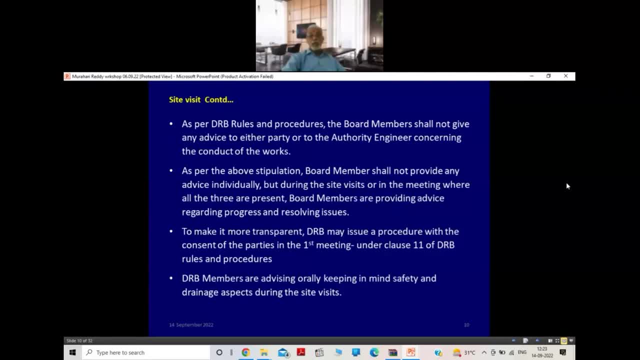 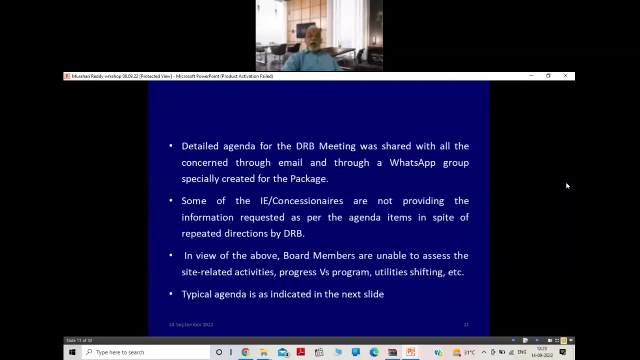 Now they have segregated that the claims are, the fee for the claims are different and the contract claim fee will be separate. Now some more features about the Amendment of Arbitration Act 2019.. That the SOC and SOD under Section 23,. 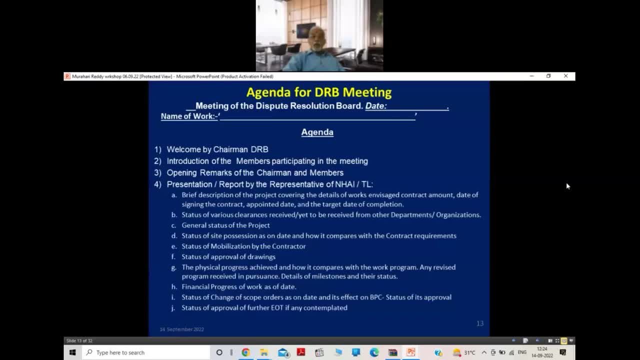 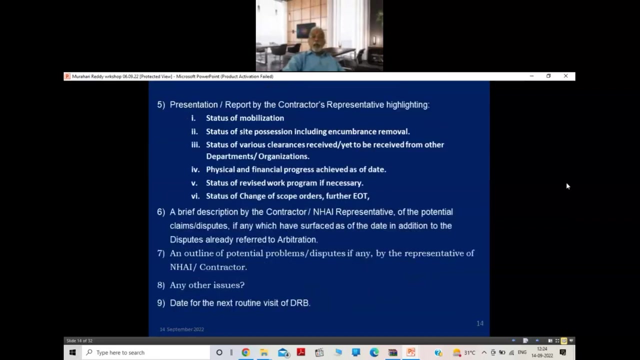 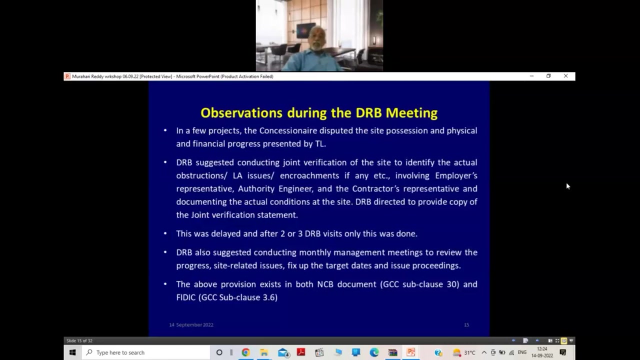 of Principle Act shall be completed within a period of six months Earlier if you go through with the earlier slide, wherein it is said that the limit for publishing award- orbital award- has been set to 12 months from the being considered. This 12 months includes submission of the pleadings, SOC, SOD and rejoinder. 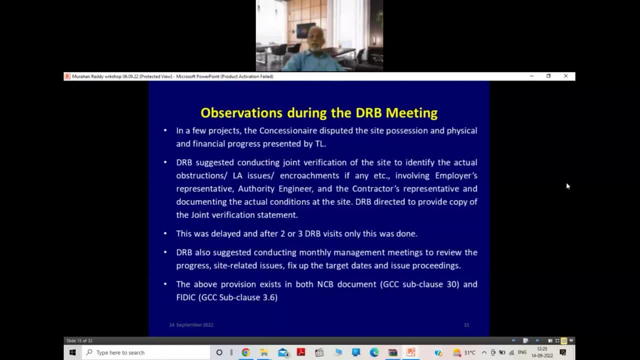 So it was found that parties take approximately four to six months or submission of their pleadings. Then half of the time of this 12 months is wasted on the submission of the pleadings for the arbitral tribunal to decide their issues. so it was. 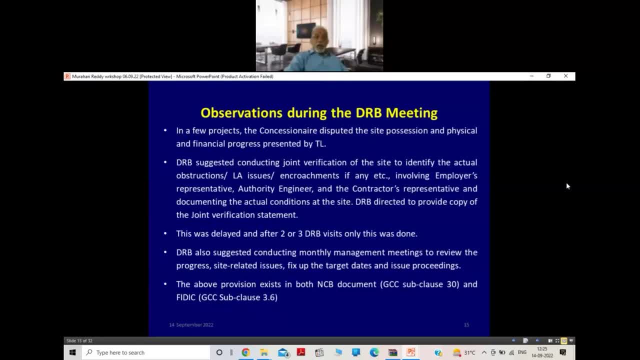 in 2019. it was decided that the submission of completion of pleadings- the time period is given as 6 months- then, after completion of this, all the pleadings 6 months time, the 12 month time will stop. section 29 A1 clarifies that the 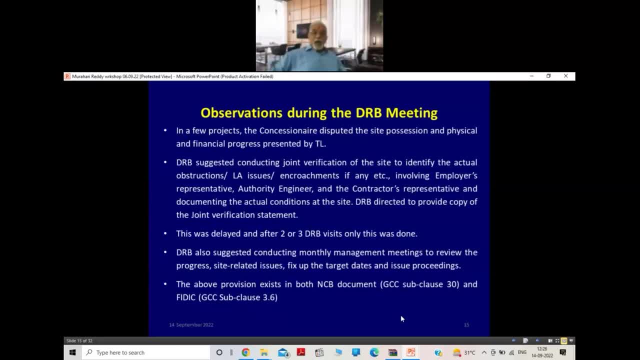 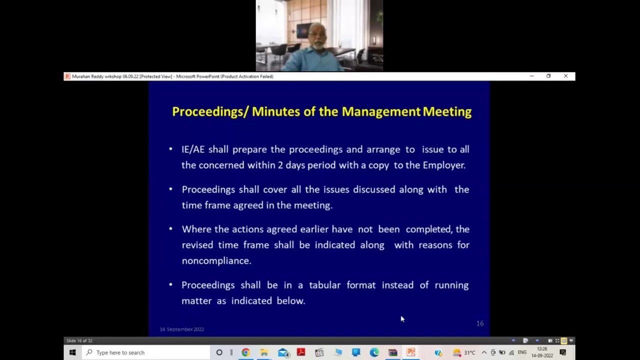 award other than international commercial arbitration shall be made by the AT within a 12 month time from the date of completion of pleadings, as mentioned above. now the 8th schedule was introduced and qualification experience of arbitrators. so that includes if an advocate within the 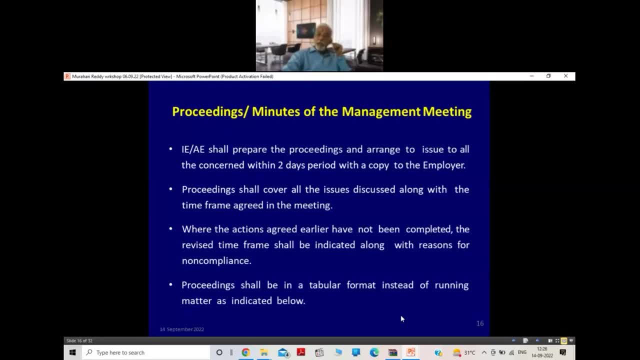 meaning of advocate: 1961 having 10 years of practice experience as an advocate is eligible to become an arbitrator. similarly, charters accountants with 10 years of experience, Post accountant having 10 years of experience, CSF companies actually having ten years of experience. 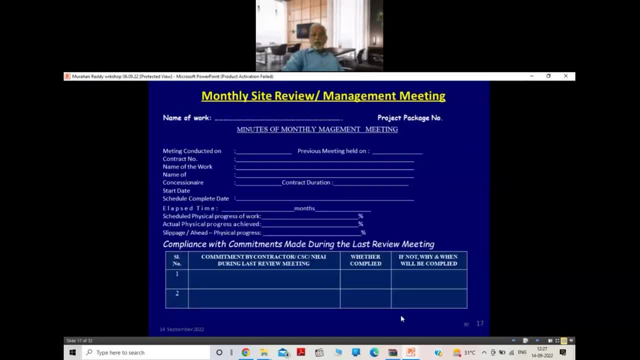 are eligible to become an arbitrir. an officer of Indian legal service and wife should be known as an 320 sabes. An officer with a law degree having 10 years of experience in legal matters in the government, autonomous body, public sector undertaking and senior level managerial position in private sector are also eligible. 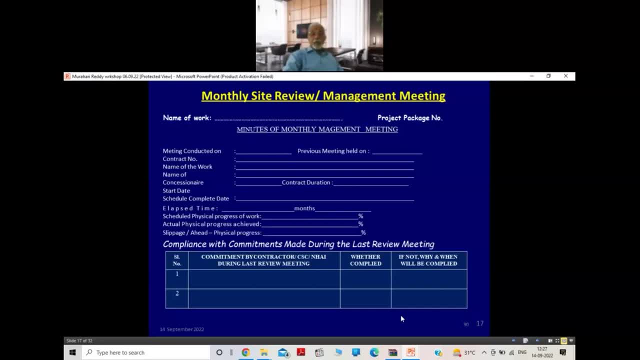 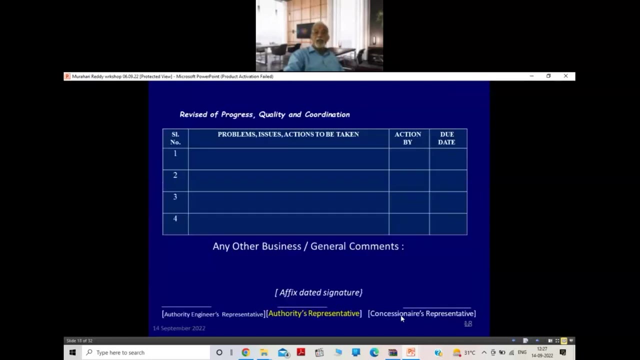 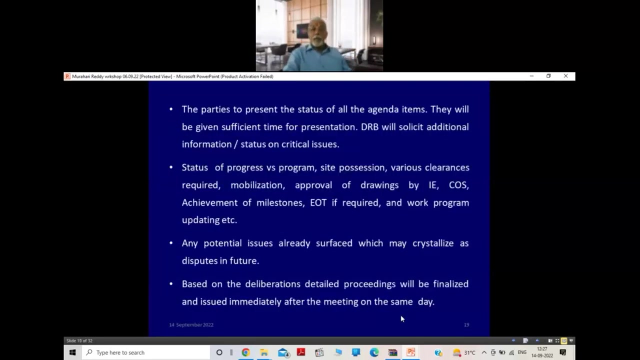 An officer with an engineering degree having 10 years of experience as an engineer in the government autonomous body is also entitled to become an arbitrator. An officer of senior level experience of administration, IAS, etc. They are talking about, So they are also eligible. 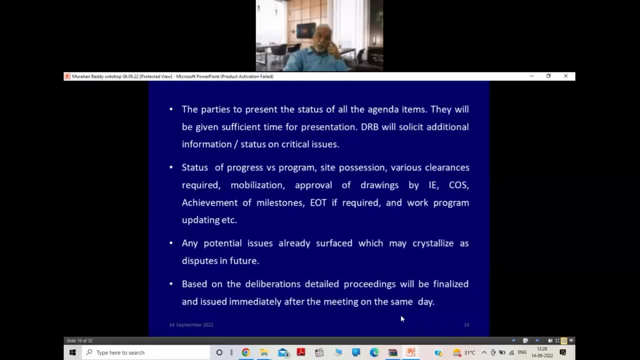 It is a person in any other case having educational qualification at degree level with 10 years of experience, scientific or technical stream in the fields of telecom and IT, intellectual property rights, etc. In government, The most body of public sector at a senior level, can also become arbitrator. 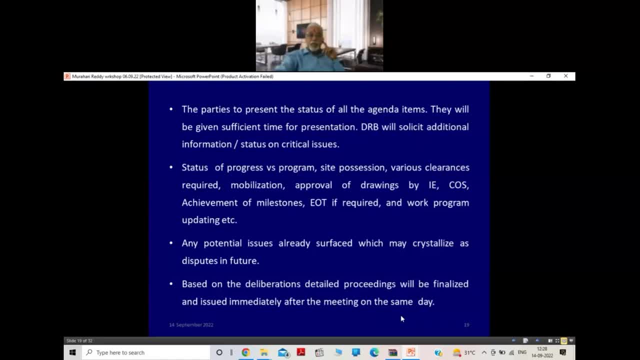 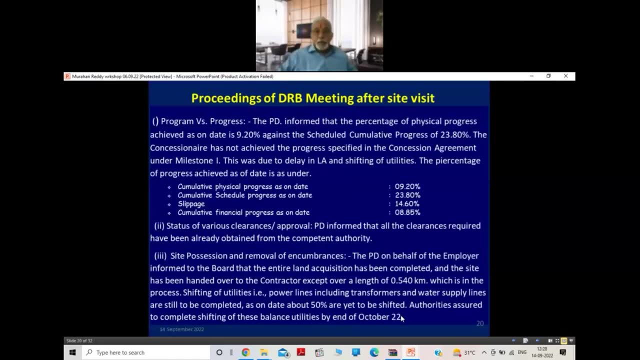 So This is What is. I have prepared a presentation for all of you Now For Now, the further I would like To ask your queries: clarification on any of the issues of the on my presentation or otherwise, also relating to any issue like mediation or DRB, arbitration or conciliation. 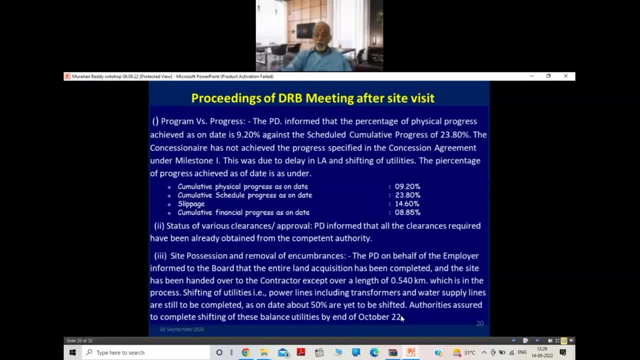 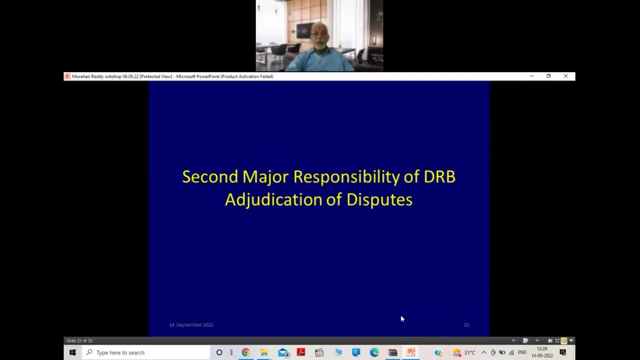 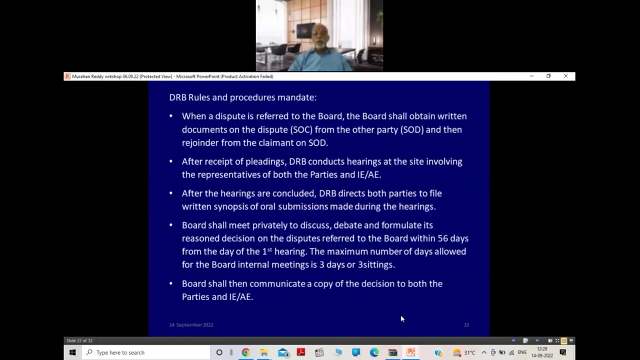 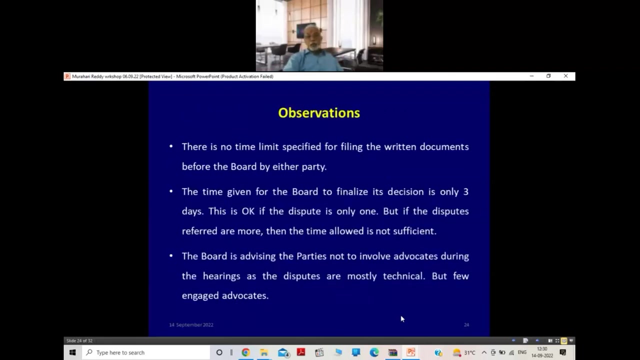 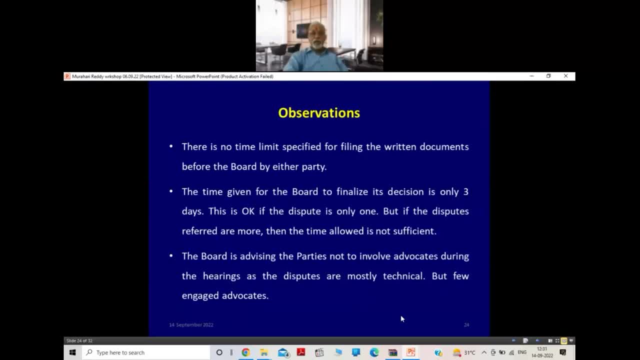 Yes, sir, Nobody is interested to raise any question. Recently, on 6th of September, Nila ji, can I share some other PPT? We have conducted a workshop recently, on 6th, on the functioning of ERB. Yes, you can share, sir. 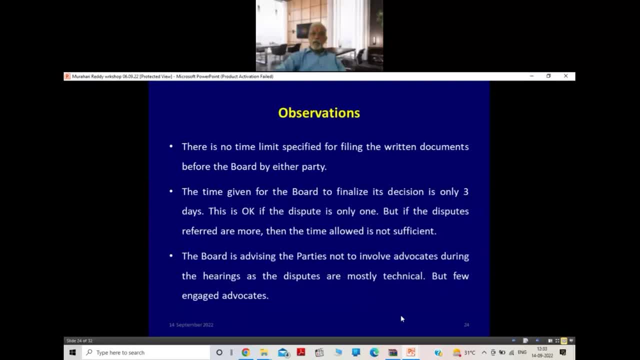 Mr Murahari Reddy, who is the Senior Chief Retired of PWD Andhra. he had a presentation. Can I share that? Yes sir, Yes sir, Share sir. So I think nobody had a query, I think. 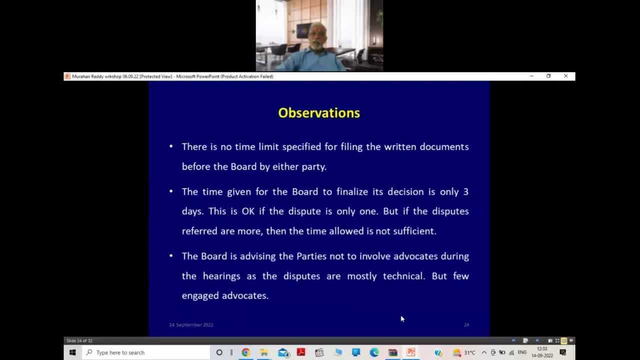 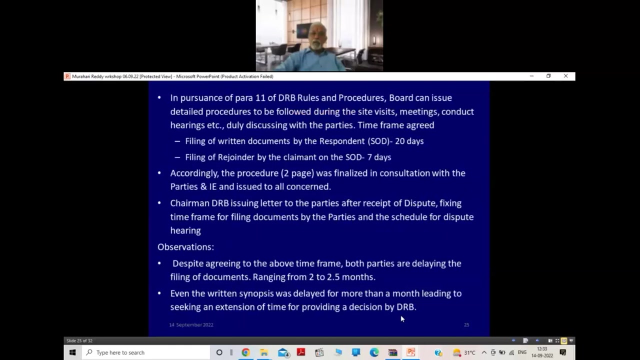 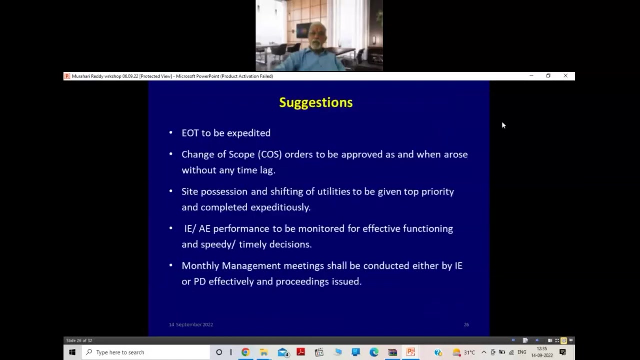 So nobody is asking for, So let me, Okay, Okay, How can you Let me do? take out that first. Okay, you, you, you. I think it is not with me presently, we are. I think it is not with me presently, we are. 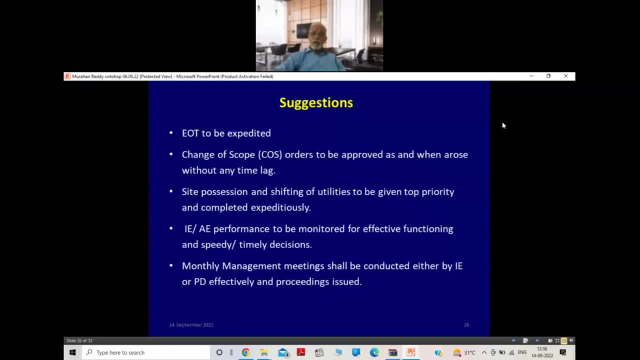 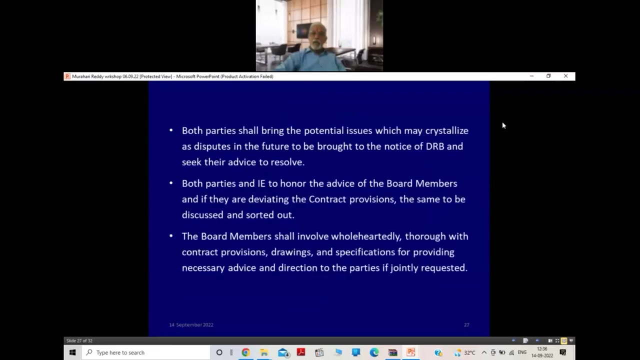 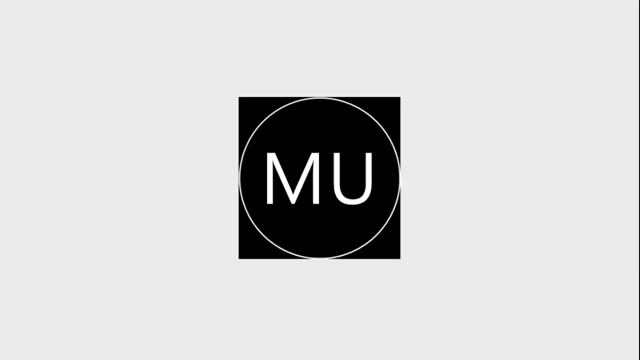 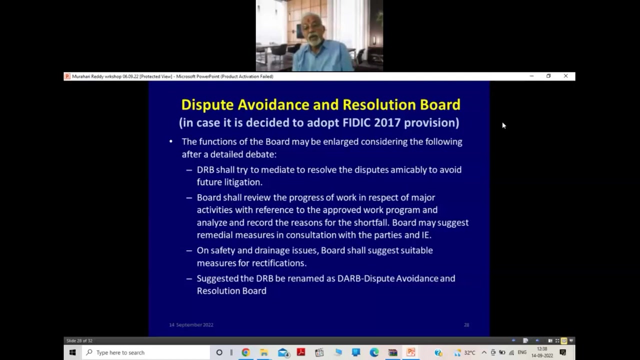 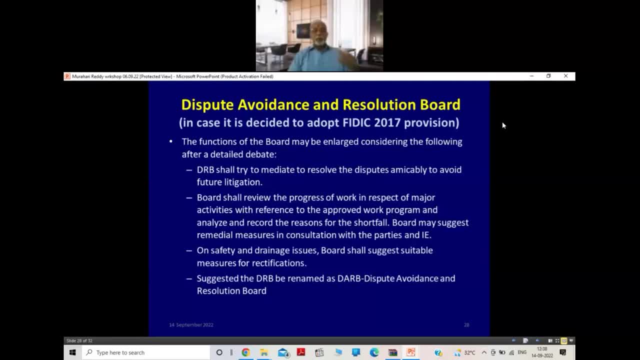 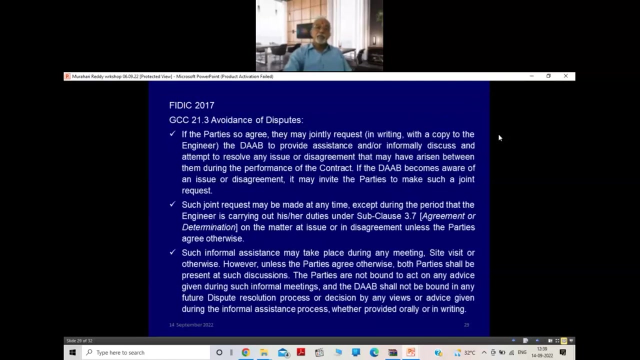 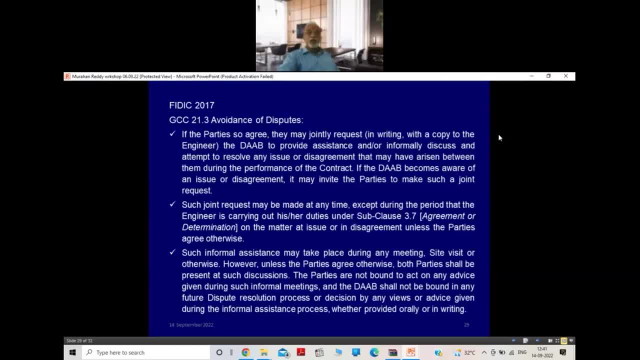 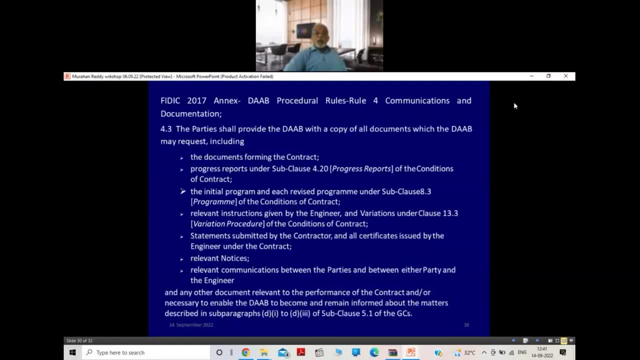 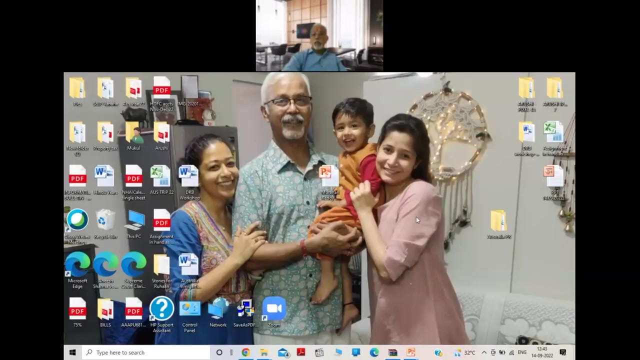 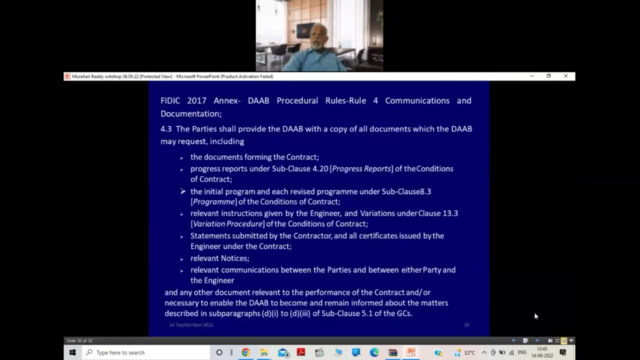 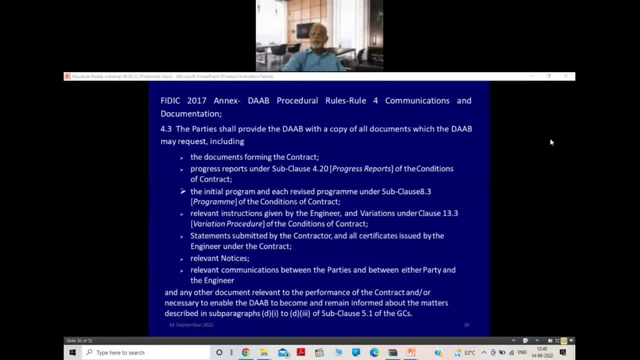 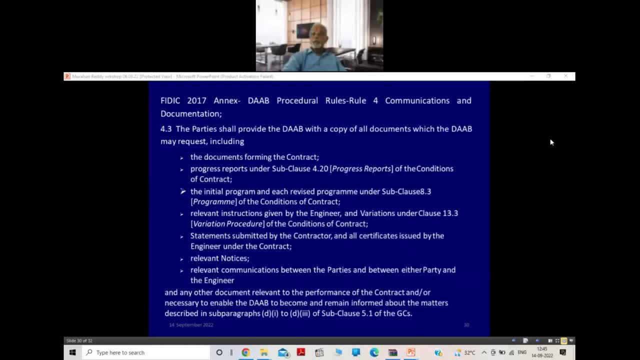 the world back funded or adb funded or the jvic funded projects and they also have started uh adopting this drb uh since uh 99 or 2000 onwards. all uh externally aided projects, initially uh and which i am panel, experienced and retired senior officials, and both parties are to select one. the rules and procedure finalized in 2000 are being followed. 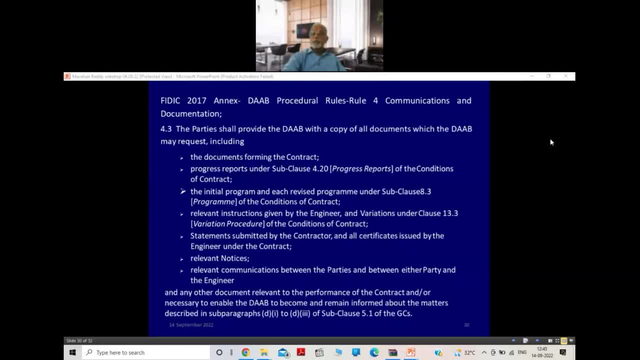 until now, the, according to research, modified knowledge has doubled. this is what his uh observation: a world once in every 30 years. in 19, then in 1970 it used to be doubled once every seven years, and then 2001, it doubled once every four months in 2012. 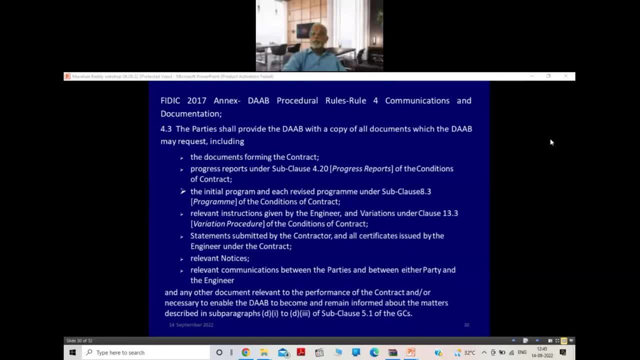 it is expected to double once every two hours by the end of 2022.. The basic responsibility of the DRB is to become familiar with the project during construction, and this begins the Board s review on the plans and specification, followed by periodic visits to the projects. 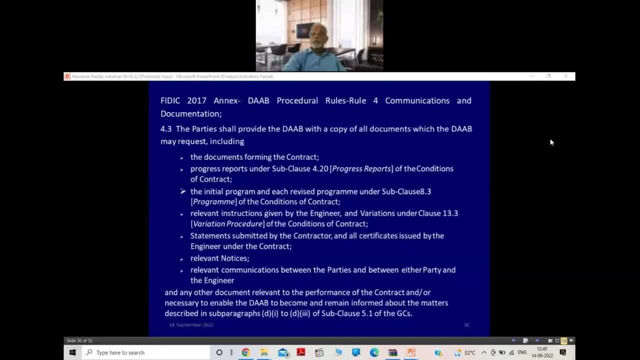 So, as far as our rules and procedures are concerned, we have mentioned in our rules recently, which has been modified Earlier. the rule says that the DRB has to visit site six times in a year, 12 months And also by mutual reference. 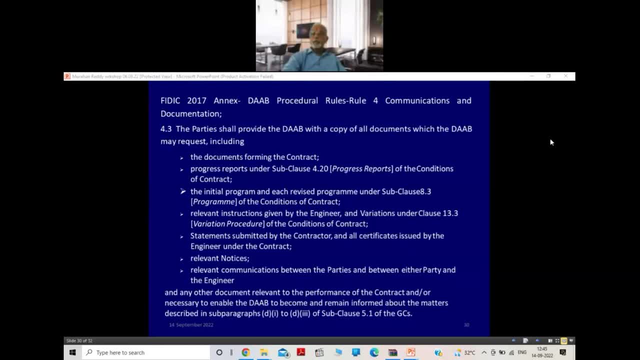 Anduce request made by NHI for the concession that six visits a year can further be extended. It depends on the important events of construction, if any is going on in the project. Subsequently, it was found that It was found that the six visits seems to be slightly higher. 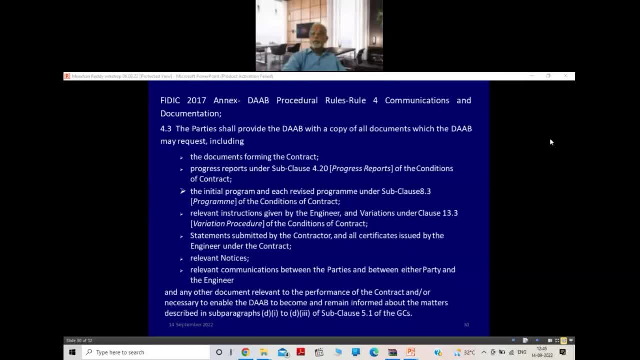 on the project. So it has been now reduced to 4 visits in 12 months, plus the additional with the request of the parties Doing these site visits. in addition to viewing the work in progress, the DRB members meet with the representatives of employer authority and the concessionaire at the job site to 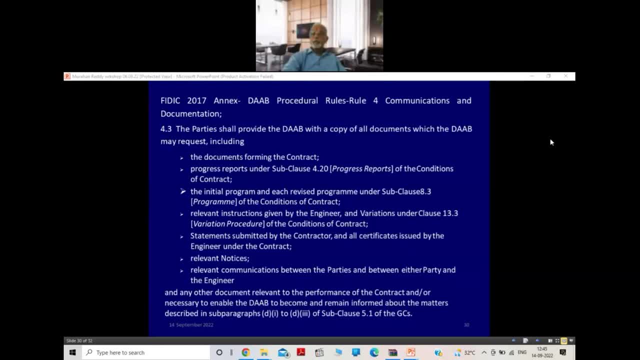 discuss the progress of works as well as potential issues on the origin. These will play a useful role in preventing disputes from arising, because the parties are encouraged to clearly and objectively state their position. 2. SECOND, MAJOR RESPONSIBILITY: conduct a hearing on any disputes referred to it In the hearing, which is usually held at the side. 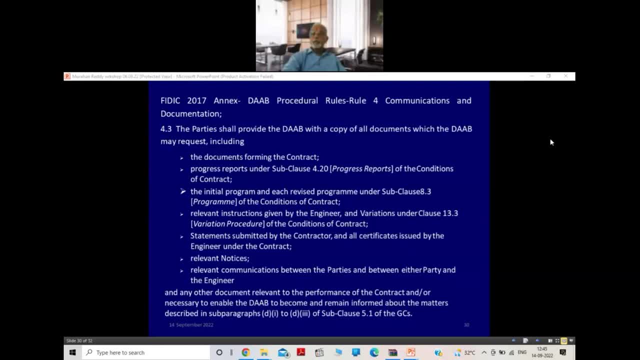 the authority and contractors. representatives who have first-hand knowledge of the issues are given the opportunity to prevent facts, documents and rationale in support of their respective positions. Following the hearings, DRB will have its internal meetings and finalise its decisions setting forth its analysis and opinion If one of the parties elects to reject the decision. 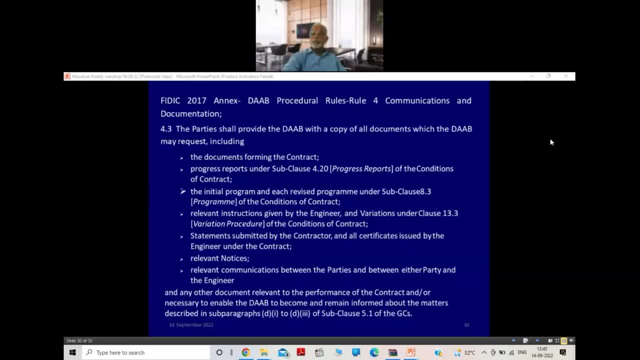 of DRB, the issue will proceed to the next stage specified under the contract agreement. In our contractual agreement, it is specified that the issues conferred that this issue can further be referred to for the next stage. For the next stage, it is specified that the issues that were talked about can be reversed. 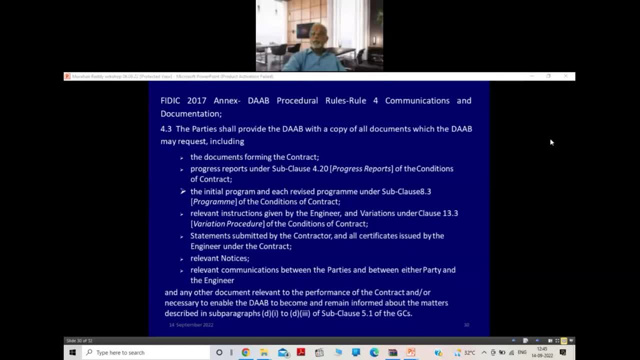 consideration through CCIE, Now BRB, rules and procedure. as on date, the member shall have no financial interest and not employed as consultant, advisor or otherwise. Member should disclose to both parties prior to appointment as member. any the concessioner shall furnish contract or concession agreement or copy, as well as the soft copy monthly. 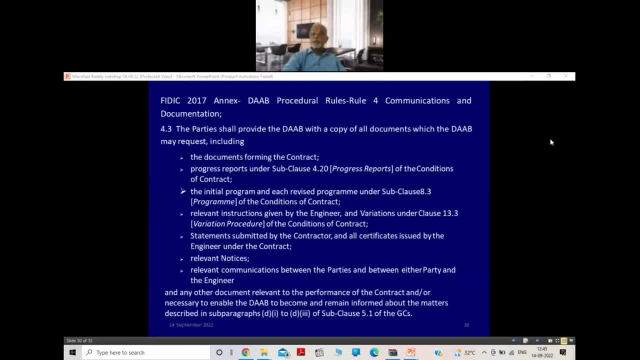 progress report and any other documents pertaining to the performance of the project, with each of the board members AE IE to provide their MPRs MIR to each of the board members. He had an experience that the chairman DRB, immediately after the seat of DRB constitutional proceedings, addressing 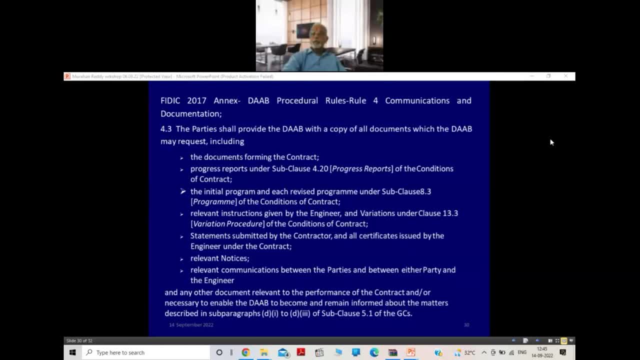 the concessionaire to provide certain documents mentioned here. The above documents are received after what was his views after one or two site visits. So their experience is that, even after requesting the parties before the site visit, just after the constitution of the DRB. 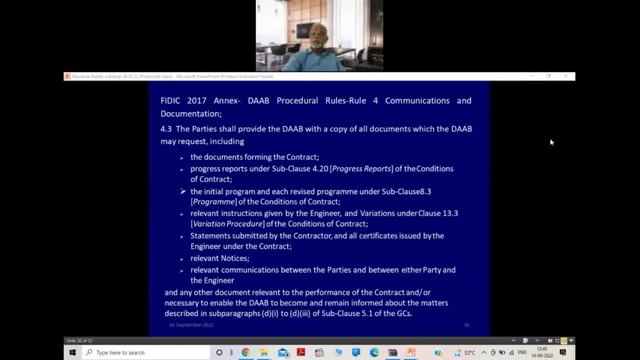 certain documents needs to be sent to them, but these are not being provided until unless for one or two site hearings or site visits are made by the DRB. So this is what they are requesting: that the documents are to be supplied just after the constitution of the DRB to all the members. 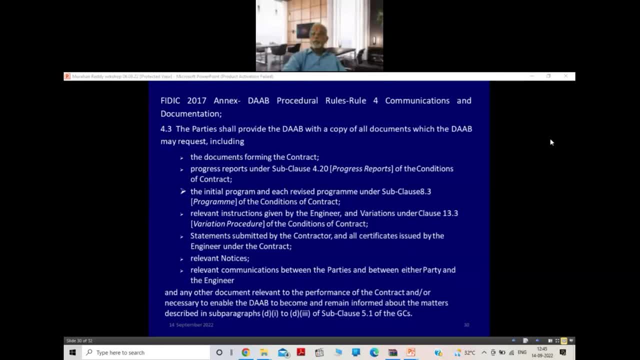 Only Volume 1 of CA is provided. Preview minutes and amendments issued are not provided. Contractors are not providing, in spite of reminders. AEE are providing MPRs to the board. What he has suggested is, if there is a requirement, then the board of the department will provide documents to a specific department. 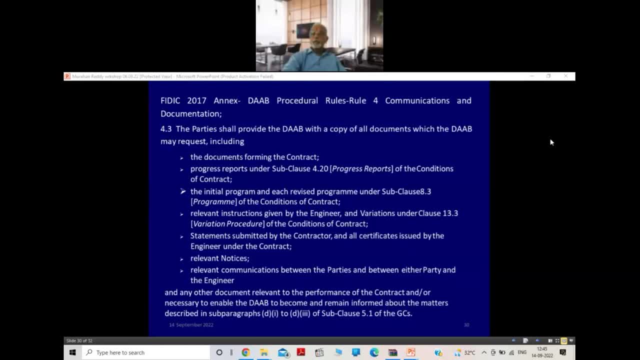 is a delay in providing the documents by the concessionary, and when it is brought to the notice of piu during the meeting, piu shall provide the documents in case. if the concessional contractor is failed to do so in time, then the nhl should provide these documents. this is what he has. 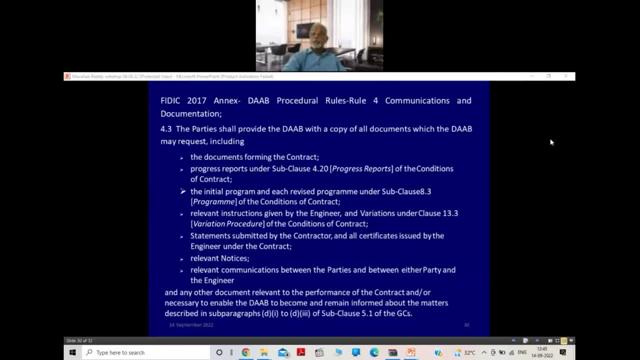 suggested this. can copy of uh contract agreement constitution also be provided? ie and pius are receiving soft copies of mprs from the concessional agreement. piu will take action to arrange to send this soft copy of mprs to the board members site visits. drb shall visit the site four times in a year and meet the representatives. 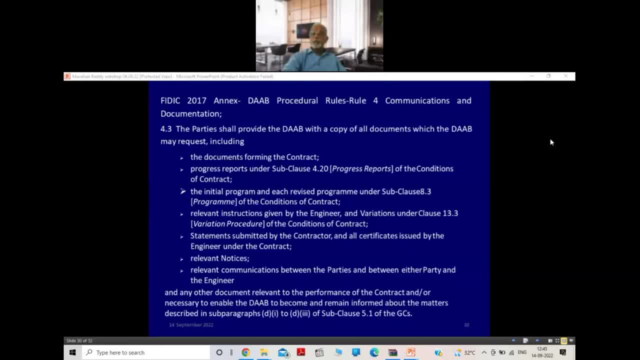 chairman drb is communicating a detailed program along with the agenda for the drb meeting. both the concessionaire and the independent engineers are being directed to provide detailed information for each of the agenda items to each of the members before the start of site visit. this will enable the board members to observe the facts of the site as per drb rules procedure. 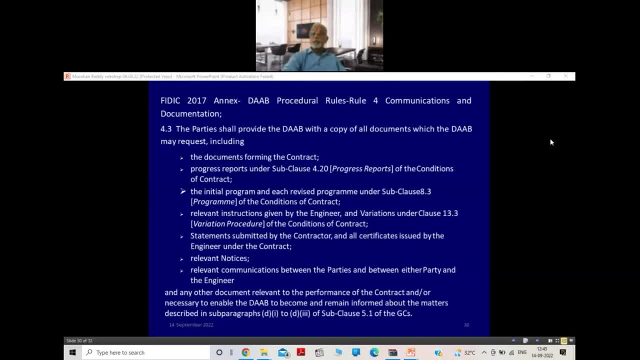 the drb members shall not give any advice to either party. this is very important. that says that drb members shall not give any advice to a party or the authority engineer concerned concerning the conduct of art. as per above stipulation, board members shall not provide any. 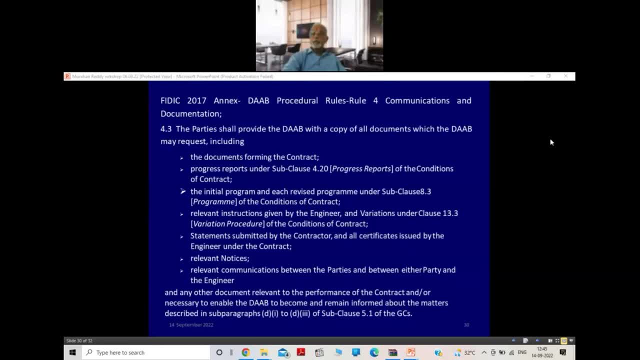 advice individually, individually to the parties, not to the authority- means nhl- not to the, the director of concession, not to the engineers, but during the site visit or in the meeting where all the three are presents. all the three means the different uh engineer, concessionaire and nhia representative- represent board members, are providing. 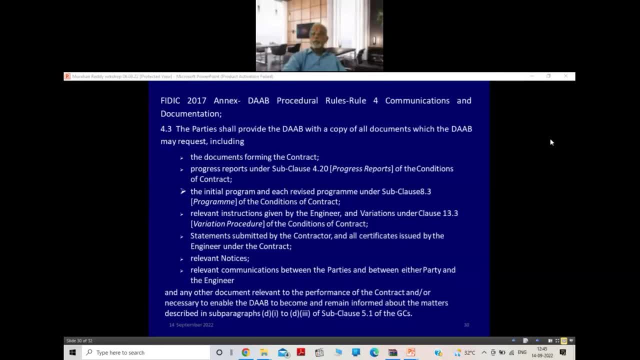 advice regarding progress and resolving issues, but they are not supposed to advise individually to any party. to make it more transparent, drb may issue a procedure with the consent of the parties and the first king of the clause so, and so the drb are as well advised. 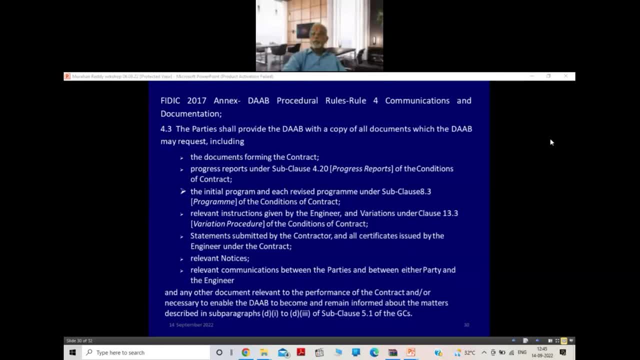 already keeping in mind safety and drainage aspects during the site visit. these are also very important uh points: the safety as well as the drainage. Detailed agenda for the DRV meeting was shared with all the concerned. Some of the are not providing the information requested in time. 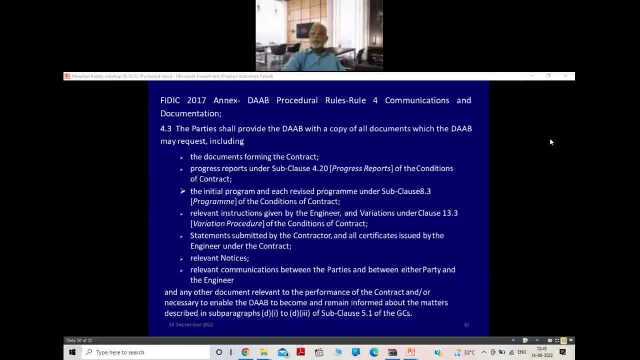 DRVs are unable to assess the site-related activities- program versus program, utility shifting, et cetera. So what he has followed, he has followed. wherever he is in the. he is the chairman of the DRV, he follows certain. 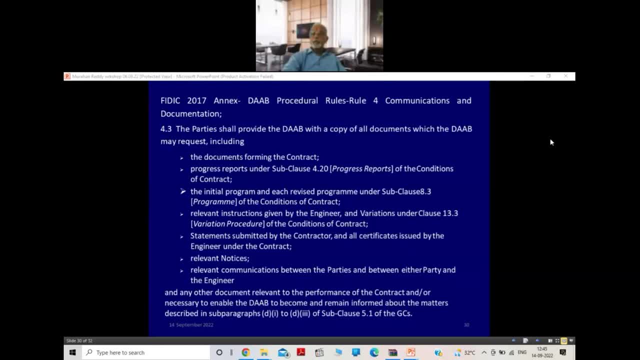 He has suggested that the template for the DRV meeting should be like this. Now he has observed certain issues regarding the DRV meeting. In a few projects, the concessioner disputed the site possession and the physical and financial progress conducted by the team leader. 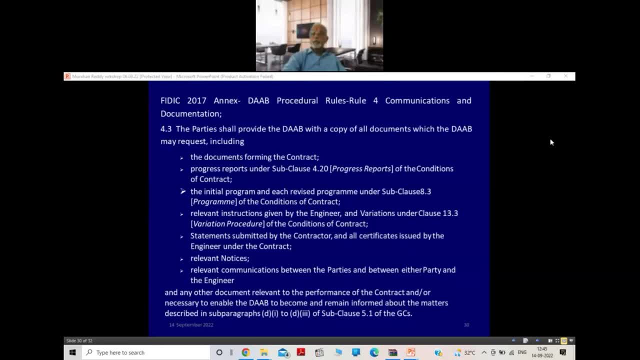 DRV suggested conducting joint verification of site to identify the actual obstruction and acquisition issues, encroachments etc. involving employer's representative authority, engineer and contractor representative, and documenting the actual condition at the site. So DRV directed to provide a copy of the joint verification statement. 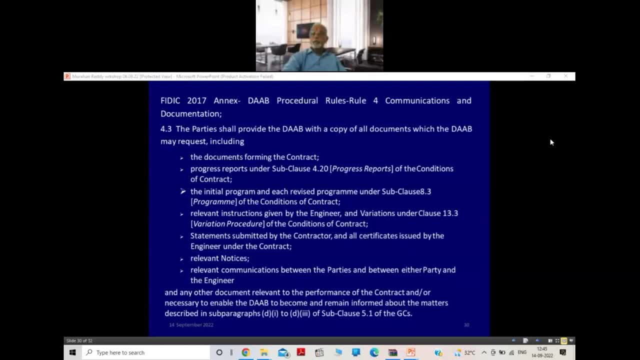 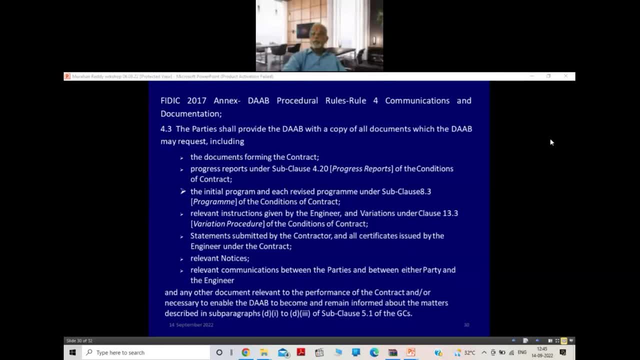 Proceedings- minutes of the management meeting. I shall prepare the proceedings and arrange to issue all consent within two days period, with a copy to the employer. Proceedings shall cover all the issues discussed, along with the time frame agreed in the meeting. where the action agreed earlier have not been completed, the revised time frame shall. 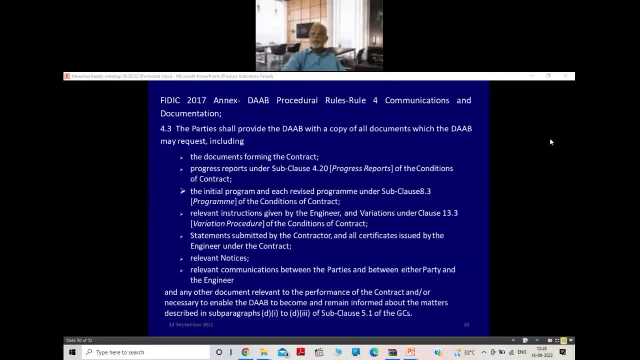 be indicated along with reasons for non-compliance, and the proceedings shall be in tabular format. instead of running matters, We have suggested one tabular form here of the action. The first tabular form is the date, contract number, name of work, name of concessionaire. 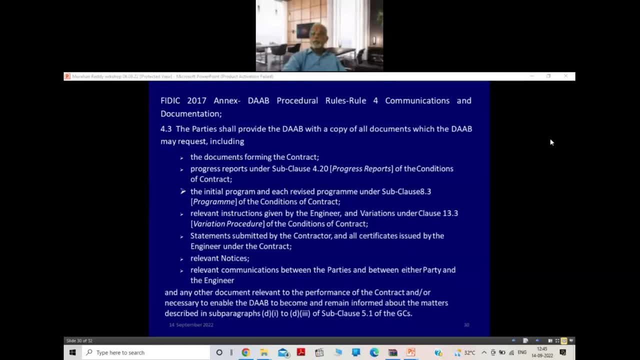 start date: contract duration schedule. completion date schedule. physical progress of work. actual physical progress of work. slippage or ahead of physical progress. The reason for this tabular form is that it should be in the date, contract number, name. 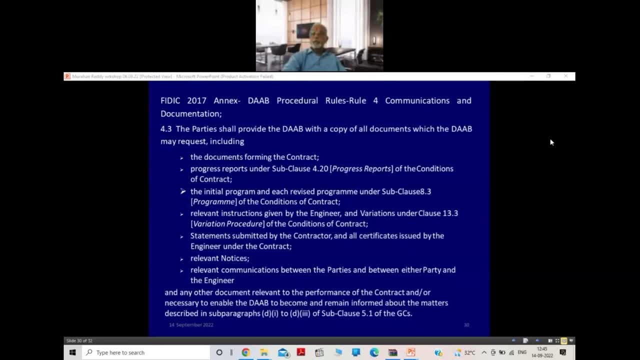 of work schedule. schedule of work schedule and the reason for that slippage or advancement. This is what we have suggested. The parties to present the status of all the agenda items will be given sufficient time for presentation. DRB will solicit additional information on critical issues. status of progress versus. 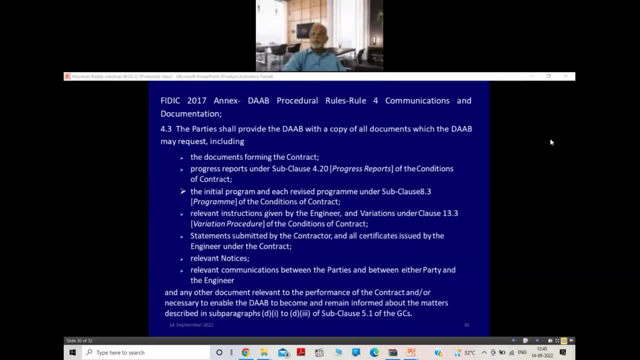 progress. various clearance required: legalization, approval of drawing by IE, COS, EOD, achievement of milestone, if required, the work program updates, etc. Any political issues already surfaced which may crystallize as dispute in future. based on the deliberation, detailed proceedings will be finalized and issued immediately after. 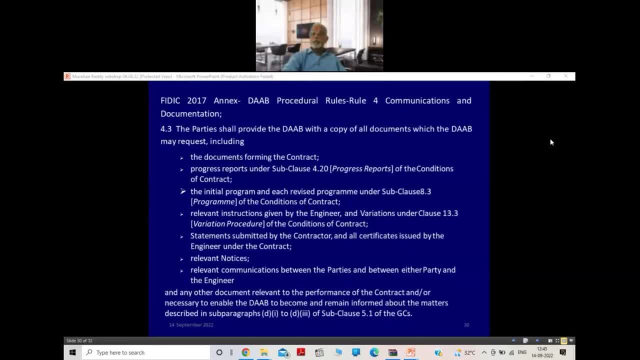 the meeting on the same day. Now proceedings of DRV meeting. after site visit: Program versus program: The PD informed that the percentage of physical progress achieved is 9.2% against the scheduled progress of 23.8%. The concessioner has not achieved the progress specified in the concession agreement on mild. 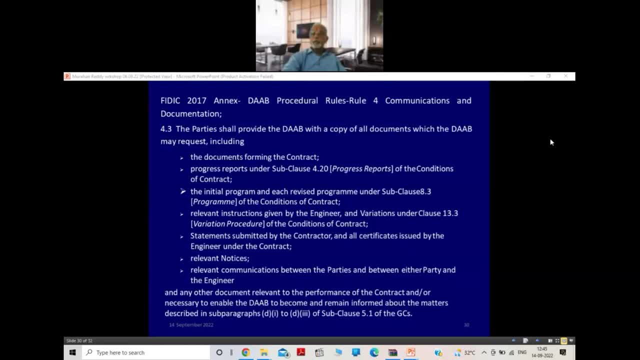 disorder One. this was due to delay in LA and shifting of utilities. The percentage of progress achieved as of date is: as of now. Such information needs to be provided in the proceedings of DRV meeting, DRV site visit and the meeting. The concessioner has not achieved the progress specified in the concession agreement on mild. 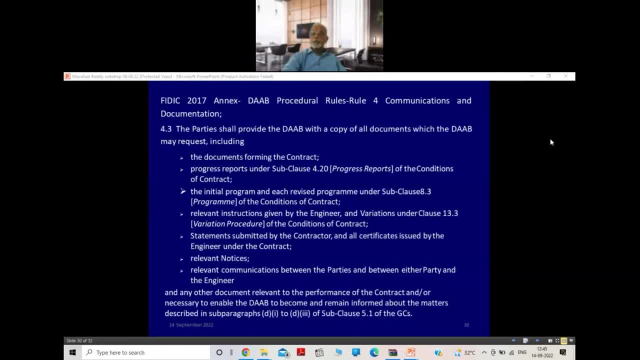 disorder. This we have already discussed after the hearing of our committee. DRV directs the party to file a written synopsis. Board shall meet privately to discuss. The maximum number of days allowed for the board internal meeting is 3 days or 3 sittings. 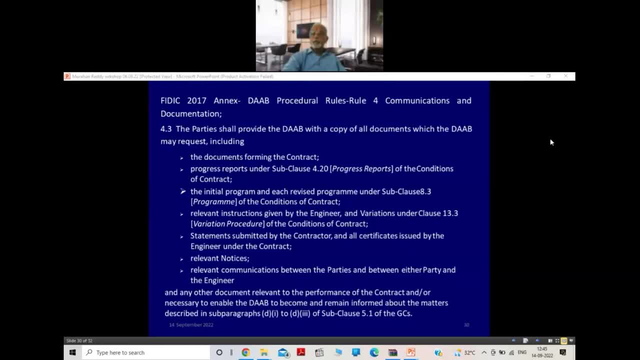 This is what we have provided in our DRV rules and procedure. They should not take more than 3 sittings or 3 days for a final discussion of the meeting, And this is what we have provided in our DRV rules and procedures. finalizing their recommendation would then communicate their decision, or: 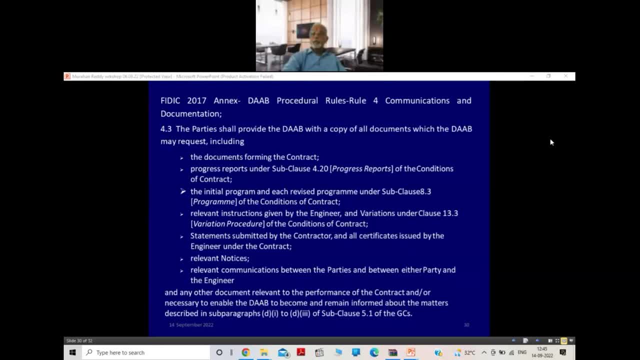 recommendation to the parties and I. there is no time limit is specified in the for the filing of written document before the vote by either party. this is this is what we are going to introduce. certain time limit is will be provided or submission of the documents, since, because once we have fixed the date for 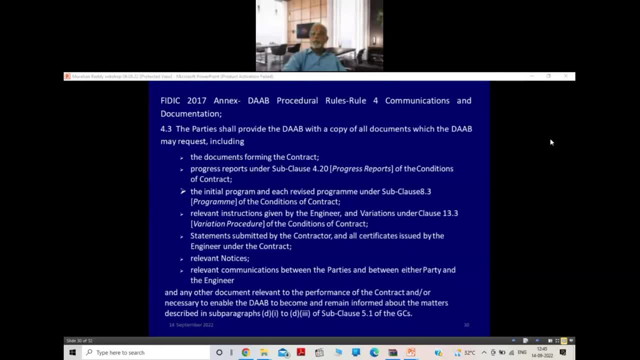 all days for showing recommendation by drb. that is 56 days. it should be. it should be. this is what we are going to introduce. certain time limit is will be provided, not be. uh, the process should not be delayed just for filing the documents of their pleadings by. 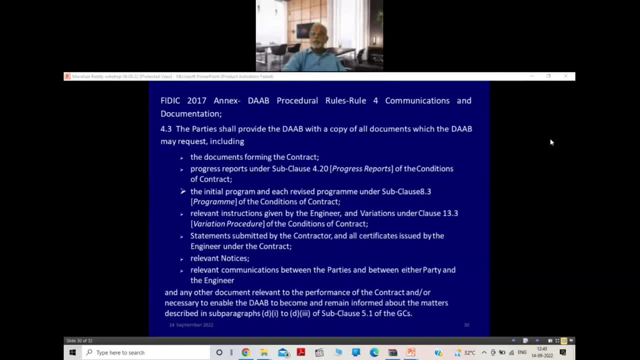 the parties. so we are, we are going to introduce the time limit for submission of the documents by the parties the earliest, uh. the time given for the vote to finalize decision is only three days. this is okay if dispute is on it. so he is of the opinion that, uh, the three days, or three sittings, 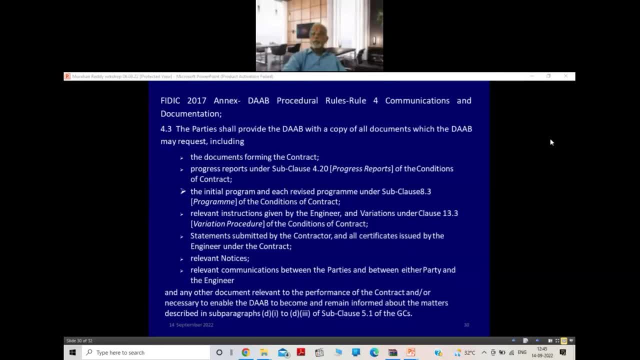 time for uh the drb to finalize their recommendation is short, it it should be increased, or? uh, there may be some provision that it can be increased to if, if the disputes are more in numbers or a single dispute is very lengthy or big, so with the mutual consent party can uh. so we are thinking of 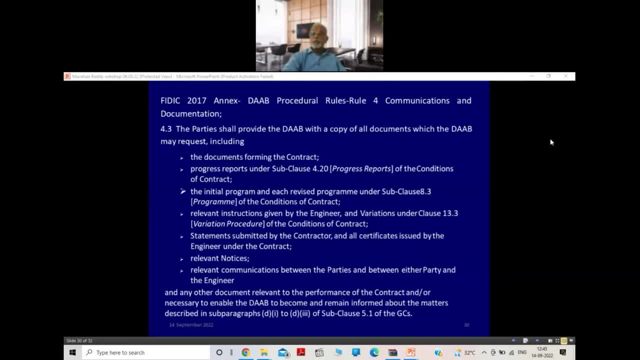 uh taking any action on this. we decided subsequently the board is advising the parties not to involve a yeah. so as far as the drb is concerned, this is very important that there should not be any uh advocate uh involvement because, basically, the issues are of technical nature and 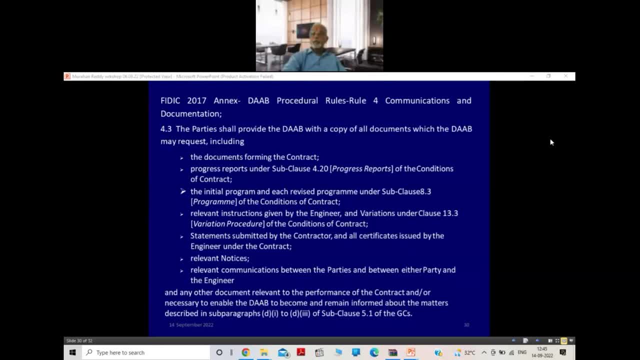 the technical person from uh all the three sides, lawyer and like the concessionaire or the engineer, all technical people are should be the presenter of their their sites for decision-making and the others should go out to the um. um board can issue detailed uh procedure to follow certain. 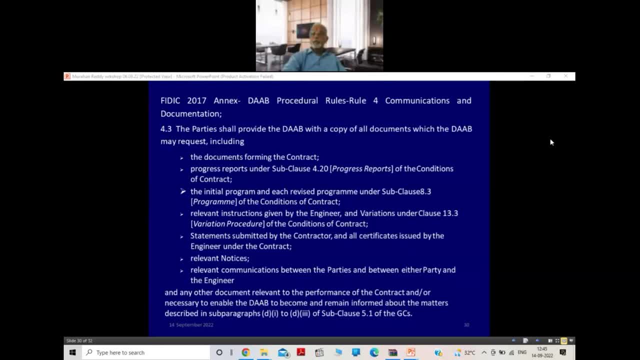 he has suggested something that the filing of written document by respondent- so the days- and the reason that by claimant- seven days. Despite agreeing to the above time frame, both parties are delaying. This is what the general observation by the DRV is: that even after fixing the time frame, 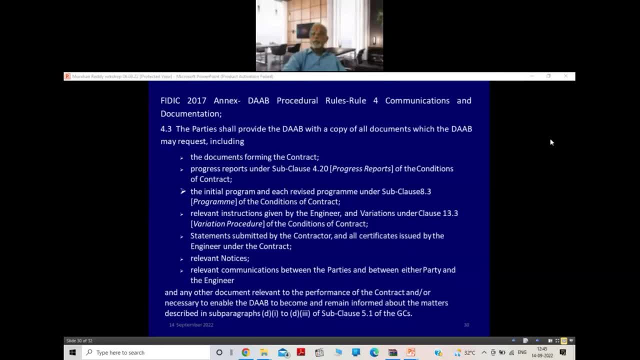 either of the parties are delaying the filing of the documents. We are doing something on that. We should have guidelines or SFP on this. Yes, now he has suggested about certain issues which are to be taken care of very seriously, like EOTs. 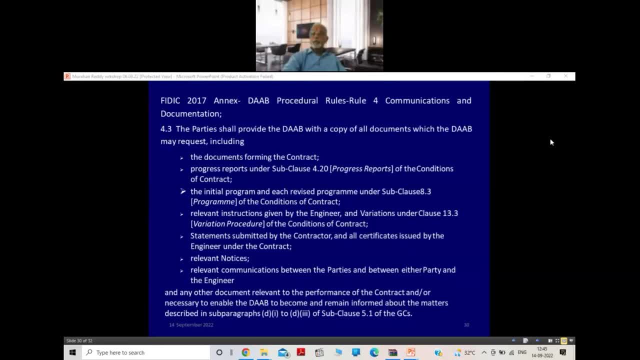 If EOTs are to be expedited, they should not be delayed for a long or longer period. COS are to be approved at the earliest. These EOT and COS are very important aspects. As far as the site position is concerned, I have already told you earlier that it was. 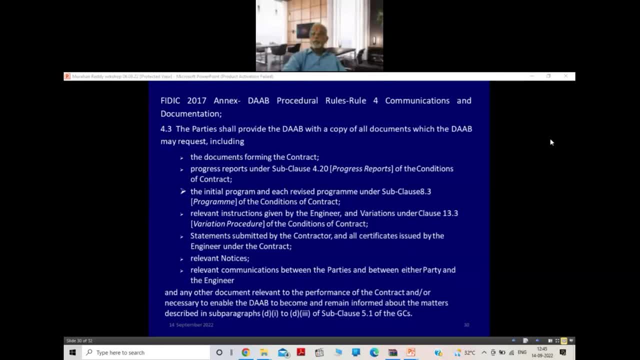 decided that until at least 90% of land is acquired, the agreement is not signed. This issue has now been almost resolved, but shifting of utility definitely is a concern. It should be taken seriously. IEAE performance to be monitored for effective functioning and monthly management meetings. 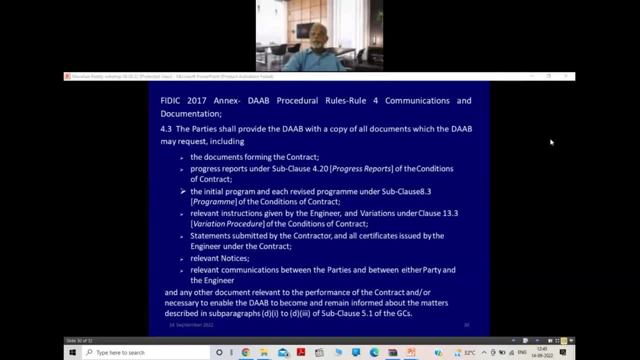 to be conducted. Both parties shall bring the potential issues which may crystallize, as discussed in the future, to be brought to the multis of DRV and CVA Advice to resolve. Both parties and IEAE to honor the advice of board members if they are deviating the. 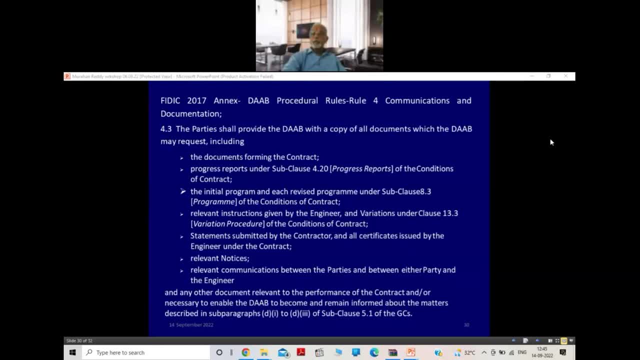 contract provision. The same is to be discussed and sorted out. The board members shall involve wholeheartedly, thoroughly, with both parties. Who has the right to follow court orders? IEAE board member shall be informed first. The board members should be informed in the following manner: as the board members. 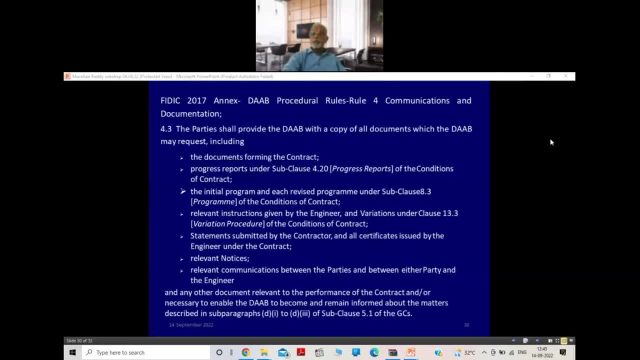 have agreed on the relevant issues in the past. Those who have not agreed to meet should be set to meet. The board members must be assured IEAE- нормative builing is a necessary part of the operation and should be agreed upon prior to the hearing of issues. 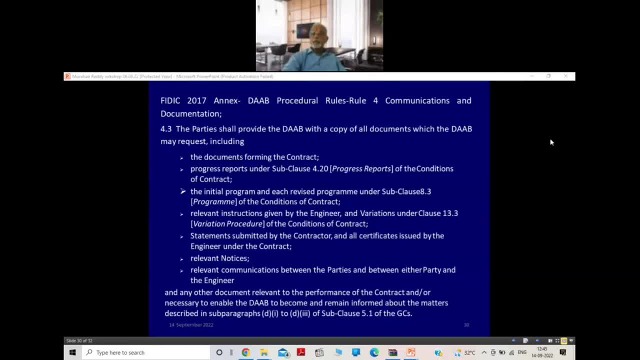 IEAE is an important part of the process. As a board member, you have to know the requirements of your daughter's rb, so this means uh dispute avoidance and resolution board. presently, the drb is just for resolving the dispute as and when it is uh referred to them or it is produced before that. 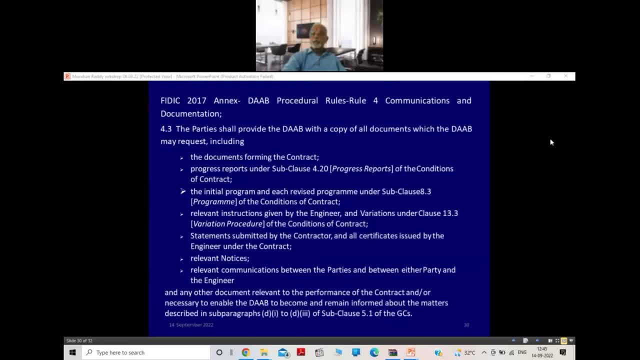 the new concept of uh provided in 2017 is dispute avoidance and the resolution, so the the board has been given additional, so up to do is, instead of resolving the dispute when it arises, they have been given authority to even go for suggesting how to avoid the dispute. 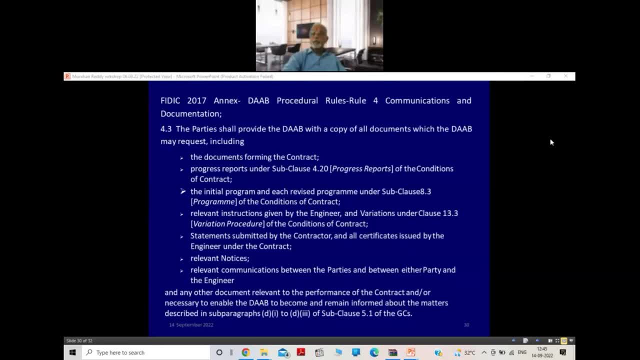 before it crops up. we are also thinking on this issue that uh that we will make certain uh changes in our rules and procedure and the uh we will issue uh this uh guideline of the press supreme. this uh avoidance and resolution, eating, prior practice and corrections after the law works. 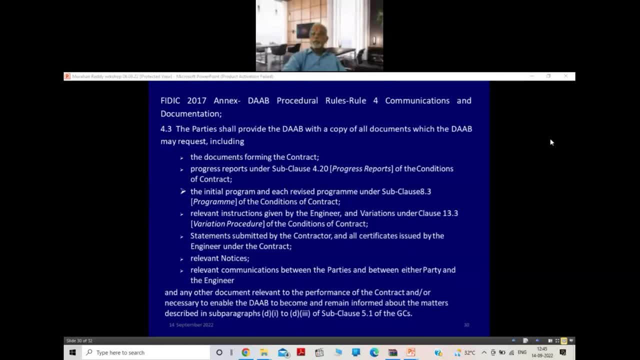 after the party organizes such and is a long the five to the of the or disagreement, it may invite the parties to make such a joint request. such joint request may be made at any time except during the period that the engineer is carrying out duties on the. 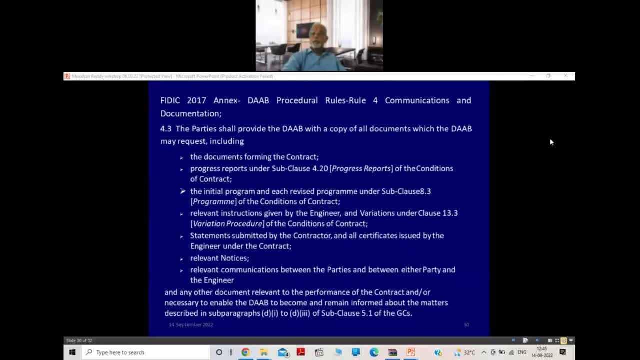 matter as an issue or in disagreement, unless the parties agree, other such informal assistance may take place during any meeting, site visit or otherwise. however, unless the parties agree, otherwise both parties shall be. you know I'm doing such information which shall be present at such discussion. the parties are not bound to act in such informal meetings and the EAAB. 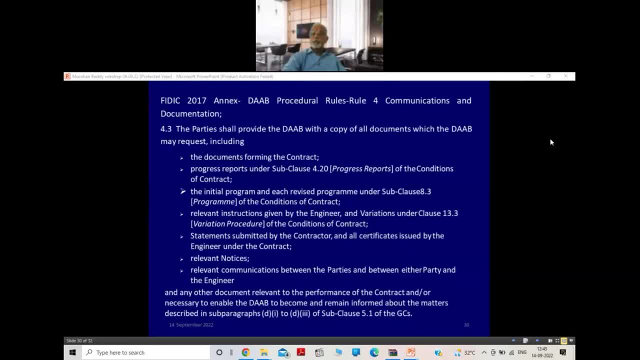 shall not be bound in any future dispute resolution process or decision by any views or advice given during the informal assistance process, whether provided or in writing. this is what the what is provided in FIDIC 2017. as far as the EAAB is concerned. what are the rule for, says the parties shall. 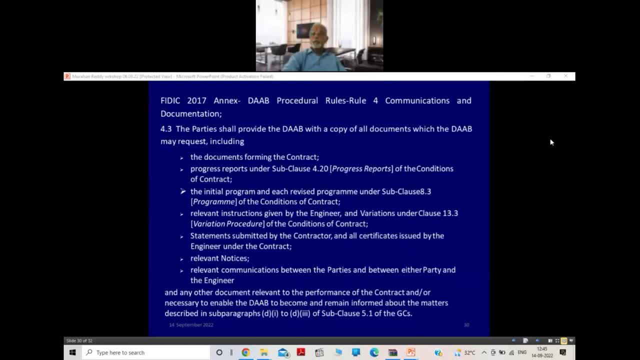 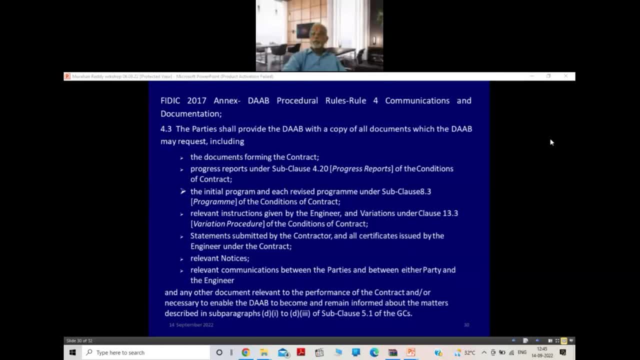 are very valuable and he has highlighted several issues which needs to be to be involved indicate which indicate the some short shortfall or shortcomings in the present process of the resolution to the EAAB. so I think I am done with all this. now I request the participants, if they want to speak out something, they want to pass a certain 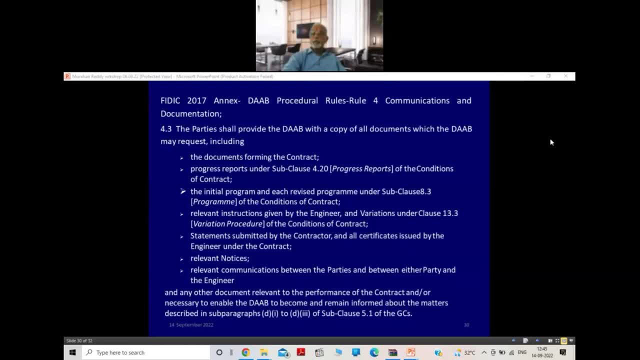 query or if they want to suggest any other things to the EAAB, Thank you. Thank you, Mike. Thank you, Neeraj ji. I think I have done. I have completed everything and I have requested other participants to ask if they have any query or question or if they have to give any suggestion. 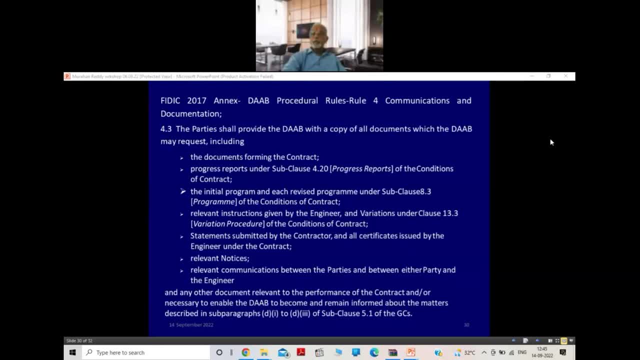 But I think nobody would like to. so can we finish it now? Yes sir, Yes sir, I think that there is no questions from the participant side, So now we can conclude this session. sir, Sir, thank you very much for sharing the presentation as well as sharing your knowledge with the participants.